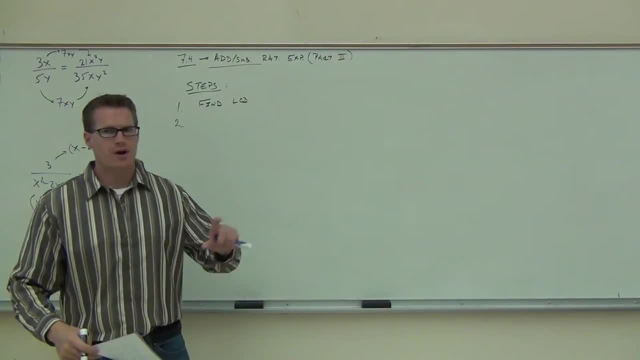 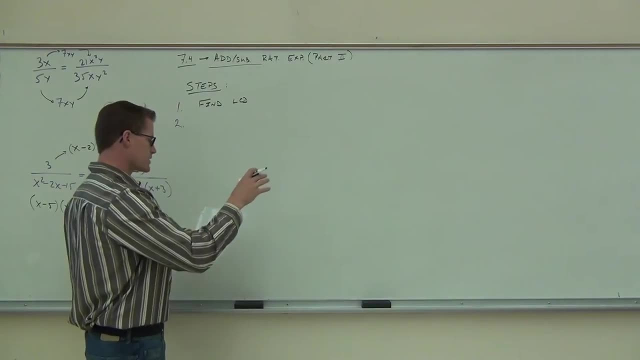 step is you're going to use that LCD to rewrite each fraction as an equivalent rational expression, what we just did. So that way you're going to have that common denominator. So find the LCD, then rewrite each rational expression as an equivalent rational expression. 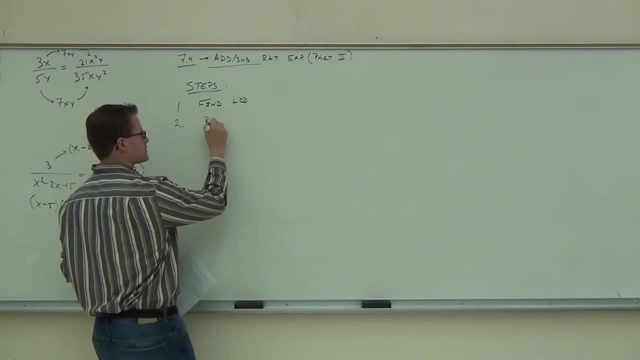 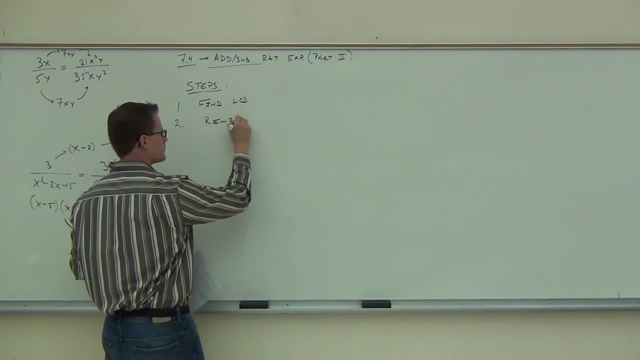 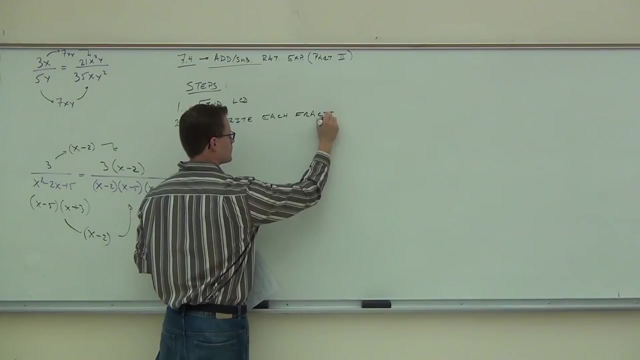 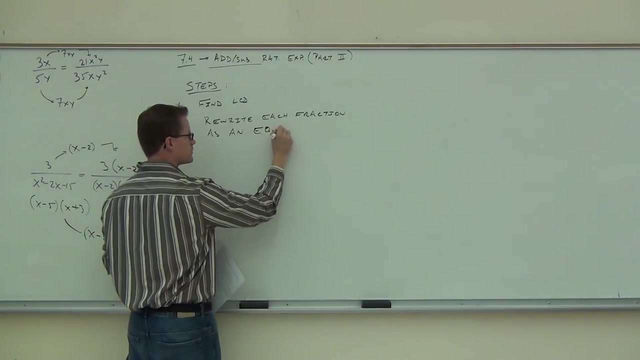 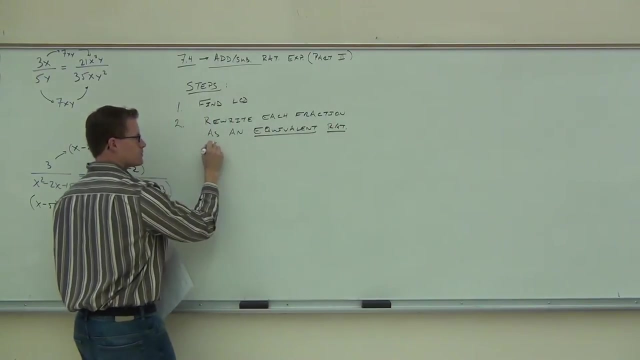 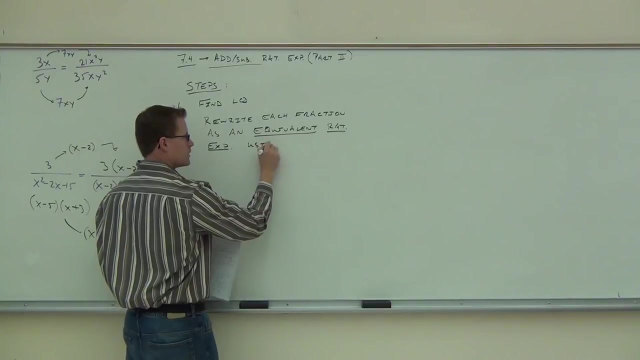 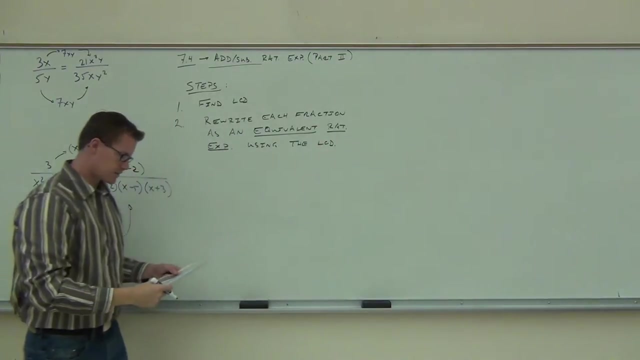 using the LCD, I'll make that a little bit more concise. Rewrite each fraction as an equivalent rational expression. That's what we did right here, and we're going to do that by using the LCD, and I'll show you how to do that in a second. 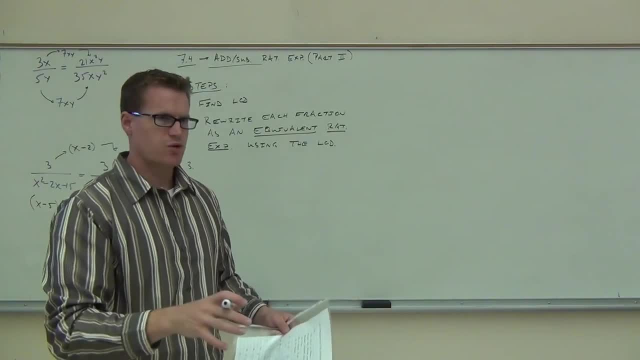 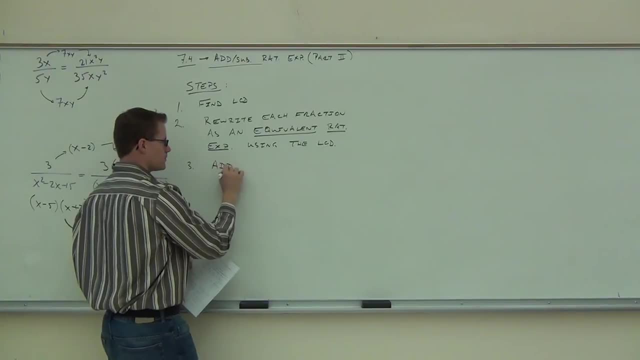 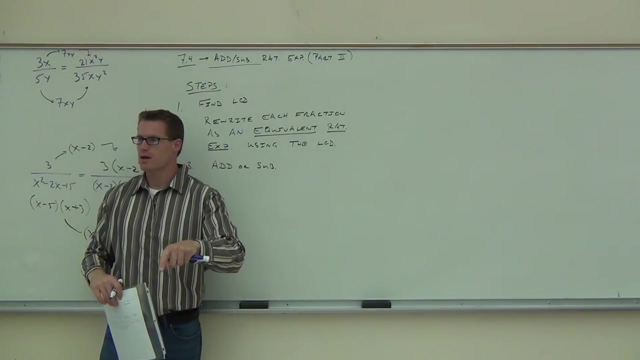 The next step we're going to do is we're going to add or subtract, because we'll be at that point We'll have a common denominator after step number two. So add or subtract. One thing I want to make a note on the paper here real quick: don't distribute your denominators. 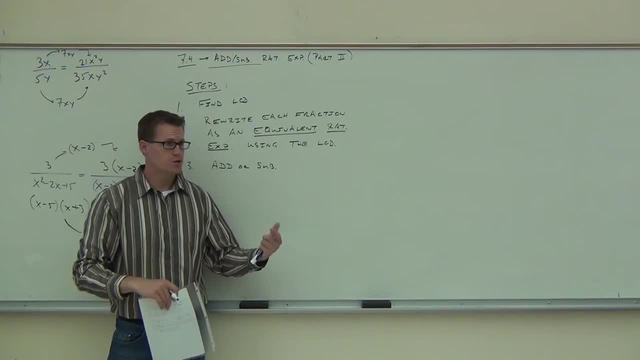 You never do that, At least in here. you don't do that because you're going to try to simplify later, right, Which means you're going to factor The numerators. yes, we will be distributing those because you need to combine like terms. 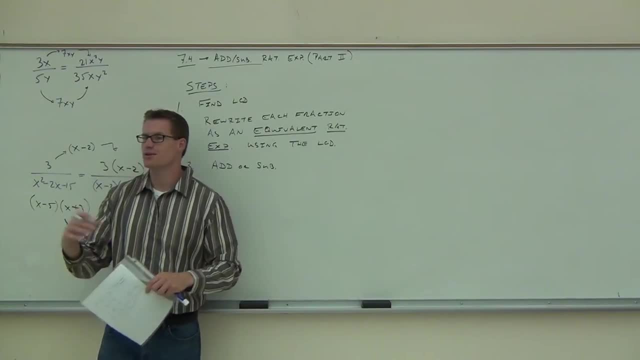 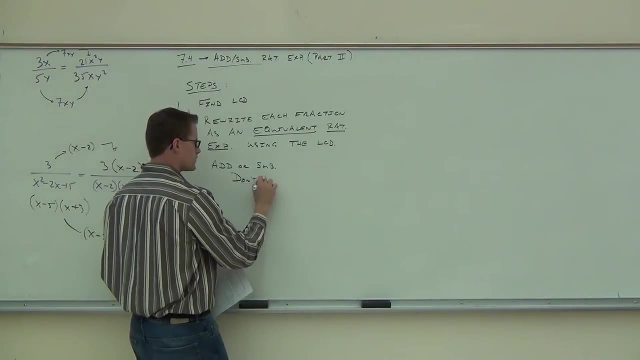 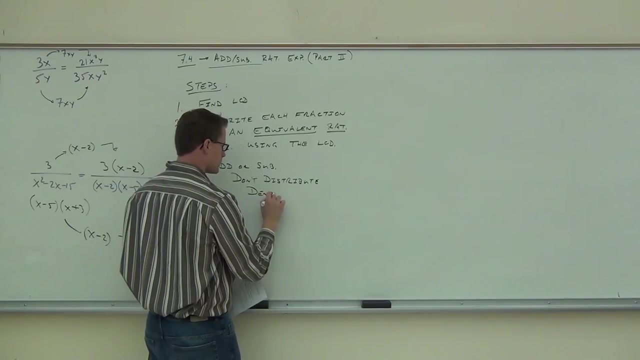 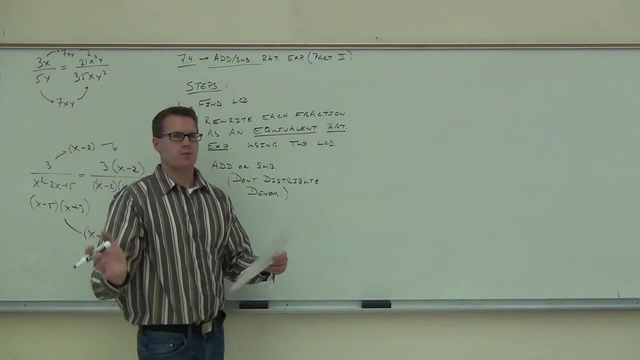 but on the denominators, you're not going to distribute denominators. You're going to wait until the very end and try to factor and simplify anyway. So don't distribute denominators. And the last step we're going to do. this is the step pretty much every time we have. 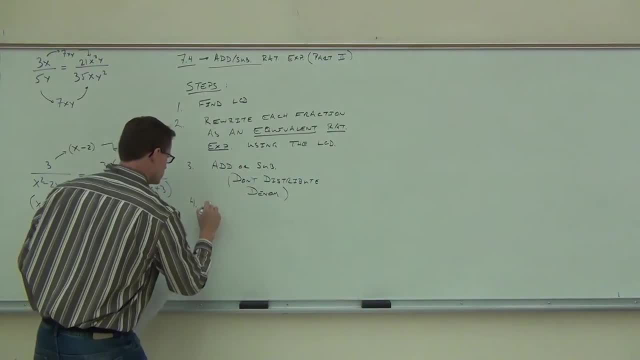 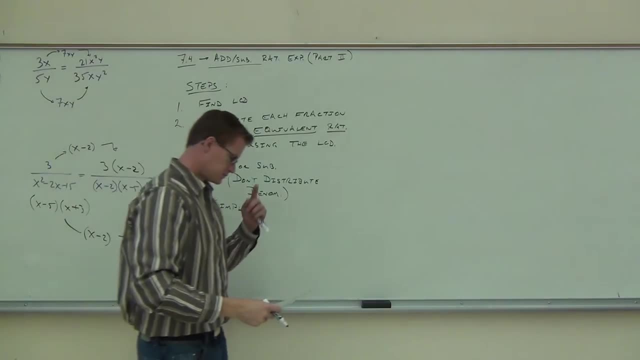 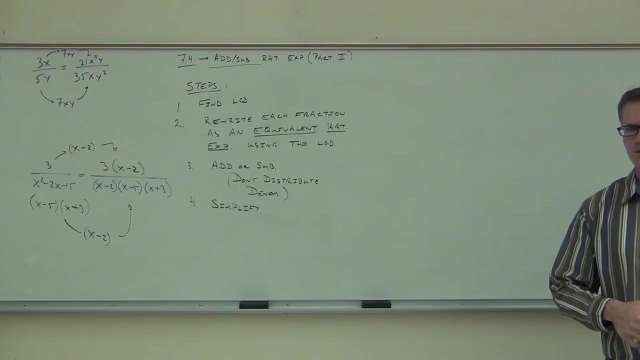 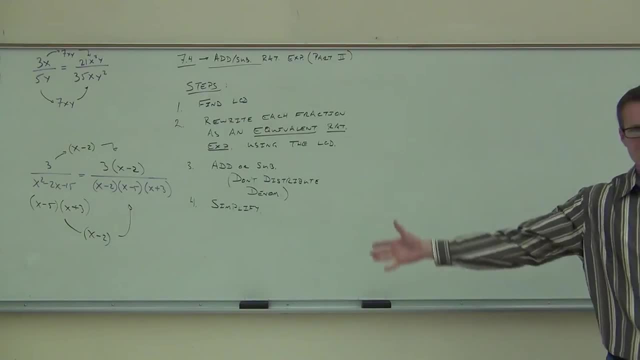 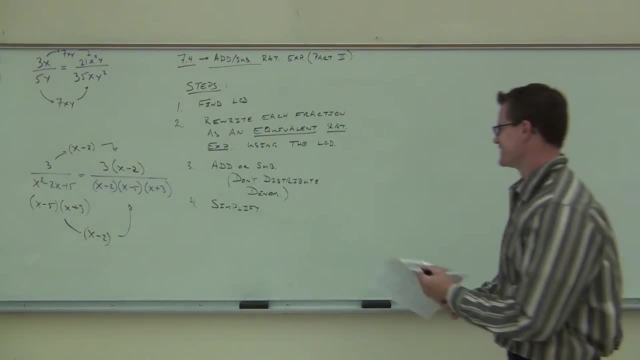 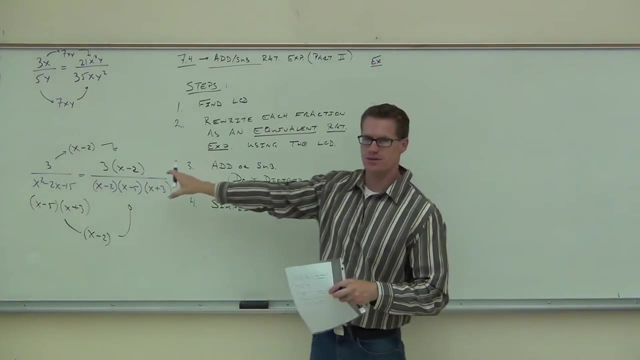 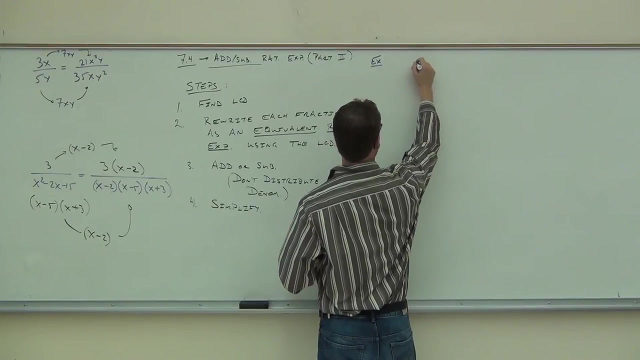 Together. Okay, We're going to start kind of slow. We're not going to do things that look like this yet. all right, We'll get there today, Okay. But to get the foundation laid here, let's start with something along these lines. 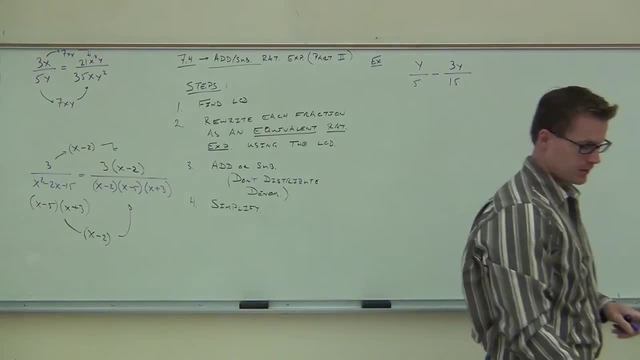 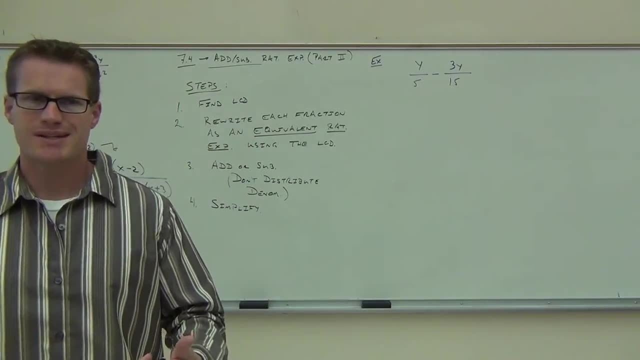 All right, All right. First thing, I want you to check to see if it has a common denominator first, because that can save you time, right? You don't want to waste your time doing all the stuff that already has a common denominator. 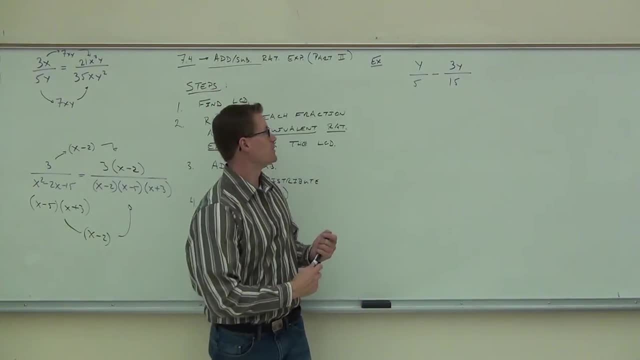 Do these have a common denominator? No, Common denominator, No, no, no, No, No, one's 5,, one's 15, so those are different. So that says you do the first step, which is find your LCD. 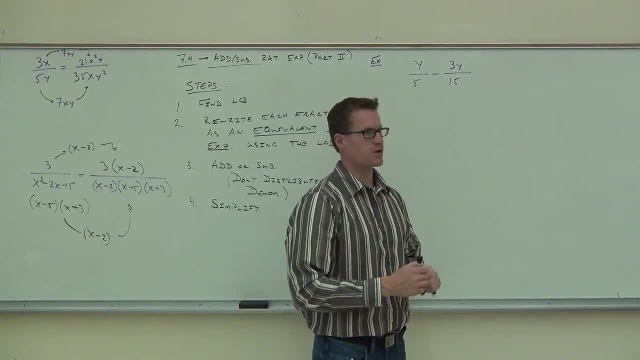 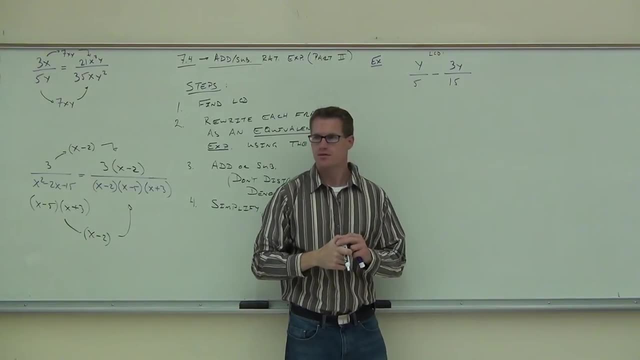 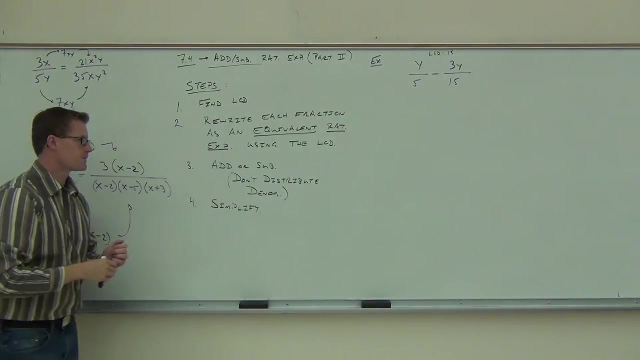 Take five seconds right now, find your LCD and write it down. okay, It should be very quick. LCD, in our case is Fifteen. Very good, Here's how we use that 15.. That 15 is very much like having this part right here. 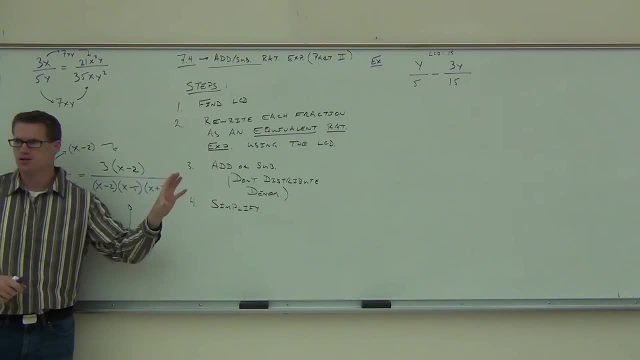 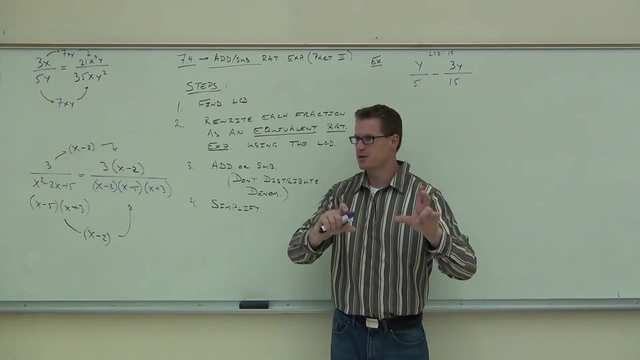 So the 15 is taking the place of the lower part of your second fraction on the equivalent rational expressions. Basically, what you're trying to do is make each denominator the same thing as 15.. Now, if it's already 15,, that's great. 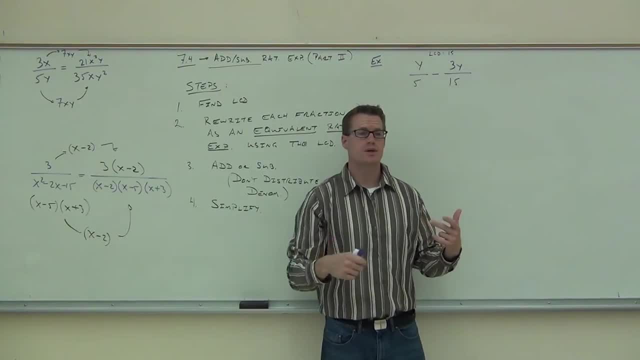 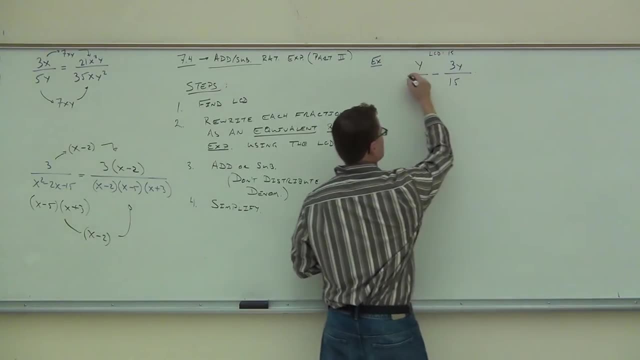 You don't have to do anything If it's not. you don't have to do anything If it's not 15, you ask yourself: what do I need to multiply by in order to get to 15?? So what we're going to show over here is multiplication on each side. 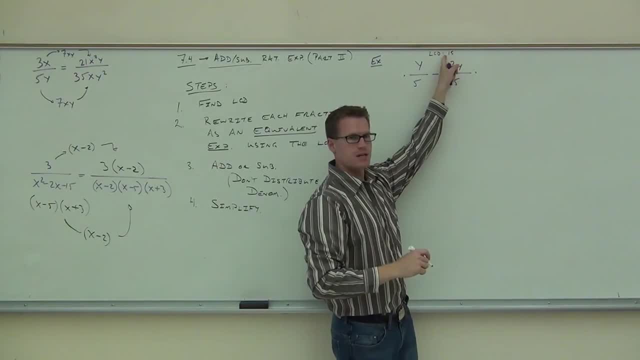 Now we're going to start on the right-hand side. I need an LCD of 15.. I already have 15.. Do I need to multiply this one by anything You're already set? Okay, that's great, That already has the 15.. 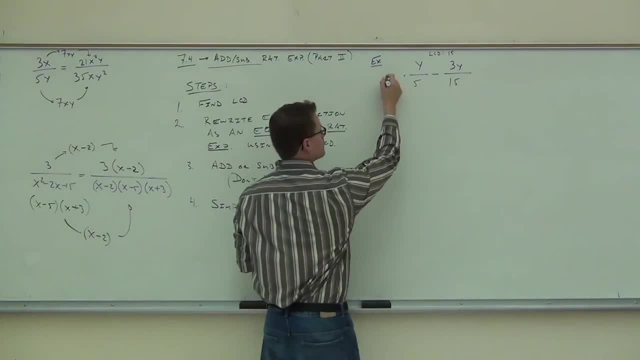 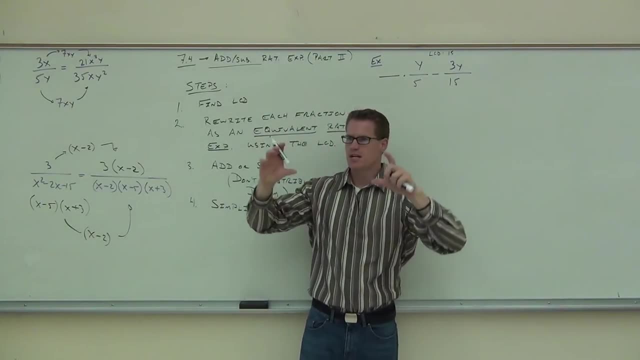 So I don't need to multiply there, On the left-hand side. the question is: what do you need to multiply by in order to get 15? What you want is 15 on the bottom of each, on the denominator of each of your fractions. 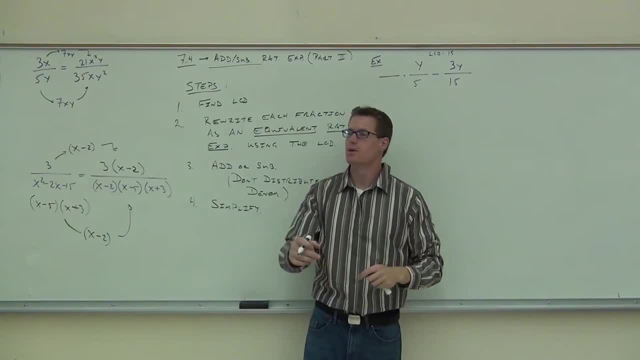 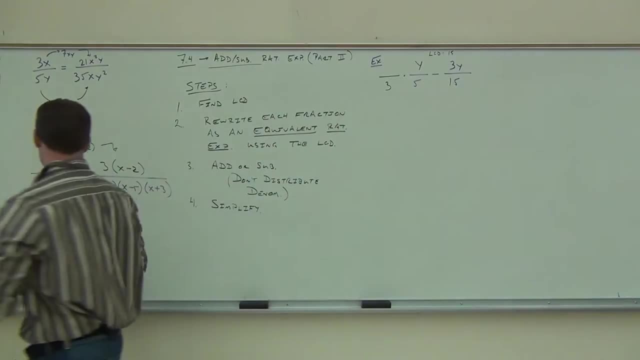 in this case, because that is your LCD, your lowest common denominator. What do you need to multiply by here? Three, Three, Okay, Now, just like over here, this is this part. look, Just like over here, what you're doing after you figure out what you need to multiply by. 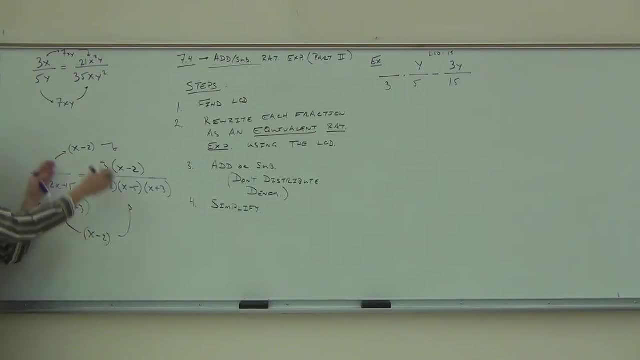 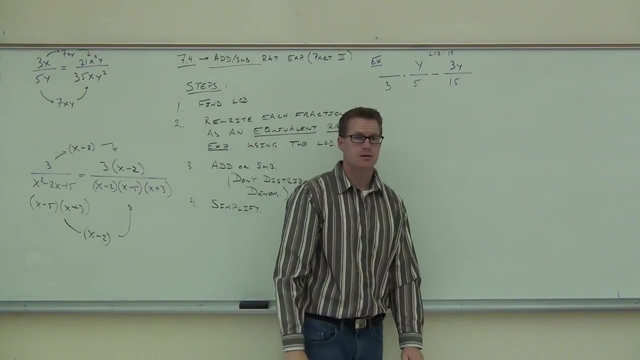 not only do you multiply the denominator, you also have to multiply the numerator. Are you clear on that part? Why is that the case? Keep it equal. Explain that, So they're the same. Keep it equal, so they're the same. 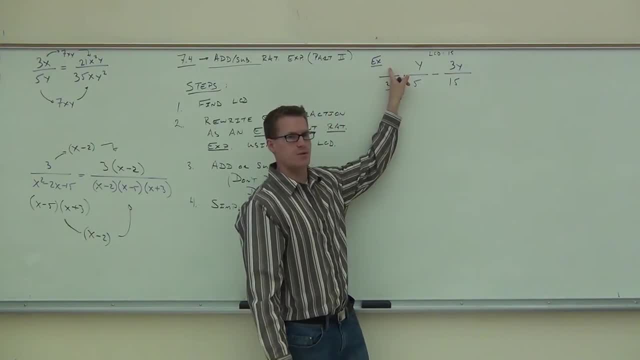 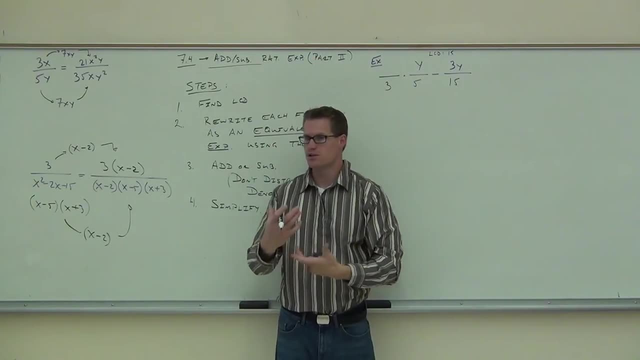 Okay, good, If I multiplied by three here and something different in three up there, would the fraction stay the same value? No, No. So basically I'm multiplying by one. Something over itself is one, And that doesn't change the value of anything. 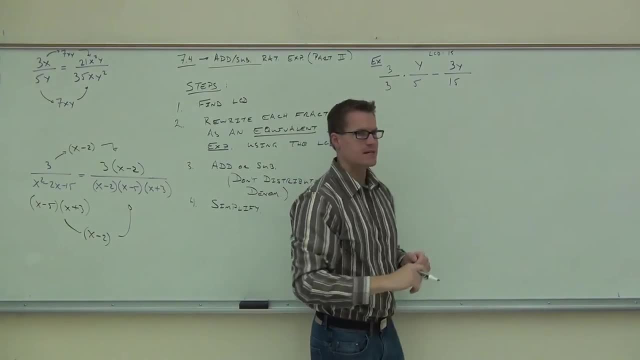 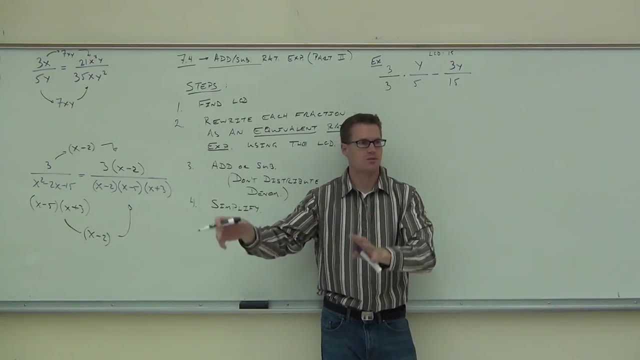 That's fine. That's what we want. Remember, our idea is that we are purposely unsimplifying fractions to make them the same denominator. That's what we're doing: Purposely unsimplifying. So here we multiply by three. 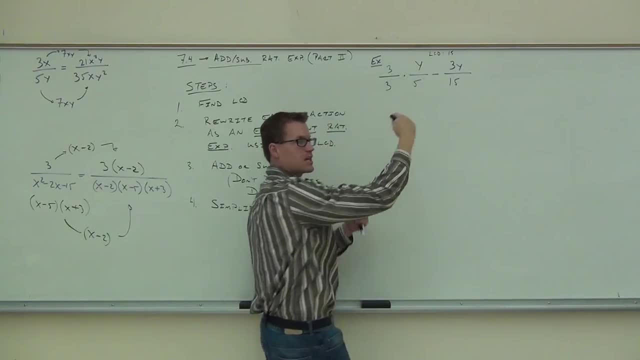 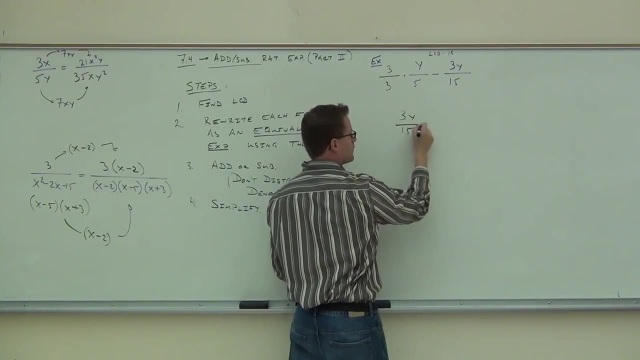 Because that's going to give us 15.. We have to multiply by three up there to keep our fraction the same value. Can you tell me what this fraction will become Minus? oh, we have three y over 15.. Very good. 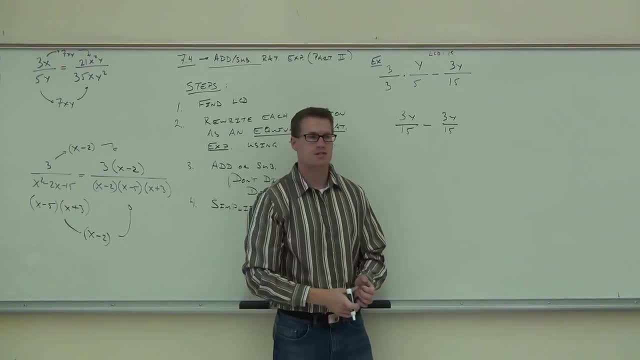 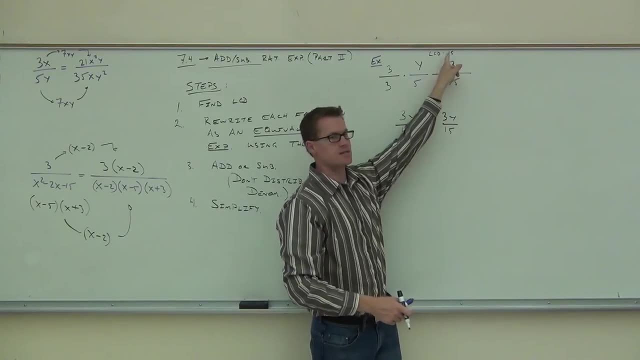 Did we do it right? You can check, because you should have the same number, three spots, Your LCD. you wrote down, So you should have the denominator there, And these two should be exactly the same as that one. If it is, you've done the right step. 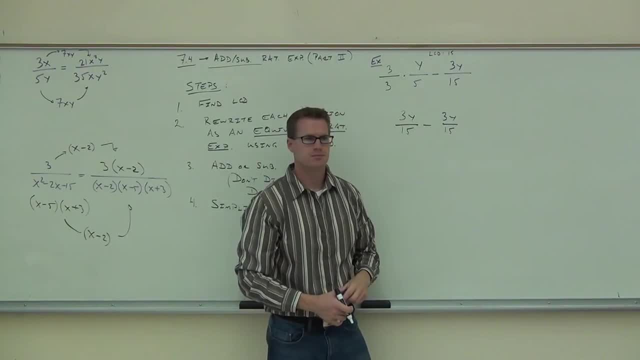 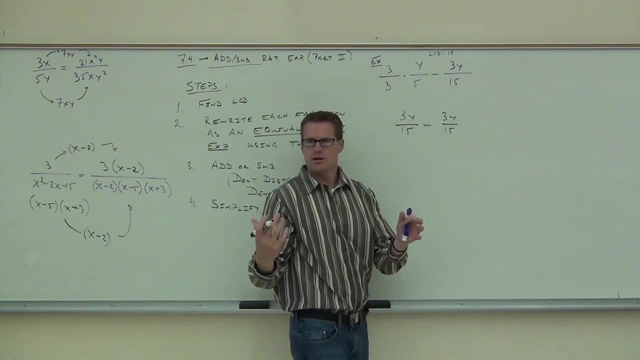 Okay, You've got that right. What's our next step? Subtract. Okay, so we're going to add or subtract, and we've already done that. This goes back to- let's see- last section or something, So that we we had this idea down already. 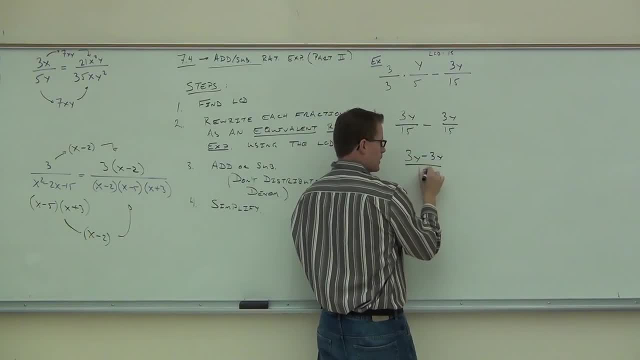 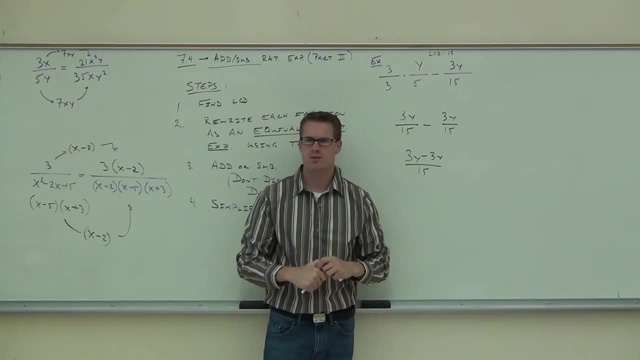 We just make one fraction out of this, Our denominator stays the same. We learned this already. And then we're going to do that subtraction just like combine, like terms. So three y minus three y gives us how much Zero, Zero. 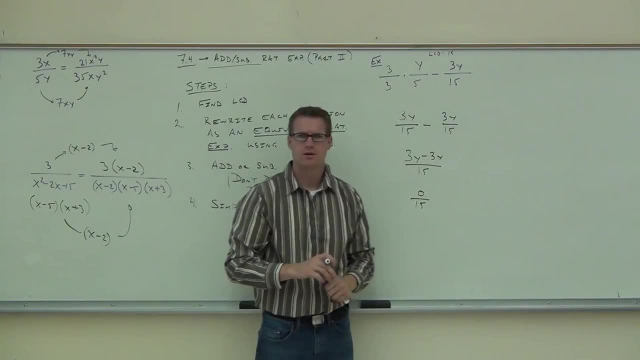 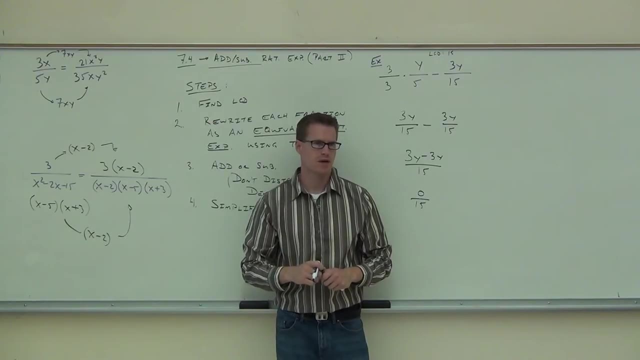 Is it okay to get zero on the top of our fraction? Yes, Is it okay to get zero on the bottom of our fraction? No, No One of them is okay. The top is okay. The top is okay. How much is zero over 15?? 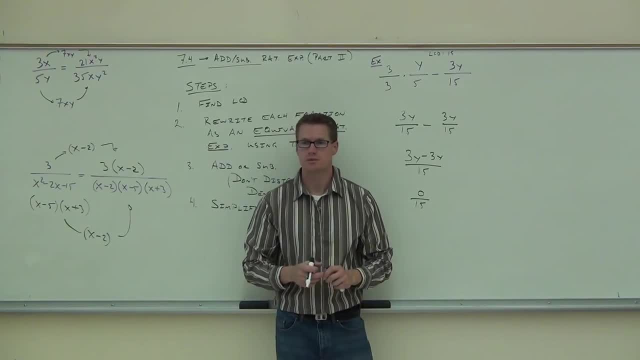 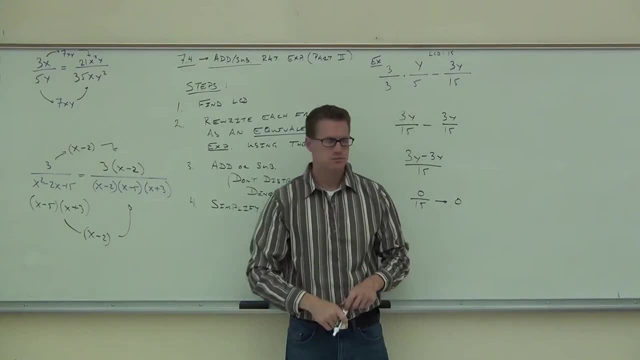 Zero, It's zero. Yeah, this one is zero, That's okay, So don't leave it at zero over 15.. The answer is zero. I wanted to show that one to you again, so that way it kind of sticks into your head a little bit. 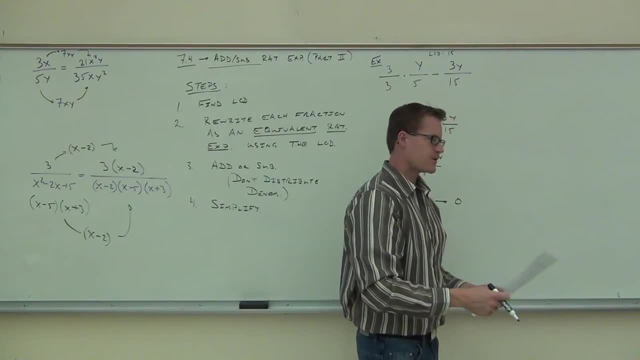 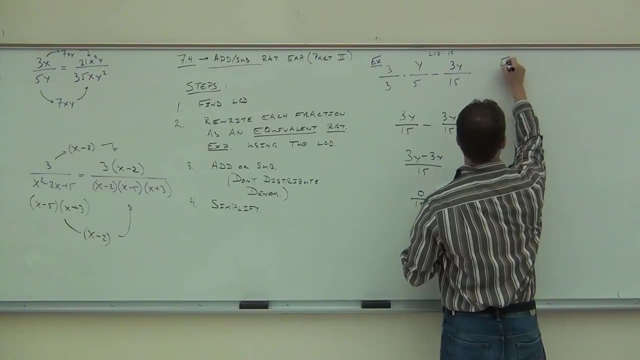 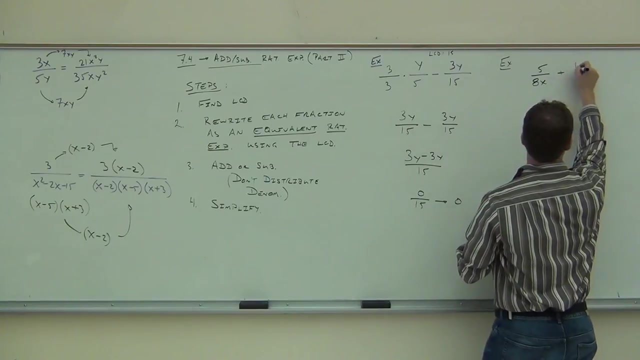 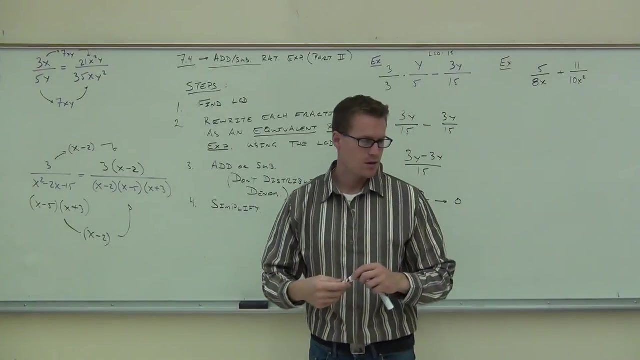 So some questions on that. last time, Are you ready to move on? Try something a little bit, A little bit different than just 15.. There we go. That's a good one for us to try. So, first thing we're going to do, we're going to do this one together. 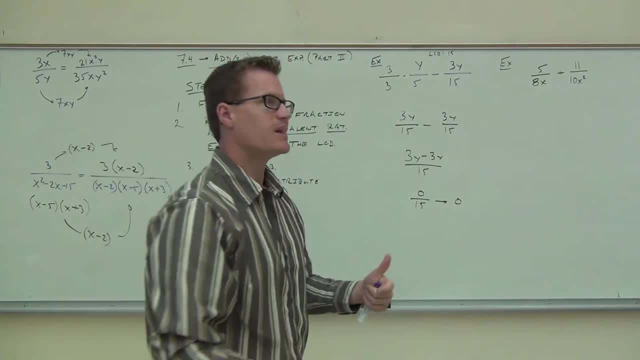 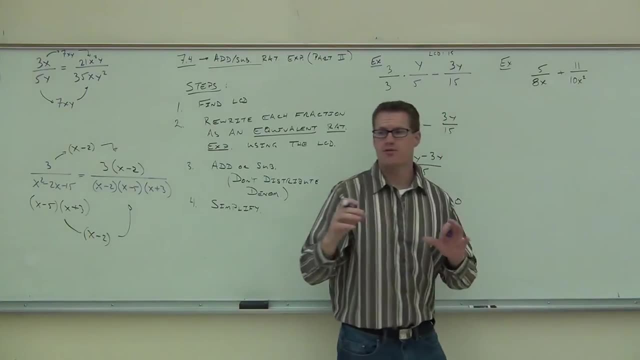 I'll model how to do it. First thing you do you check for common denominators. Now, of course, I don't have any in this case, so I'm going to try to find my LCD Now. we have spent a whole lot of time finding LCD. 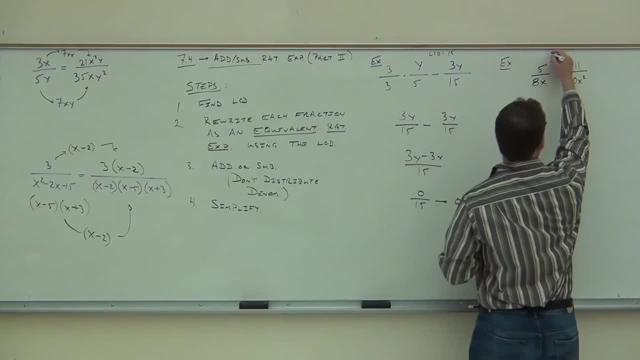 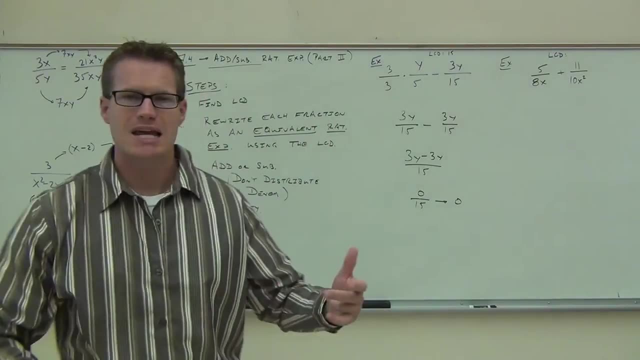 which is that's why we spent the time, so we'd be good at this stuff. LCD, the first thing you do. again, I'm going to look for my numbers. I'm going to look at 8 and 10 and find the LCD of just those numbers. 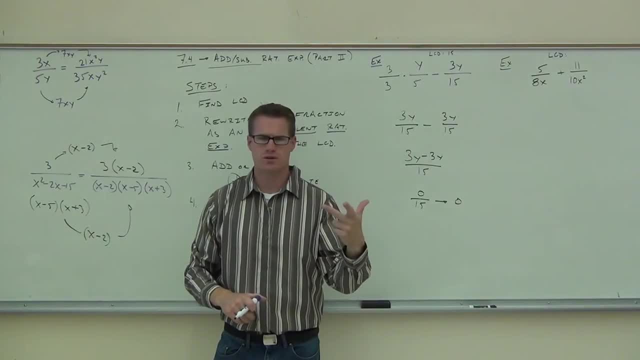 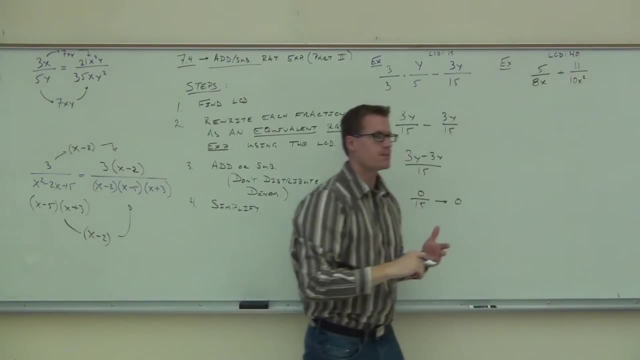 So I take my 10, it goes 8 going to 10, no 20,, no 30,, no 40, yeah, So 40 is going to be my coefficient of my LCD. The next thing that I look for is any variables. 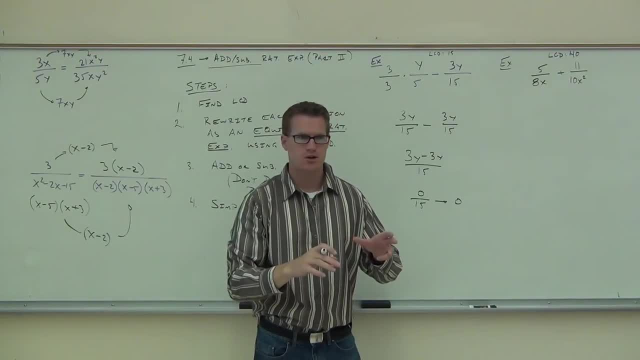 The different factors. Remember working with different factors. You probably did it on your homework. if you started your homework, You probably were able to get this far and go. oh yeah, I know how to do this. We look at our different factors. 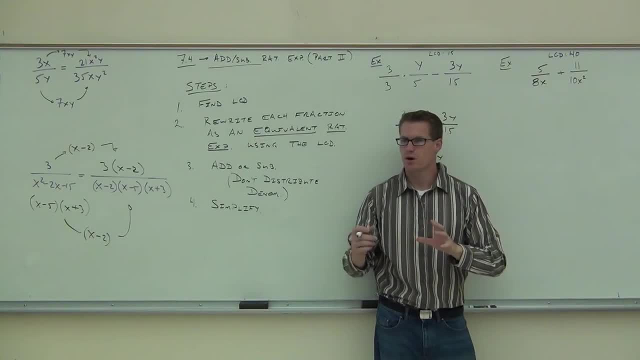 In this case, the only factor we have is X, So we're going to take the largest power of X that we see. There's X here and X squared there. Which one am I going to write up there? X squared, Not X cubed. 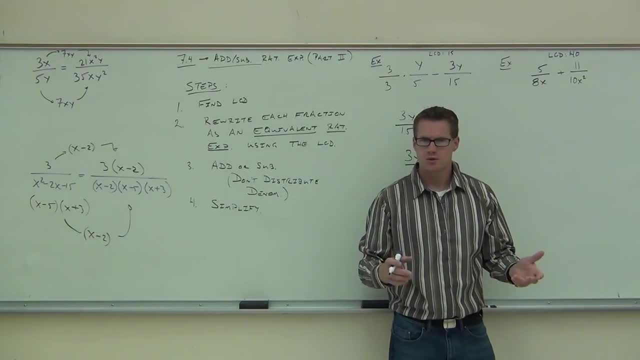 That's too big, We don't want to deal with that. Look, if you wrote X cubed, you're going to have to do work on this fraction that you wouldn't otherwise have to do. That's going to make things a whole lot bigger. 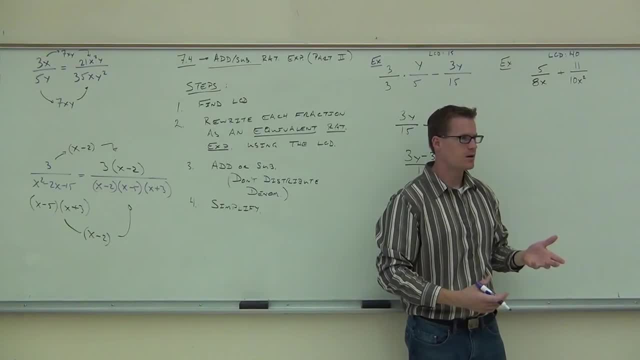 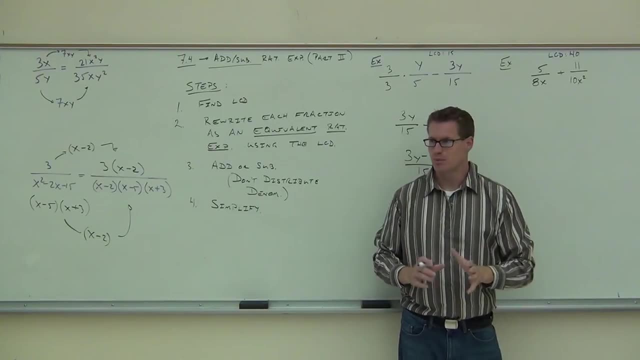 and make your simplification a whole lot easier, A whole lot worse. Are you with me on that? Make sure You don't want to make your fraction bigger, do you Not? if you don't have to, No, We're going to make things as simple as possible. 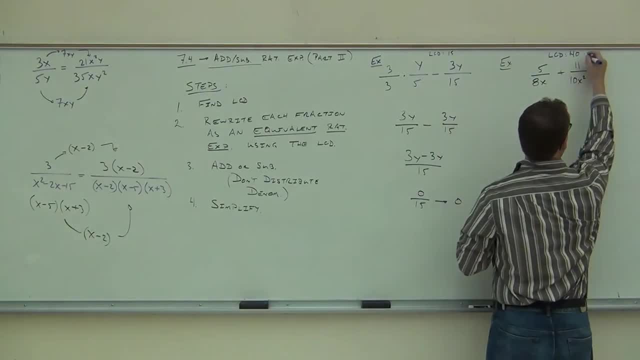 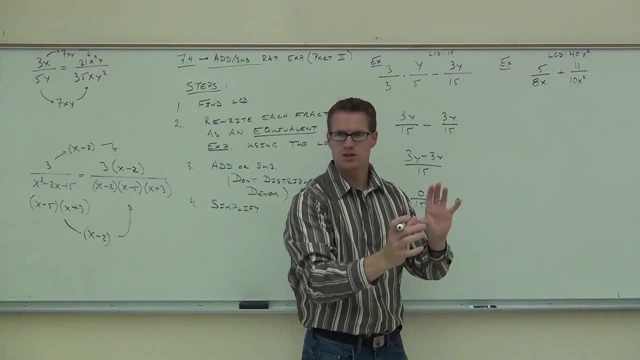 Not as worse as possible. That would suck. So the 10 to the 8 gives us 40 as an LCD, The X and X squared, we take the largest power of each different factor that we see. There's only one different factor. 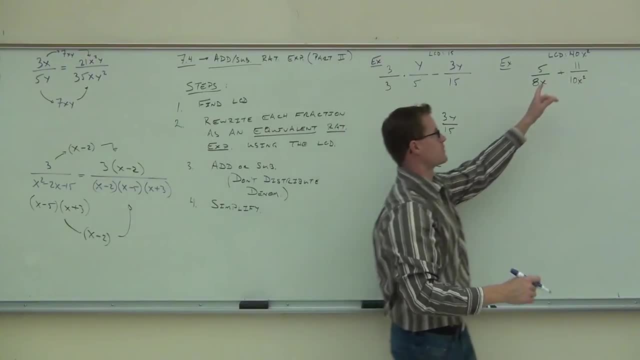 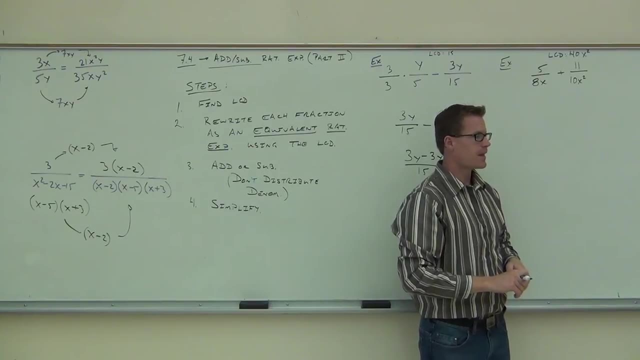 There's only X, So we take the largest power of X and that right there is our LCD. Are you good with that? Yeah, That's what we got. That's what we covered last time. So the question now is: how do I get from these denominators to my LCD? 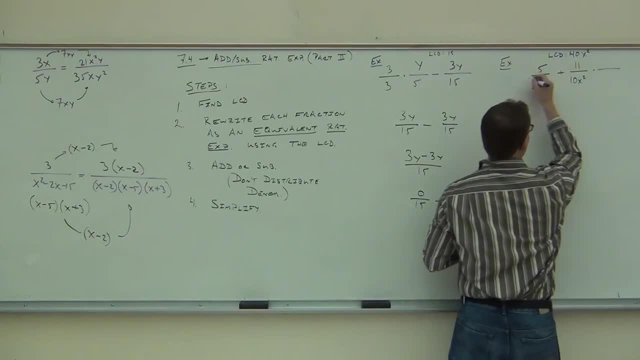 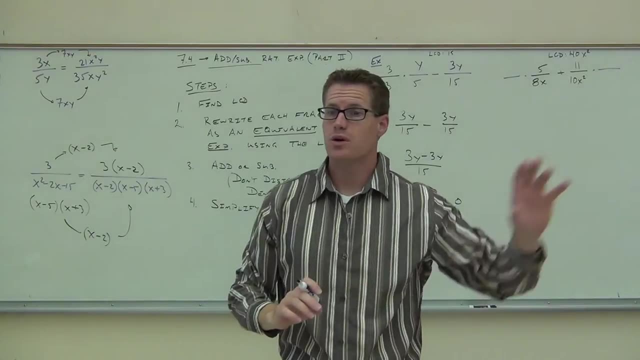 And that's where the multiplication takes place. So, on each fraction we're going to have to multiply by something. Let's work on the right fraction first. Let's look up there. I need to get from 10X squared to 40X squared. 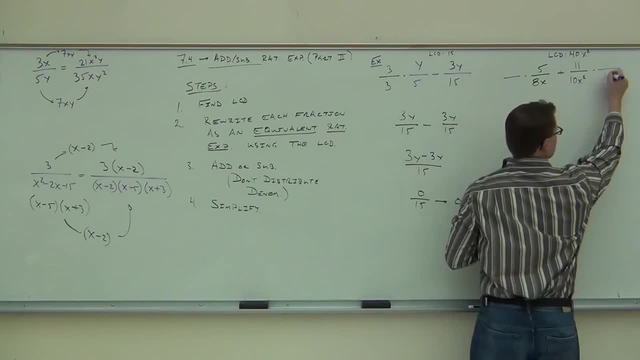 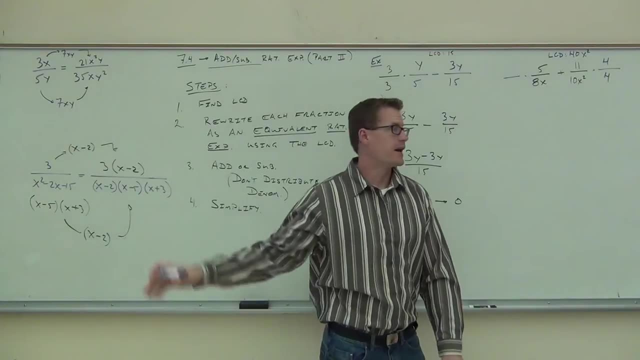 What do I need to multiply by, ladies and gentlemen. So that's here And that's there. 4 over 4, because that makes a fancy. 1. On the left-hand side I have 8X. I need 40X squared. 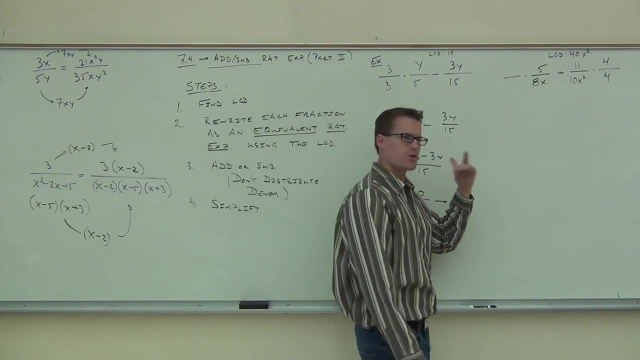 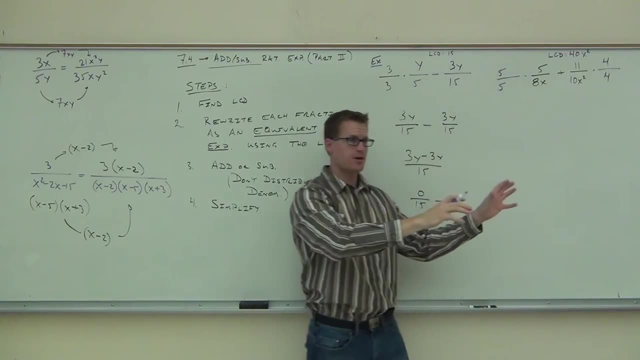 So to get from 8X to 40X squared, I'm going to ask first the number: what number do I need to multiply by 5.. 5, because that takes you from the 8 to the 40. That's, I need to multiply by 5.. 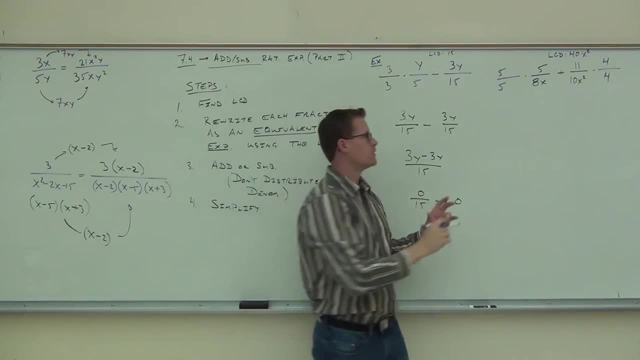 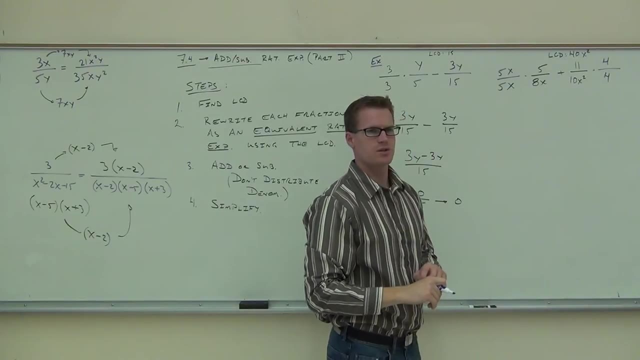 How am I going to get from X to X squared though, X times X squared? Let's see if this works. So let's do the math in our head, okay. What's 10X squared times 4? 40.. 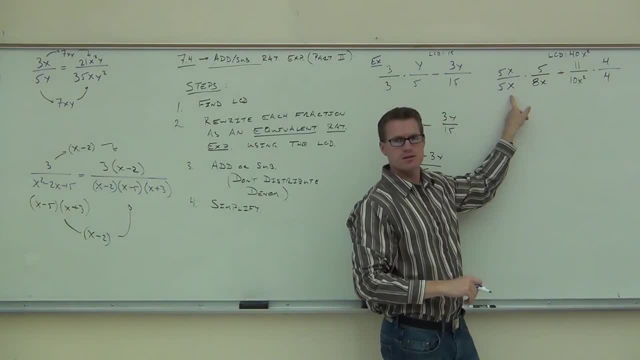 40 times 4.. What's 8X times 5X 40.. 40 times 4.. That's what we want, right? That's where those numbers are coming from. You're asking yourself: how do I complete this problem? 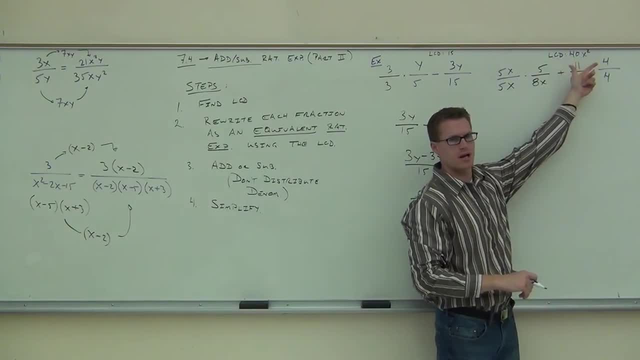 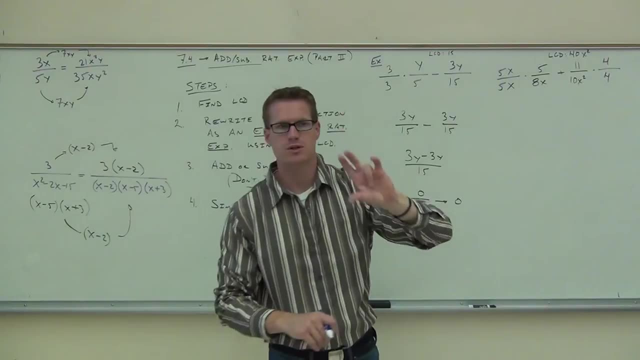 How do I make this into this by multiplication? That's what you're asking. How do I change this denominator into my LCD by multiplying things? And we do that to both the top numerator and bottom denominator. I'll try to help you. You're okay with this so far. 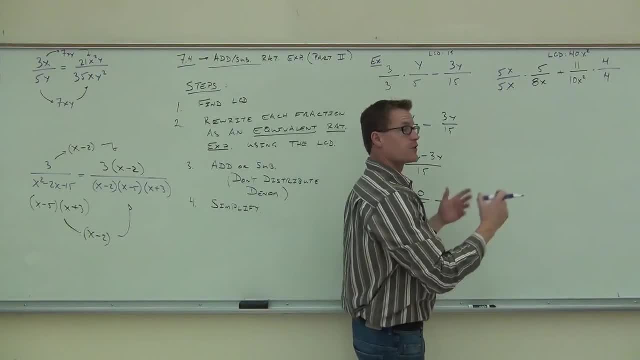 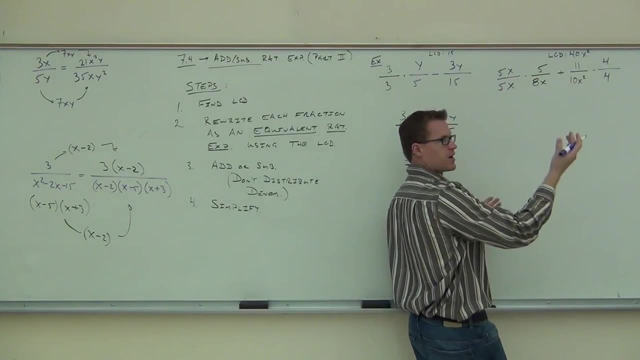 Yeah, Okay, Let's figure out what this fraction is going to be now, Because, remember, we're purposely unsimplifying. So I'm taking the 5X times the 5.. We've multiplied fractions before. That's great. I certainly don't want to start simplifying things, do I? 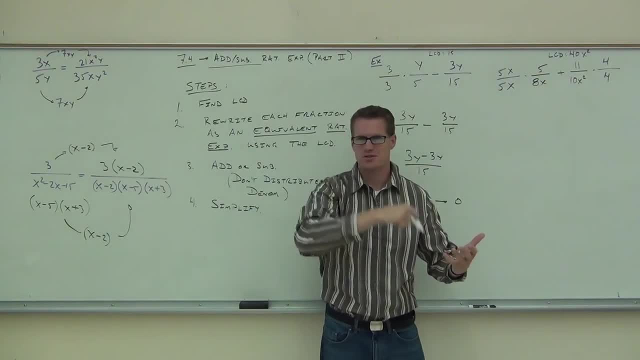 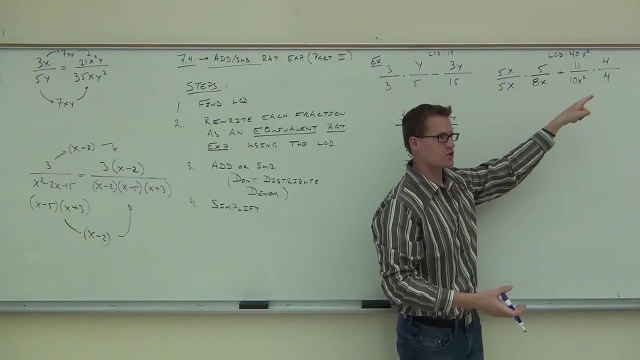 Because I'm purposely unsimplifying. I don't want to do that. I don't want to start crossing stuff out, So don't waste your time, because that would be a complete waste of time, right? If you did this work and you did this and you crossed everything out because you're going. 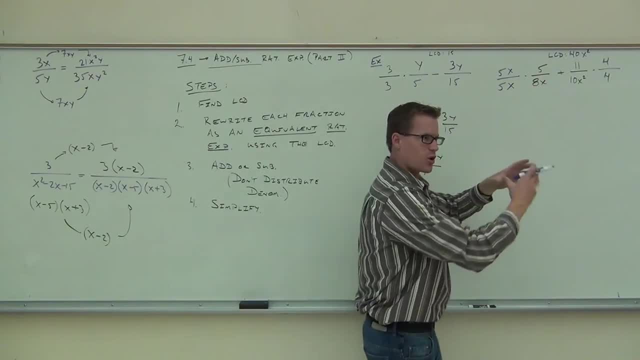 to get this right back again. So we don't want to do that. So we're purposely simplifying, We're simplifying, We're simplifying. We're purposely making these bigger temporarily so we can add them together. This is going to give me 25X. 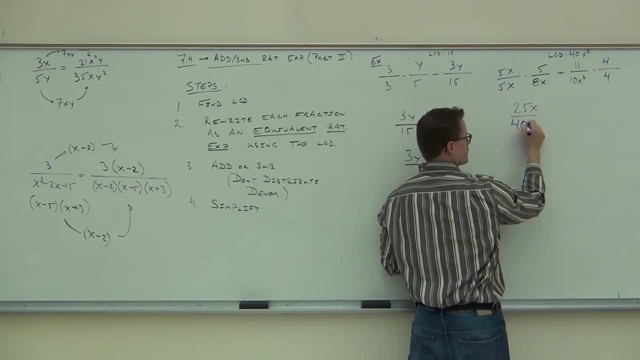 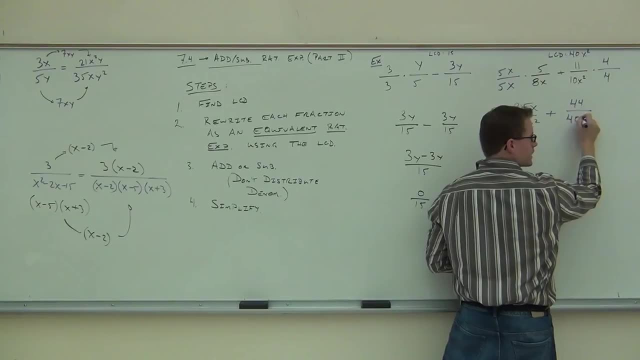 On the denominator, I get a 40 and I get X squared. That's what I wanted. I have the plus sign. still On the second fraction, I get 44 over 40X squared And we're going to see that I did the problem right. 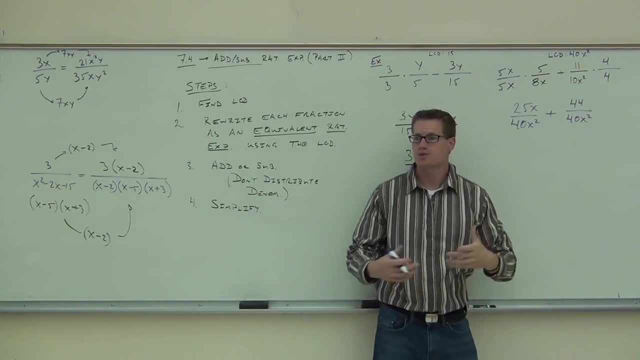 We have the LCD up here. We have it in both spots down on our fractions. So now we're able to add these things together because we have a common denominator. The next step would be: okay, It says we can't. We have the common denominator. 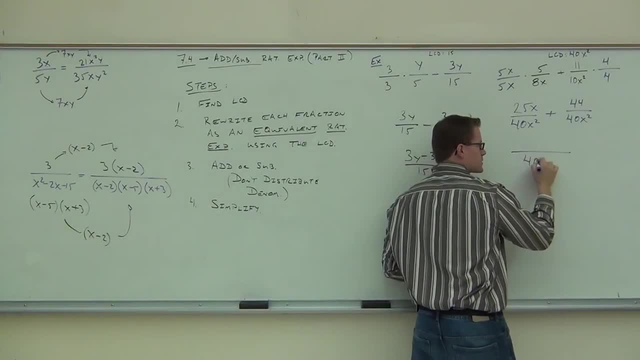 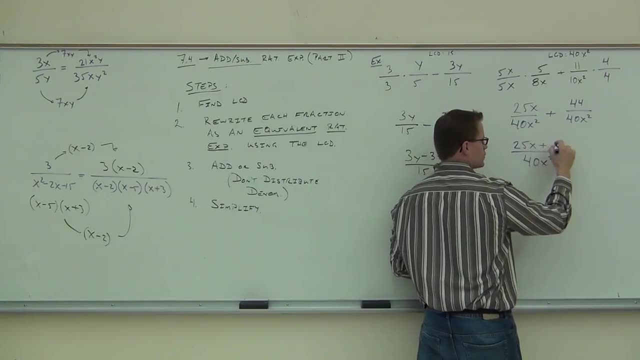 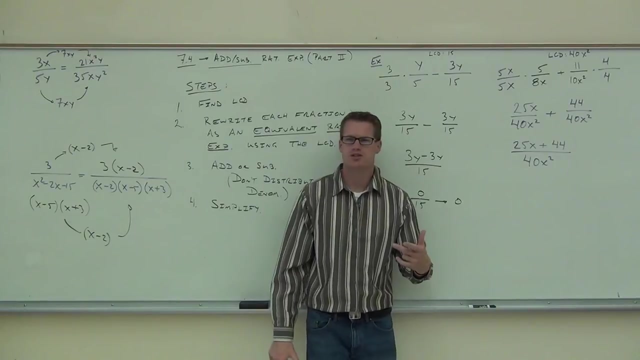 We're going to make one fraction out of it, write that LCD again, put our two fractions numerators on the second numerator, here on our new numerator. And the last thing we try to do is to simplify. Simplify means you're going to try to factor and cross stuff out. 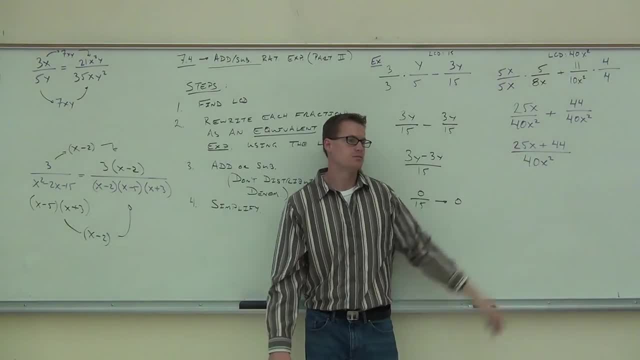 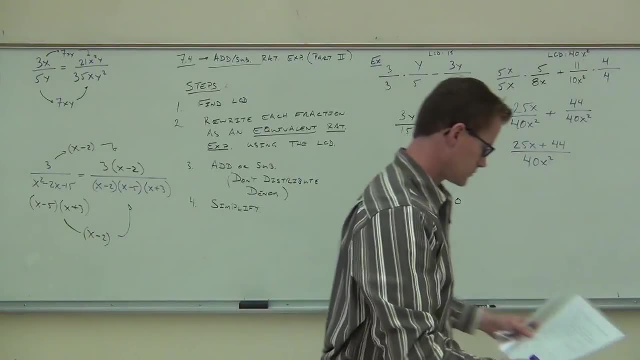 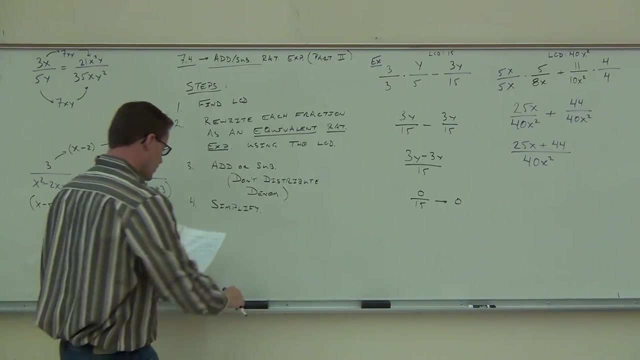 That's the fun part. Can I factor that? No, Then I'm done As far as you need to go. Raise your hand if you have a question, If you're okay with this problem. Before we go any further, I'm going to give you about a minute to try one of these on your own, okay? 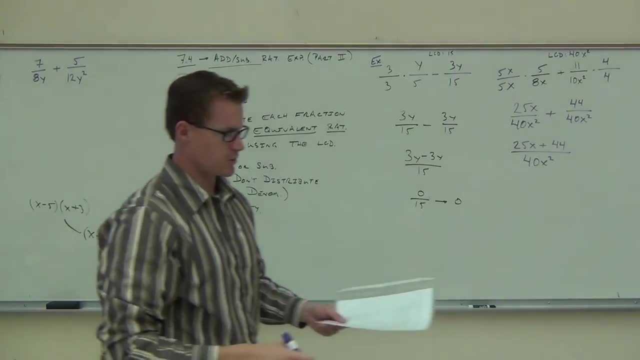 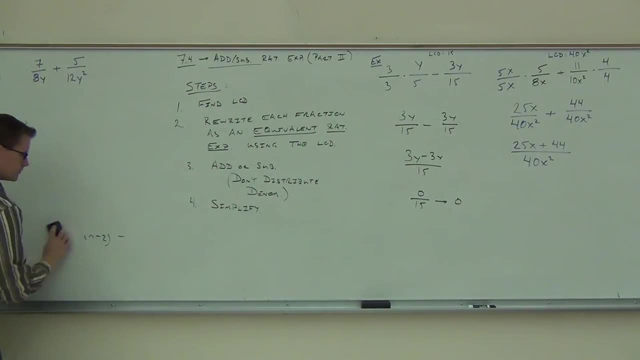 All right. So we made use of about an ounce and a half of that and that amount is going to be B 1 times the EPA, per second out of A. Now it's a little bit of an area here, a little bit over here. 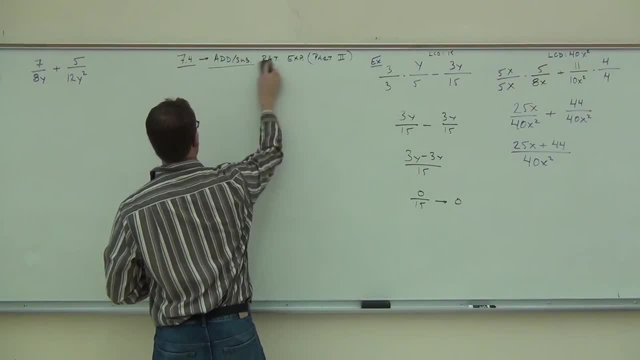 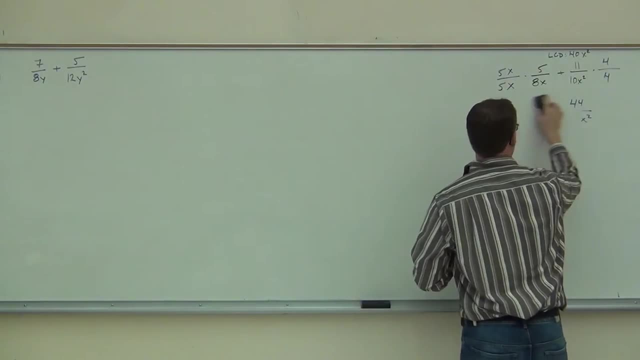 So lets give it a bit more tension, Let's give it a little sense. Once you know that, and then, as soon as you figure out what is going to work for your fries in this pool, We'll see how it goes down, down, down, down, down down. 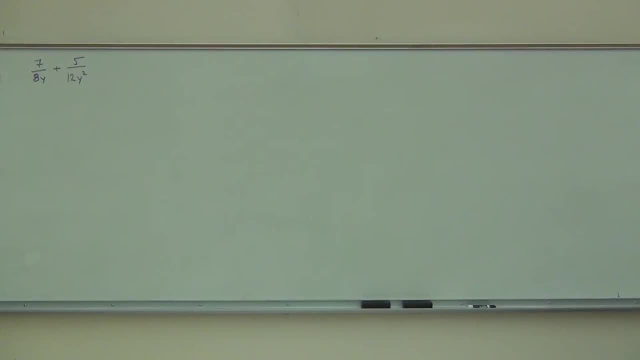 Thank you. Okay, so the first thing we do is find an LCD, because we need that. What is our LCD here? Let's see What's the number, part 24.. Great, 24.. That's fantastic. And the variable part: 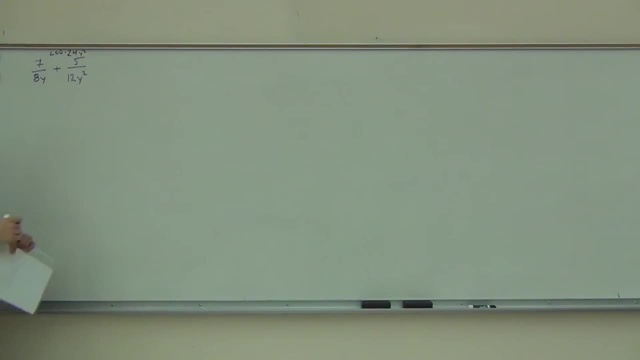 Y squared. Hopefully you got 24y squared. Did you get 24y squared, Sweet? That means we need to multiply each of these fractions, because right now we don't see 24y squared anyway, So we're going to have to make each of these denominators into 24y squared. 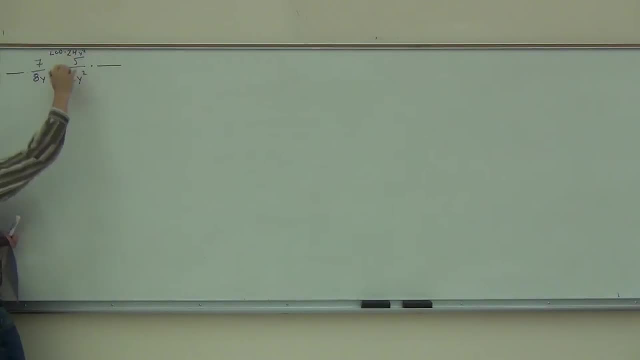 Over here. I'm noticing: in order to get from 12y squared to 24y squared, I need to multiply by a 2.. Did you multiply by 2?? Okay, Okay. On the left-hand side, I have an 8y. 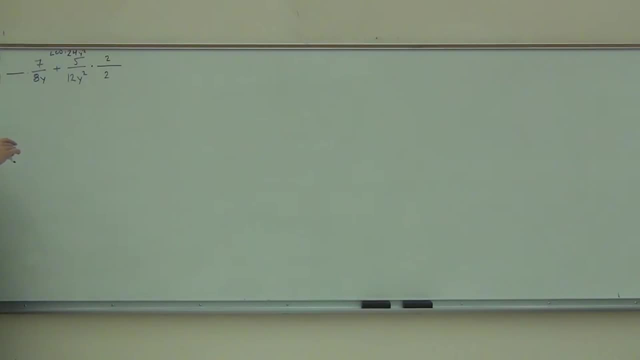 I need to get to 24y squared. So the number I need to multiply by to get from 8 to 24 is what 3.. That's going to be there, The variable to get from 8y to Y. 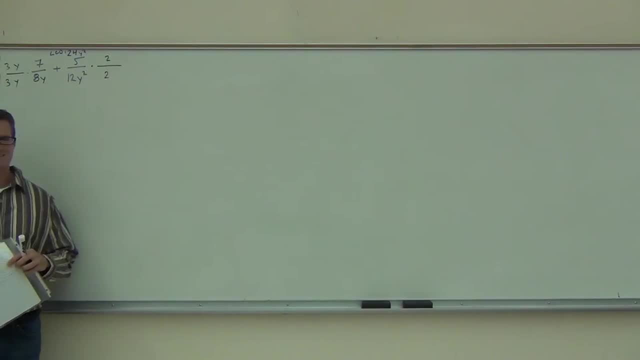 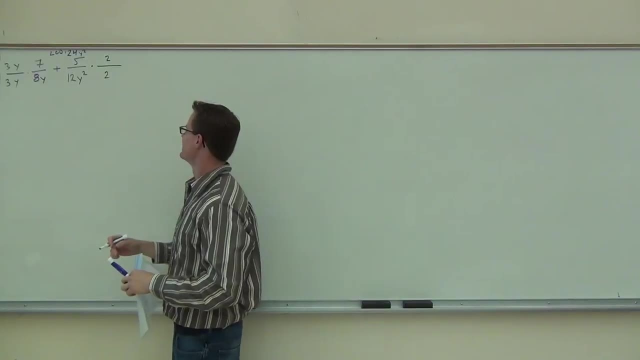 That's a huge. I didn't even finish. that's awesome, quick, good deal. I like it. read my mind. see if we're melding already. no, How many of you made it that far? Good, okay, we figure out what these fractions are. 3y times 7 gives us 21y. 3y times 8y gives us 24y squared. 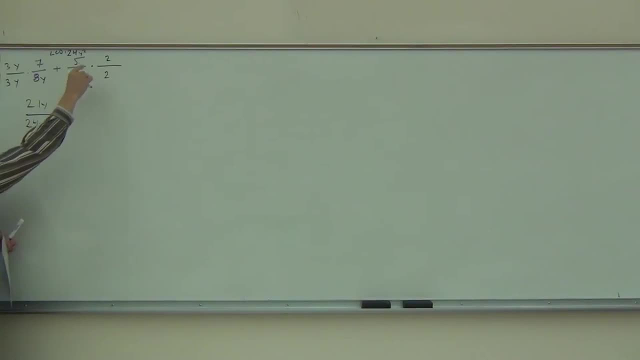 Again, you're just trying to find this thing. that's why we write it down, trying to find this thing on these denominators, And that's what's telling us what to multiply by to get that thing. So, plus to get our LCD, 10 over 24y squared, we see we have an LCD in each spot, so we did our math right. 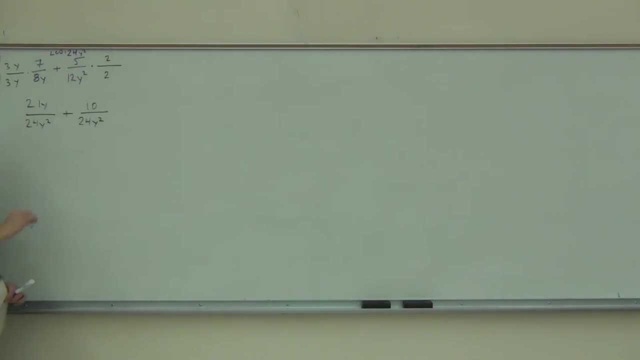 If you happen to do this and you get the wrong or you get different things already you've done something wrong. go back and fix that mistake. you just multiplied by the wrong thing. that's okay. go back and fix it. don't keep playing at the problem, thinking you got it right. 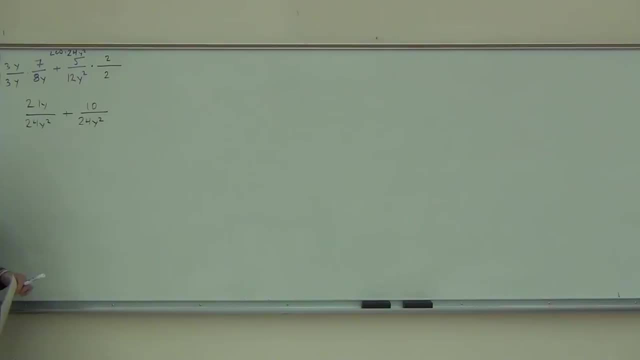 if these things are wrong. okay, We don't want to keep going any further. Last thing we're going to do is add: Since we have a common denominator right now, we're going to get 21y plus 10.. We would try to factor. it's not factorable, so you leave it just the way it is. 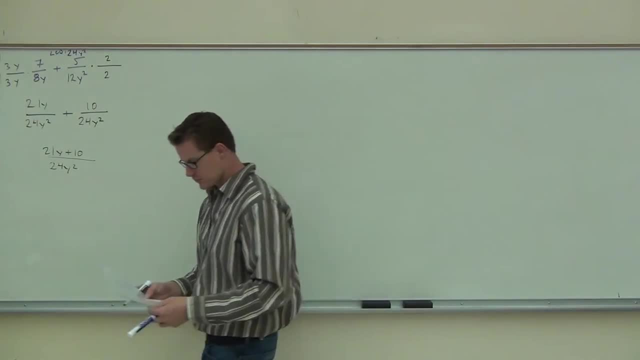 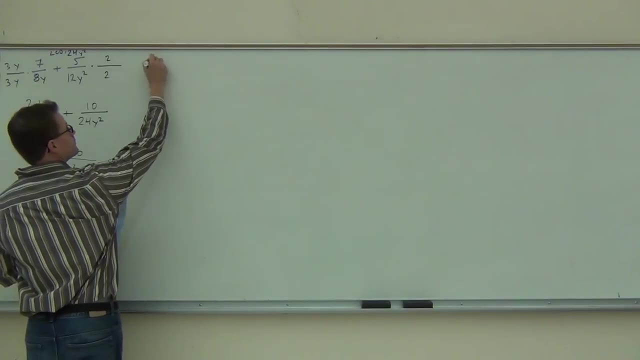 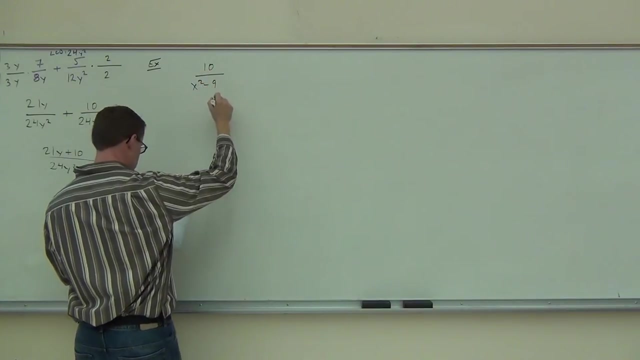 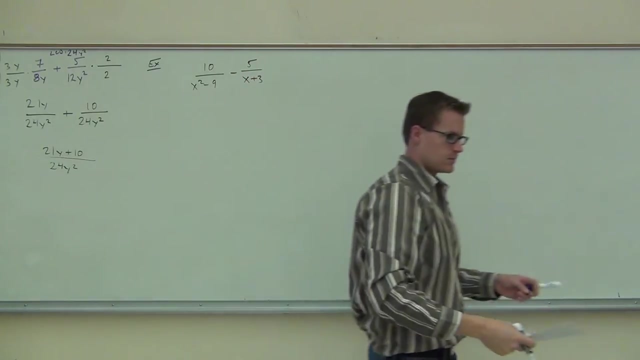 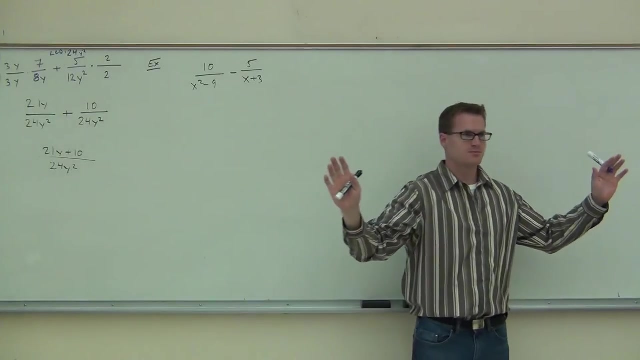 So far, so good. all right. We're going to start making these a little bit more involved and seeing some different problems we can do up here. Uh oh, more than one term. we're done, let's give up. we're going to get this problem too hard. 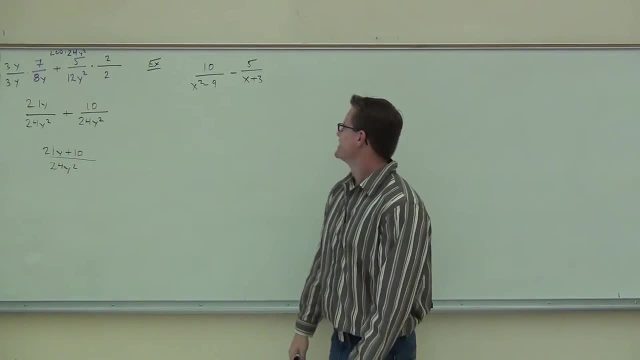 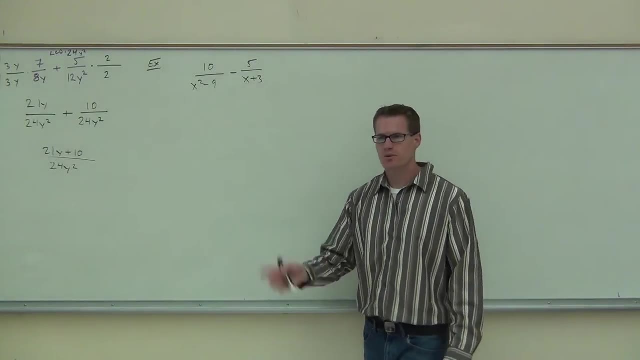 No, no, no. we can't do that other than math class. What's the first thing you might do? What's the first thing you do every time? Yeah, not the numerators. don't care about the numerators, but the denominators. 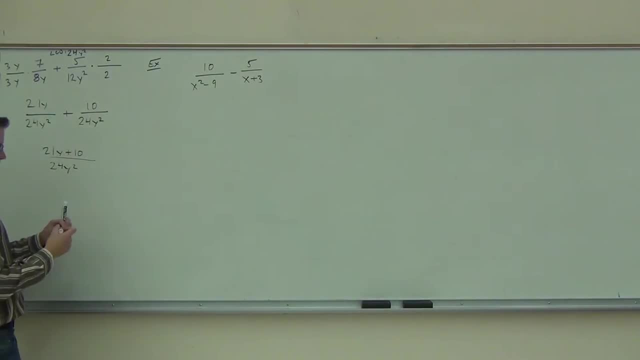 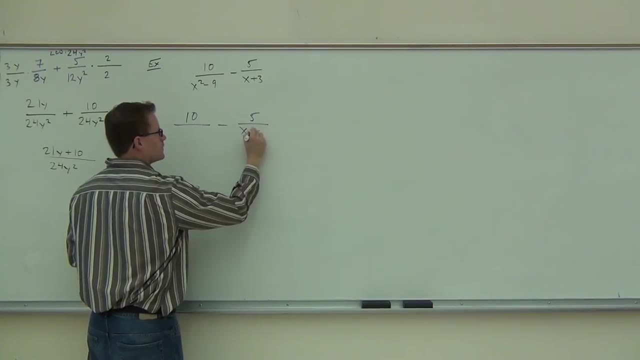 yes, we're going to factor that, Okay. So, first thing, The first thing. let's factor that together. Hopefully you already have a factor. The second one not so much, but the first one you need to be seeing, that's the difference of squares. 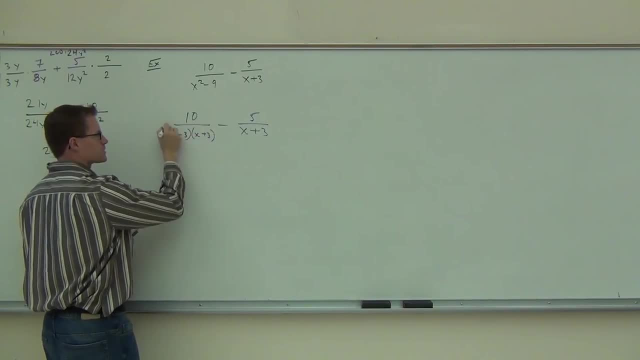 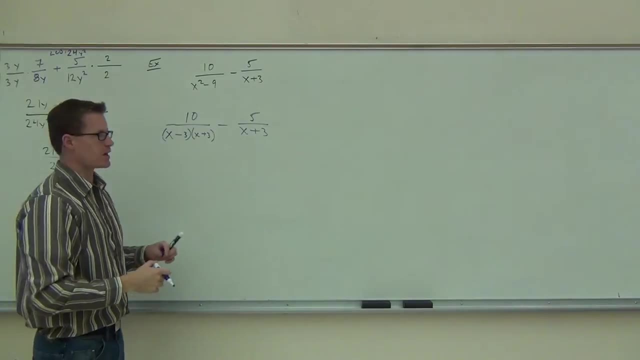 x minus three, x plus three. That should almost be coming automatically to you Almost at this point. it should be, And next week it'll be coming automatically to you. You okay with this one Now? we spent a lot of time finding LCD. 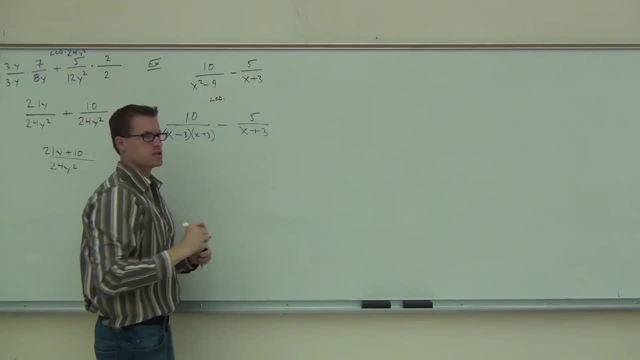 Let's write down our LCD. LCD is the largest power of each different factor, considering all of our denominators. So what are the different factors that you see up here? X plus three. Okay, Here, x plus three. Anything else besides x plus three? 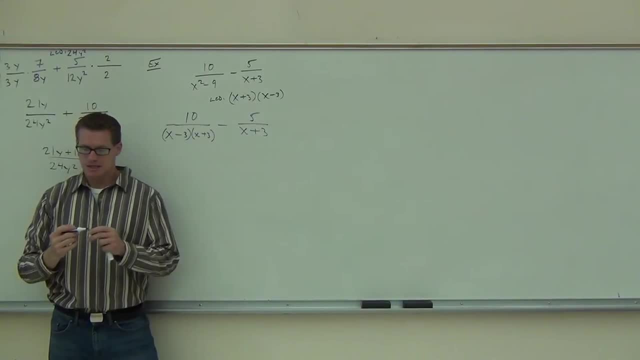 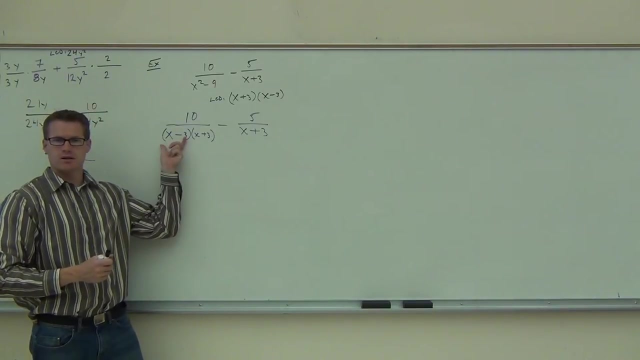 Anything else? Do I need another x plus three? This is just like the LCD stuff we just finished. So all your LCD has to do is be able to cover each of the denominators' factors, the factors of the denominator. So here you'd ask, does it have an x minus three? 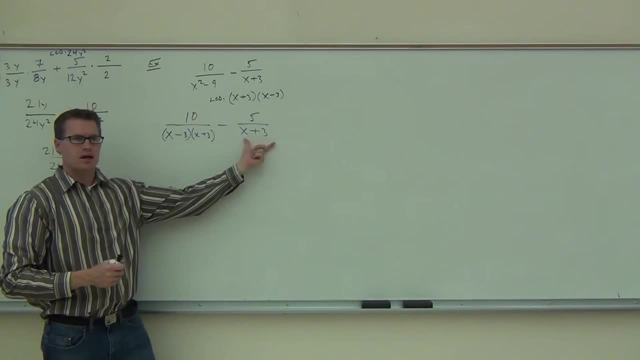 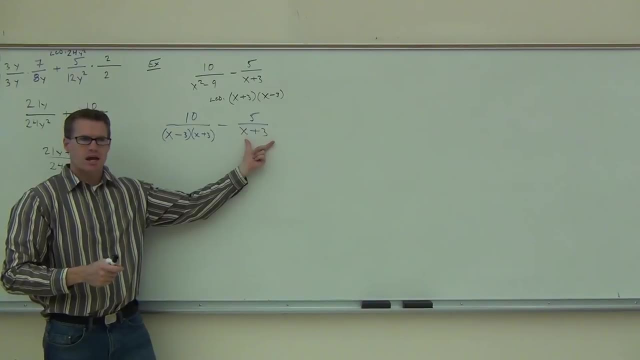 Does it have an x plus three? Does it have an x plus three? Yeah, it covers both. That's fine. That's okay. What would be a problem? here's the problem is if you factored it and you got the same thing twice. 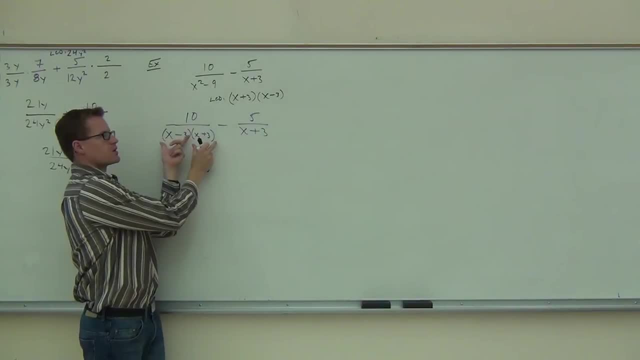 over here, not spread between the fractals, but you got the same thing twice: over here, not spread between the fractals, but over here. then you'd have to combine them and get the square. You see what I'm saying. You got to make it as simple as possible. 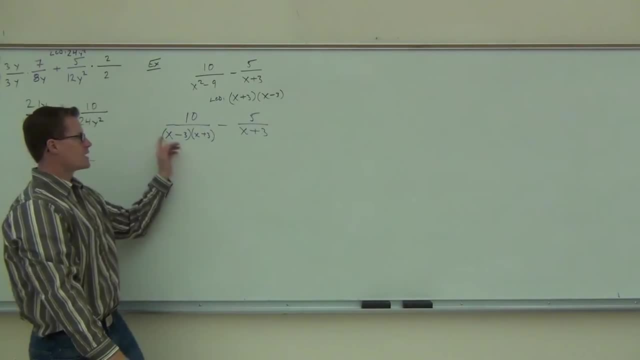 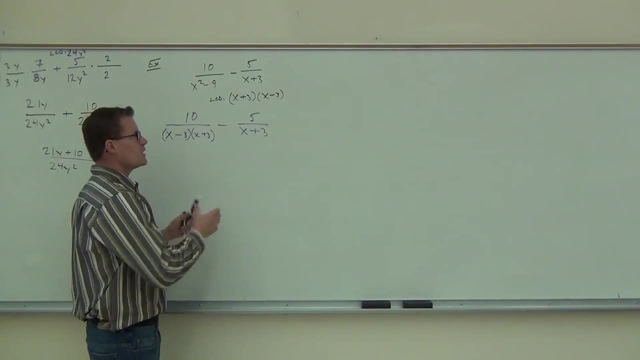 before you find your LCD. That'll take care of everything for you. So here we have our LCD, You're okay on finding that right, And now we're going to multiply it by the appropriate thing to make sure we get our LCD on the denominators. 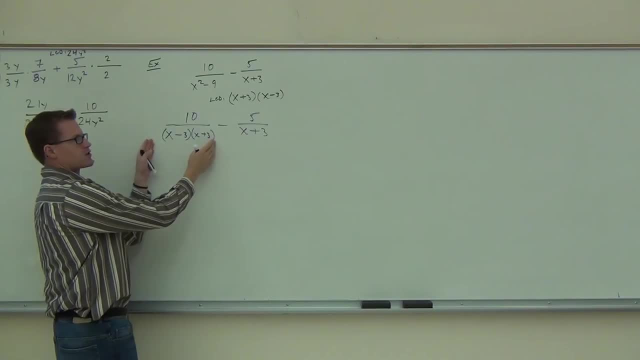 On the left fraction. let's look at that. Do I need to multiply the left fraction by anything? No, It already has it. That's great. That's what we want to happen. On the right-hand side, though, we're missing something. 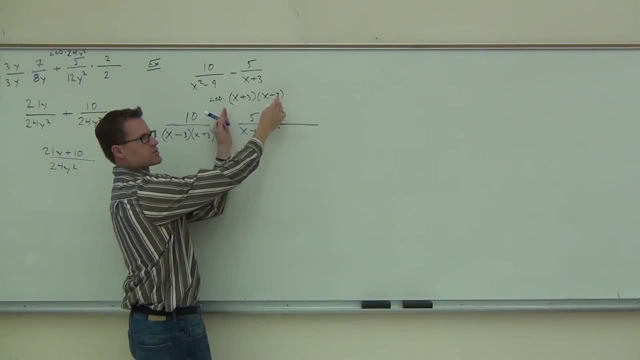 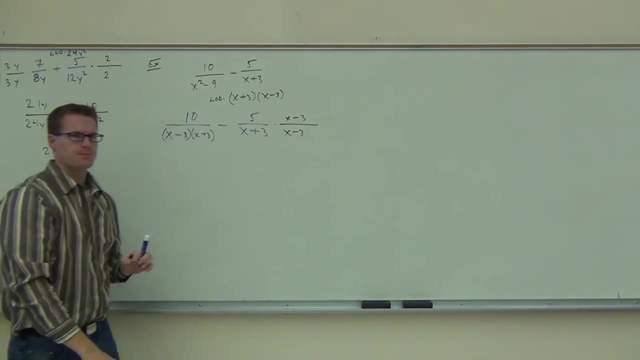 because I have an X plus 3.. I know my LCD is X plus 3, X minus 3.. So what am I missing here? X minus 3.. Perfect, Now we remember how to multiply some fractions right. 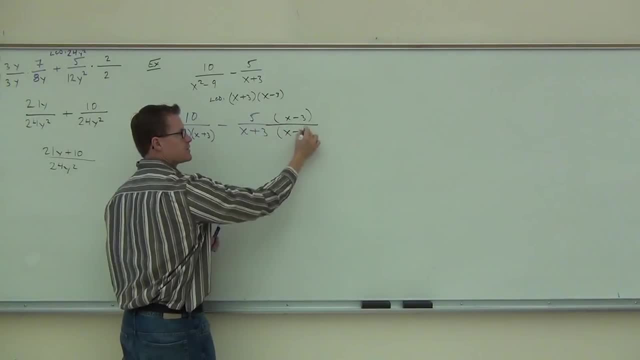 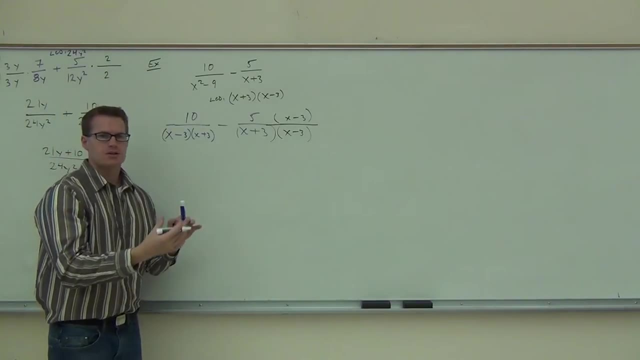 How we multiply fractions is: extend the line. put some parentheses around these things, because that's kind of important. We need to show that. And now that we have our LCD notice, bam, bam, bam, three spots- We can make that into one fraction. 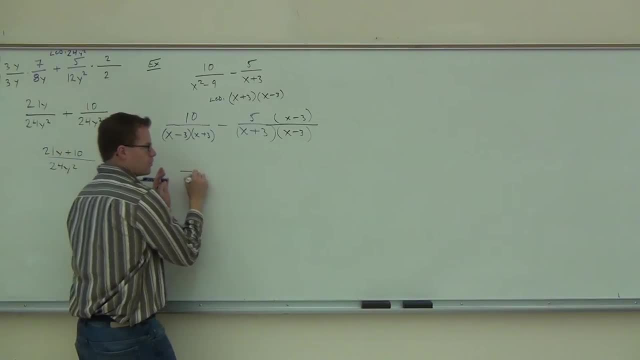 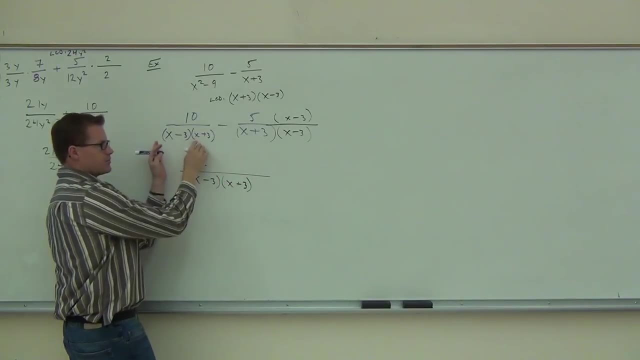 Watch what happens here. okay, When you have your LCD and you make one fraction out of that, your LCD still doesn't change. as long as you have the same LCD here, That's great. We have 10.. What's the next thing I'm going to write? 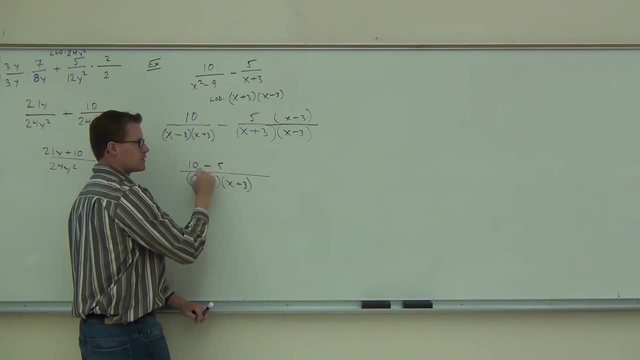 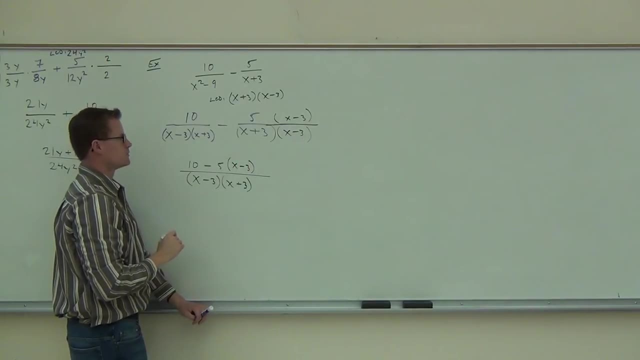 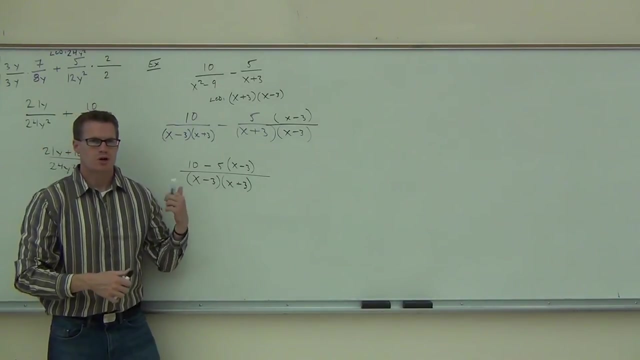 Minus, Minus and then Five, And then There we go, X plus 3.. Are you okay with that so far? Do you remember talking about these things a while back, when we added- and we already had common denominators? 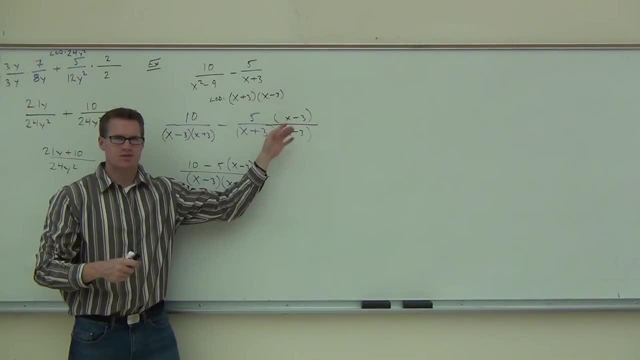 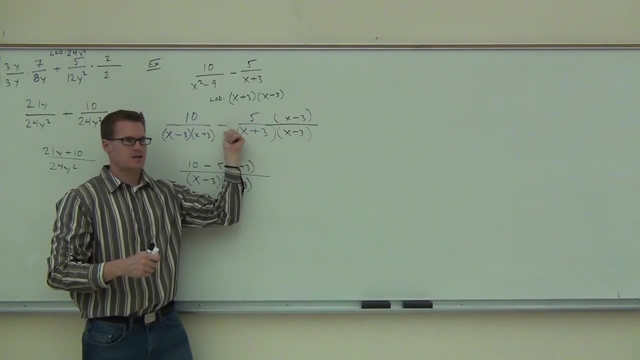 I said: don't do any of this distribution stuff until you get to this step. Do you remember that? Because, why? Because a lot of people, if they distribute here, they're going to forget about that minus sign, And so we're not going to distribute. 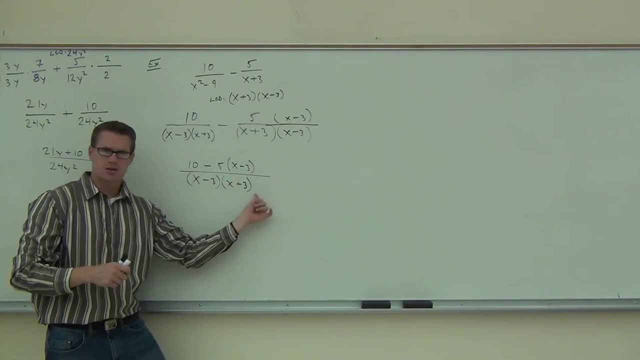 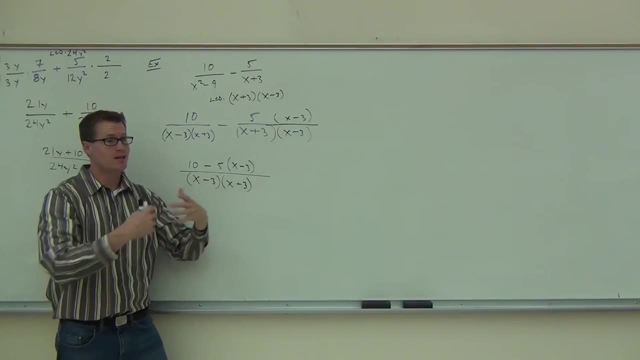 until we get right around here. Then we have to. We're not going to distribute denominators ever, But we will distribute the numerators, all right, Because we've got to combine like terms. So we're going to wait, We're going to do our LCD. 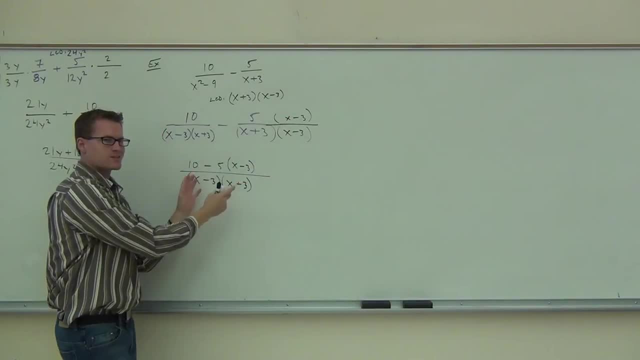 We'll use the LCD to find a couple rational expressions. We'll make one fraction out of it. That's great, But then, right here, we're going to wait to distribute to this point, Because now we can see it's not just 5.. 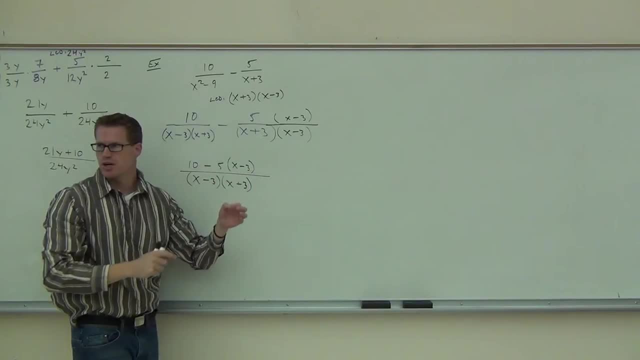 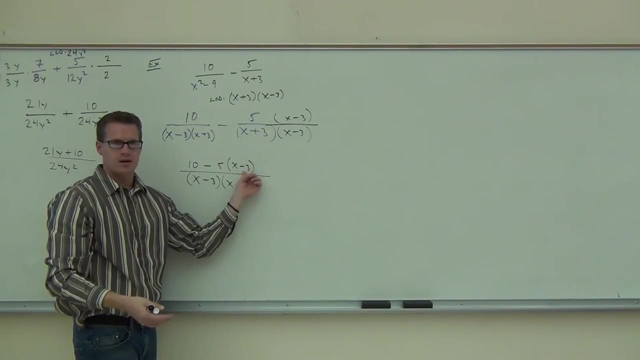 It's minus 5 that's going to distribute. Are you seeing that The second sign will change? And again, of course, where do I look? I look right there on your problem. on a test, If you have a minus still, I know you don't understand it. 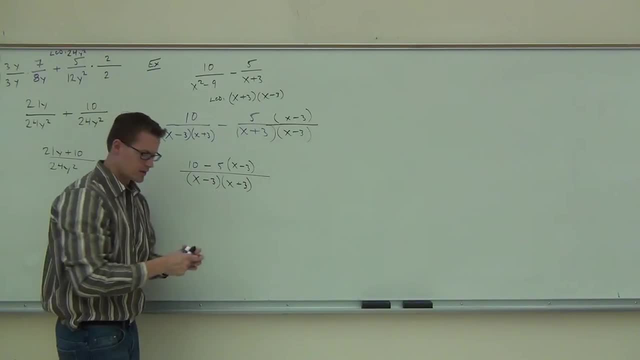 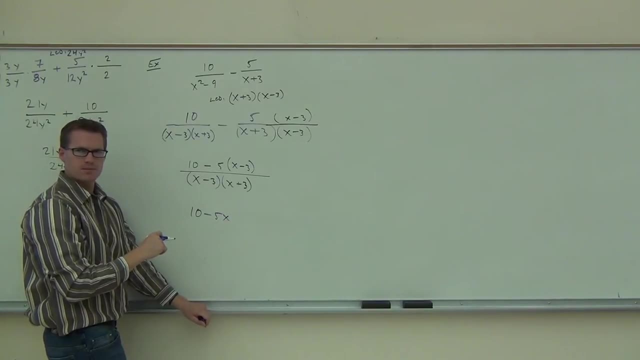 If you have a plus, I know that you distribute the negative appropriately. That's where I look. It kills me a lot, So I get the 10.. I get minus 5x. I get, not minus 15.. What do I get? 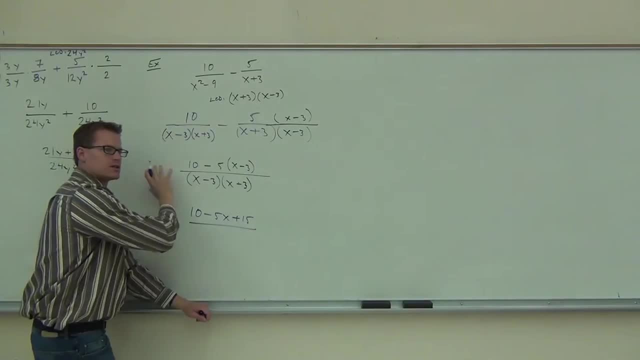 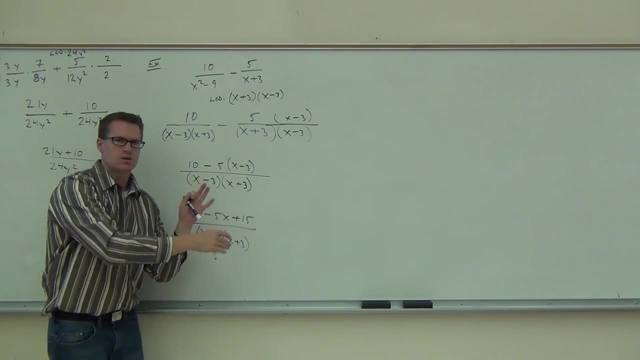 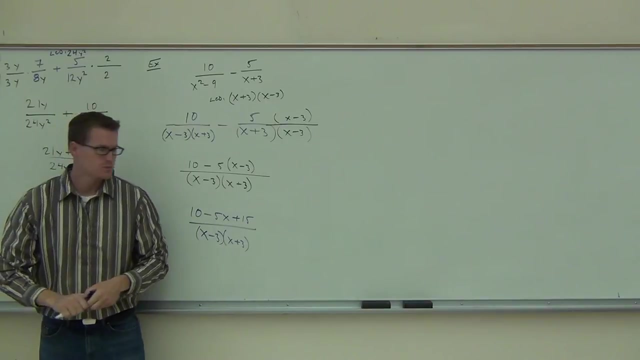 Over. I'm going to leave the denominator exactly like it is Once you find this part. unless you can simplify the end, it stays the same. Last step: what are we going to do now? So some like terms. We're going to get how much? 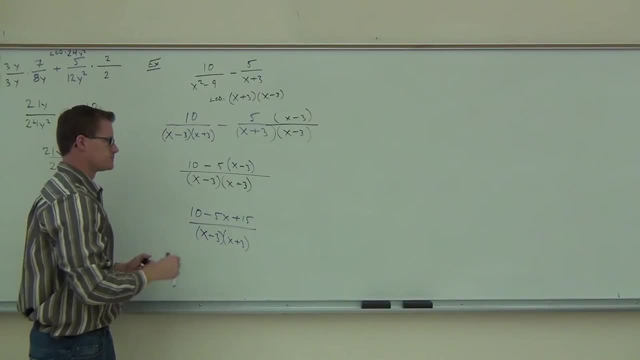 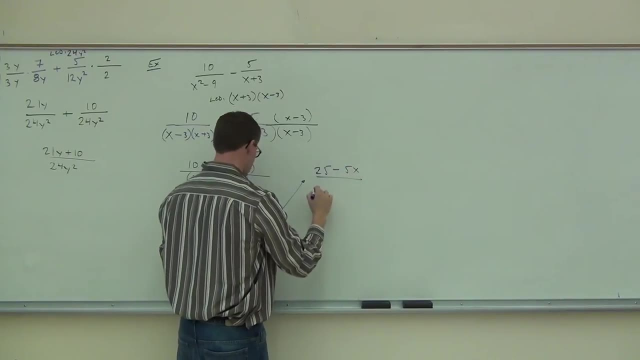 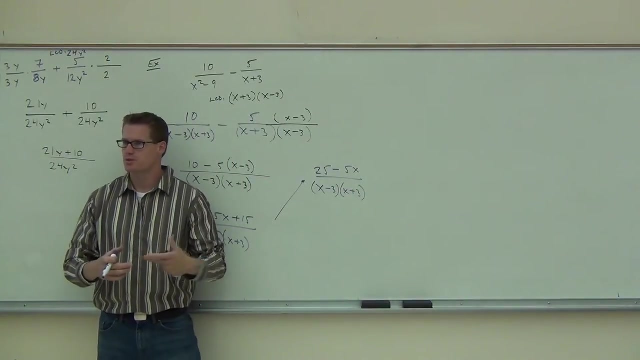 Okay, Either way you want to write that, It doesn't really matter. I'll choose to do 25 minus 5x. Now the next thing you do after you combine your like terms. Are you okay on this? first, That part. 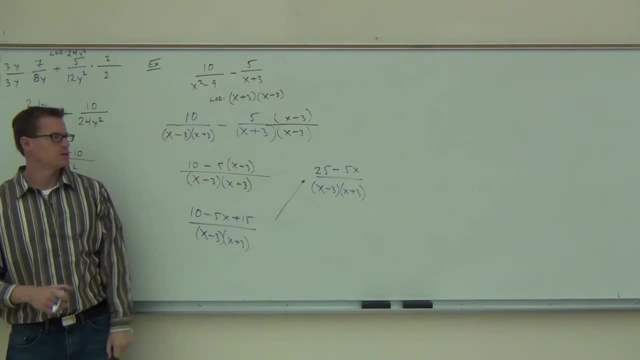 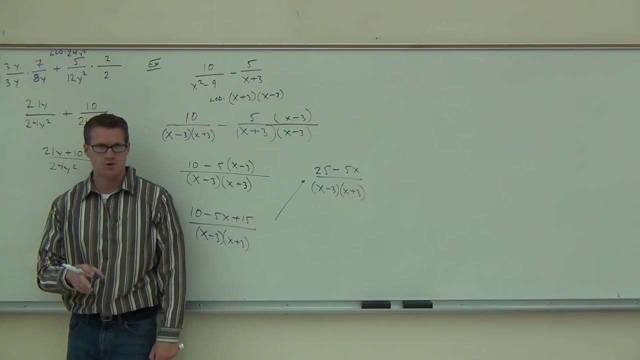 Yeah, Next thing you try and do is factor that. Now I see that a 5 factors out of that, Or a negative 5. you want to make thex explode, So that's 5. x positive, like you're supposed to. 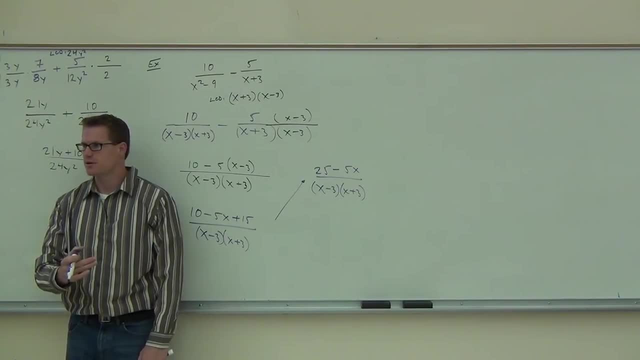 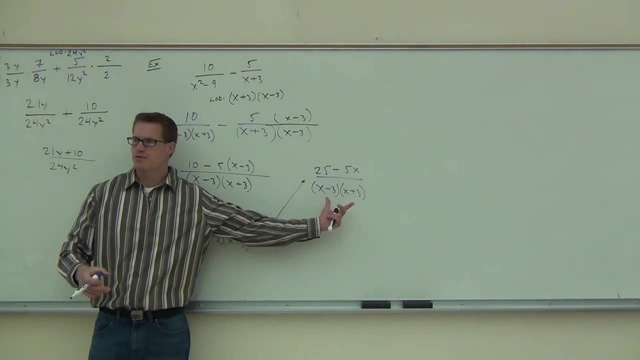 However, if you do that, are you going to be able to simplify anything? No, because you're going to get 5 minus x or x minus 5 if you factor out the negative. It's still not going to simplify, so I'm going to leave it up to you all, right? 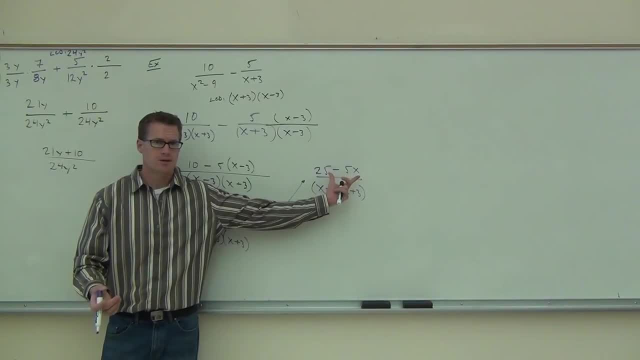 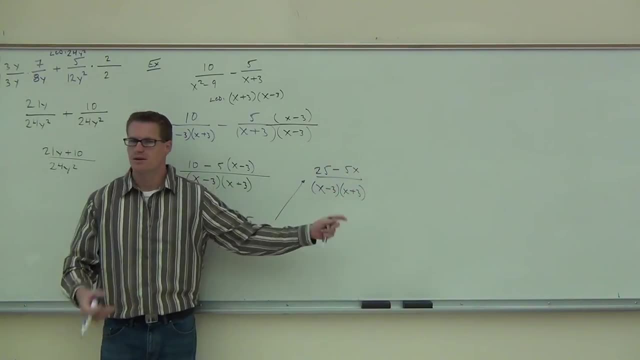 If you want to, you should try to factor, at least in your head, because that's going to tell you whether you simplify something or not. But if you know that even if you factored it it's not going to simplify, you can leave it, that's fine. 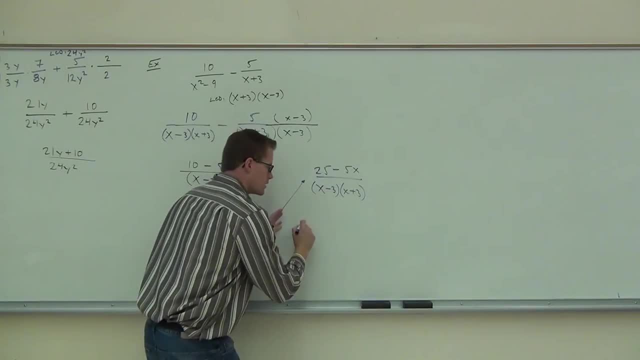 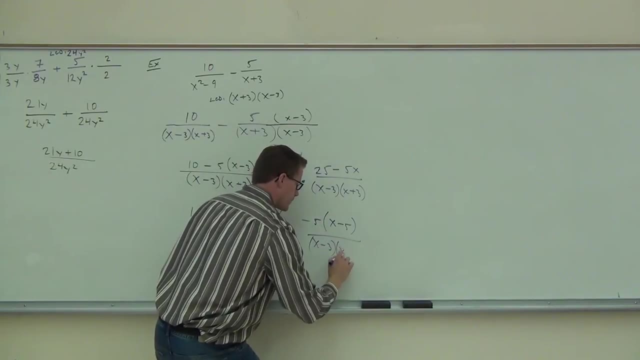 OK, if you factored appropriately, this would be the other option you have. You'd factor a negative 5, you'd get x minus 5, after you switch things around over x minus 3, x plus 3.. That's another appropriate answer. 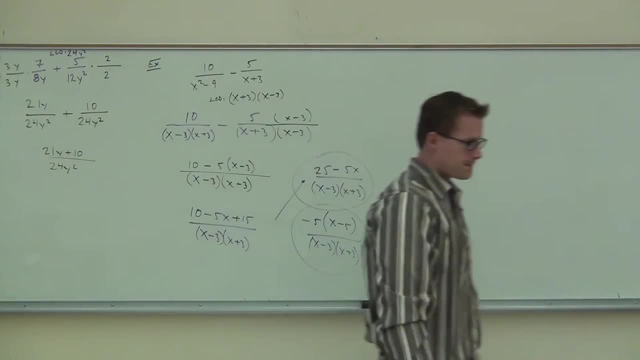 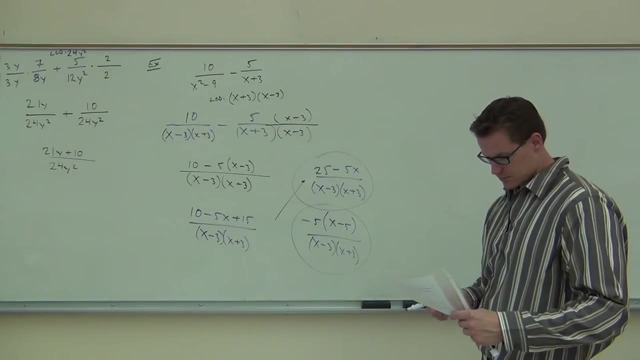 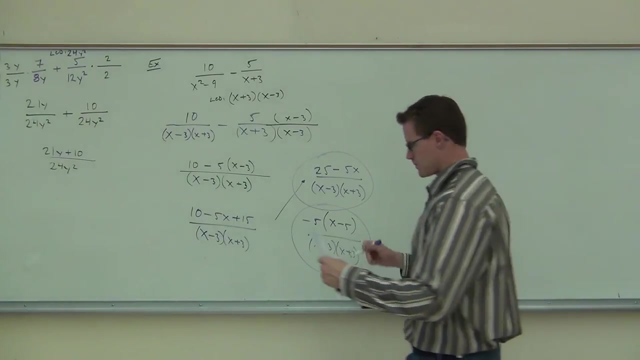 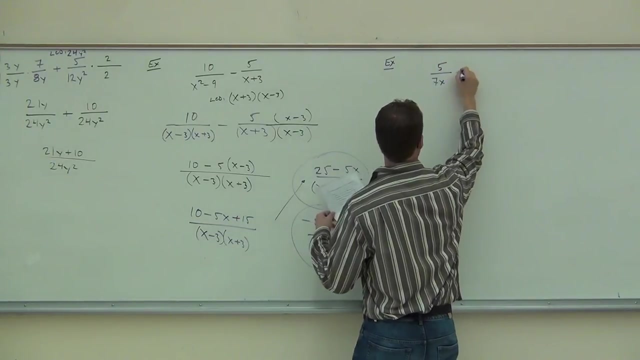 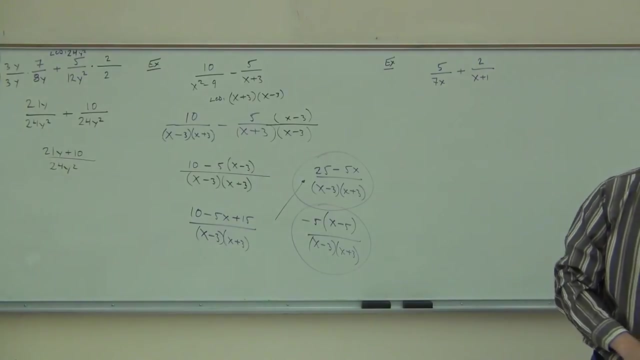 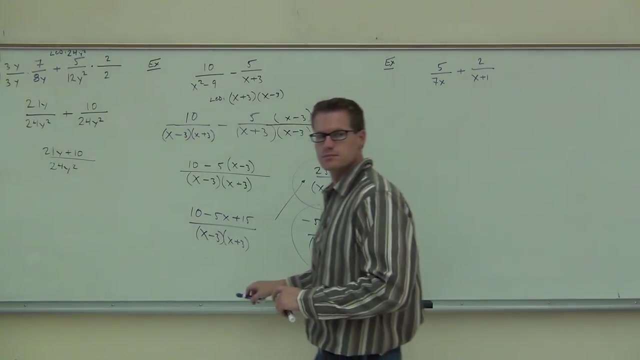 Either one of those is appropriate, because that's not going to simplify out. Do you feel good about that one? Let's try it a little. OK, first things first. Since we don't have a common denominator, the first thing we need to do is find what. 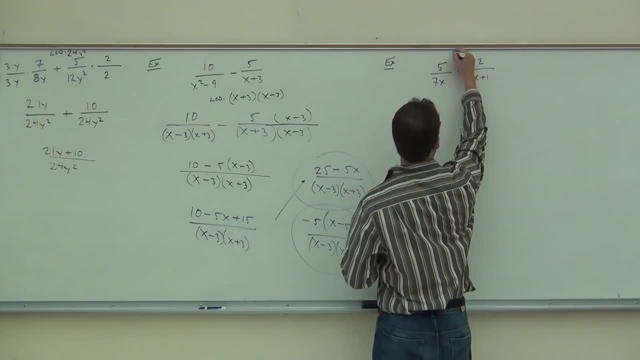 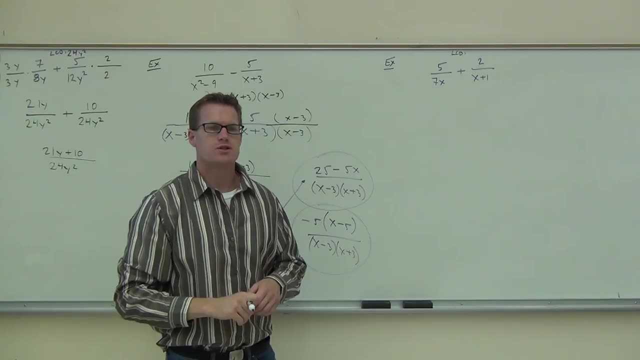 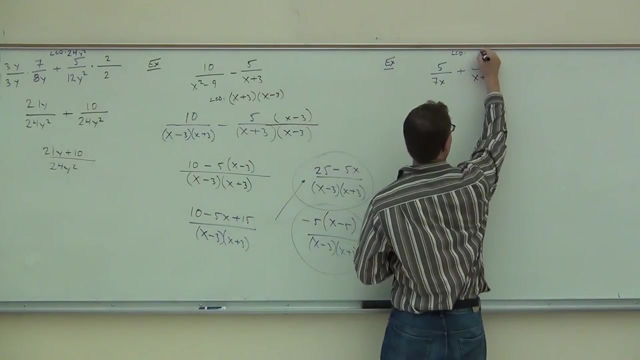 Let's find the LCD. The LCD must include all the different factors up here. So can you tell me what's one thing that has to be in my LCD? x plus 1? definitely has to be there, you're right. OK, is that the only thing? 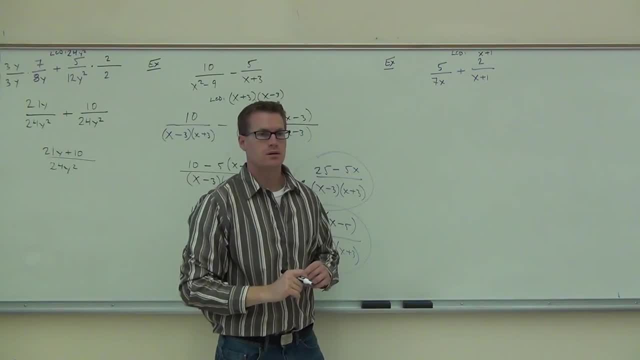 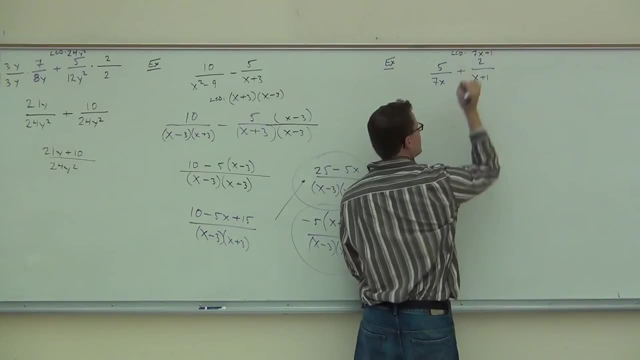 x plus 1.. OK, I got x plus 1.. Oh, 7x plus 12.. OK, the 7 has to be there, that's for sure. Now my question is: can I write? is that OK? 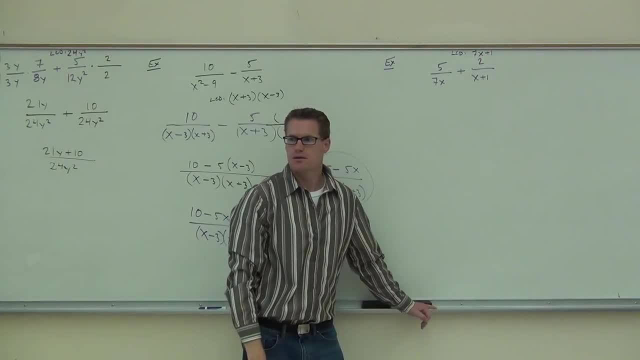 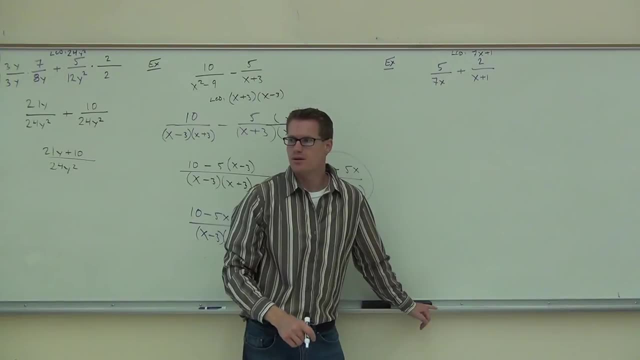 Just the 7x plus 1, like that. No, because what I've done is I've changed something from a factor to a term. Right now the 7 has to be a factor and right now the 7 is incorporated with a term there. 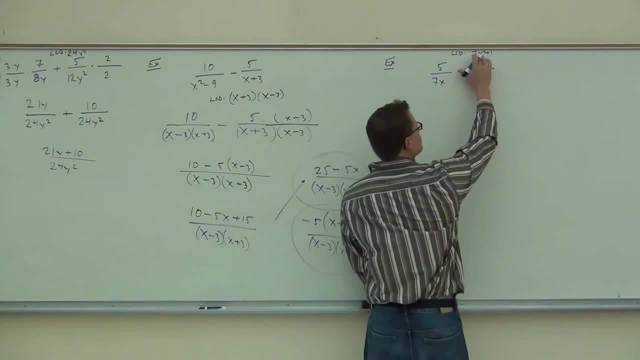 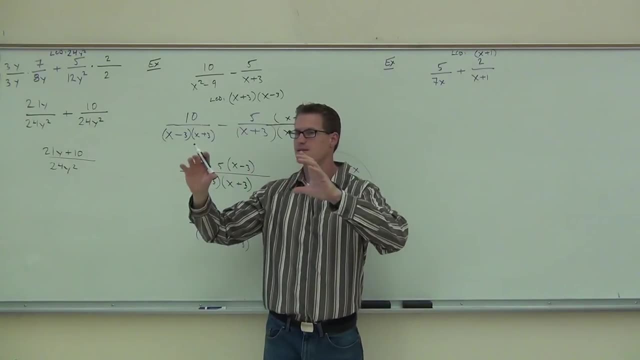 It's not OK, that's not good for us. So if I say x plus 1 has to be there, x plus 1 has to be there by itself, right like that. OK, that's the way x plus 1 needs to be written. 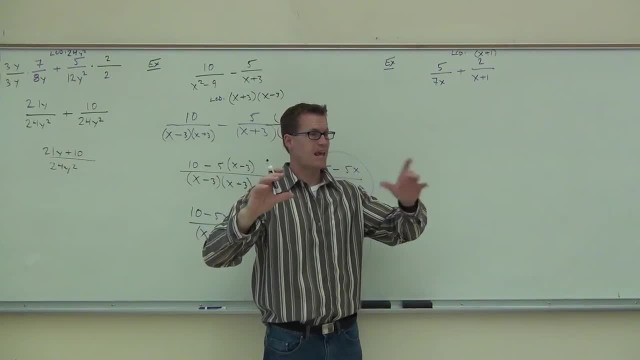 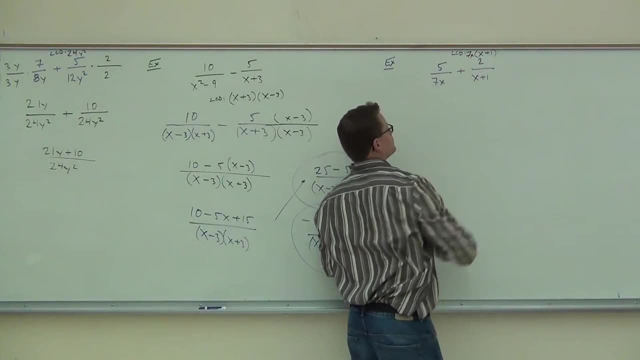 Then also, I'm missing something else. What am I missing? 7 and the x. I'm missing the x That we talked about this a long time ago, that x doesn't count, Not for this x. So we have 7x times x plus 1, that's our LCD. 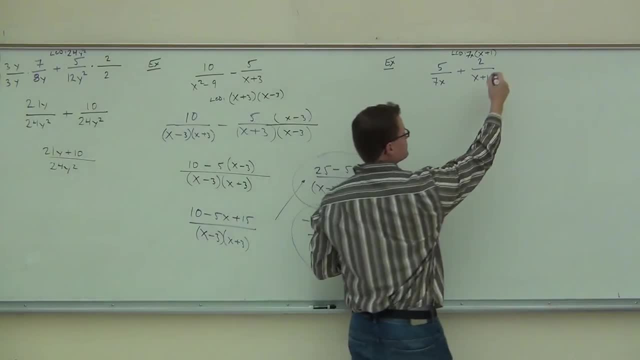 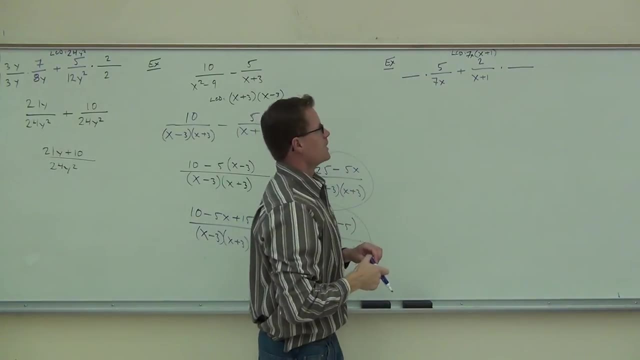 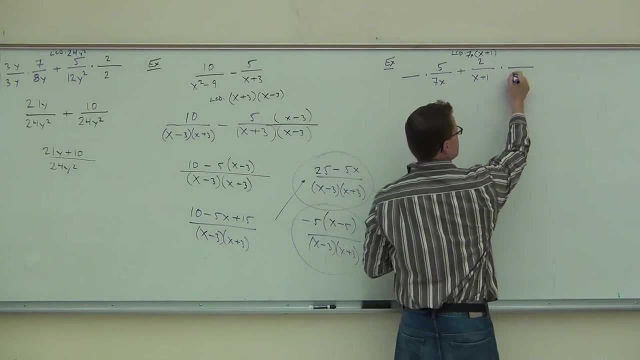 Of course we're going to use that. Let's see if we can do this thing Over here. on the right fraction we have x plus 1.. What are we missing? What do we need there? 7x. So that's going to be on both the numerator. 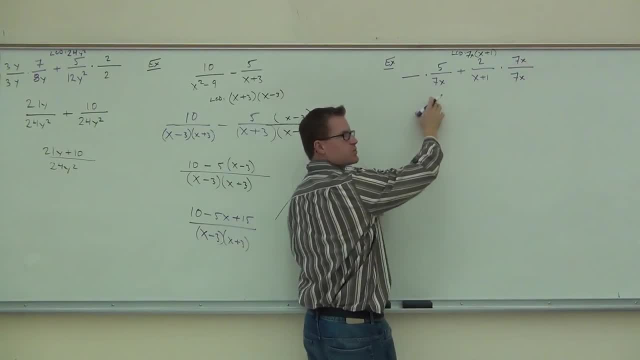 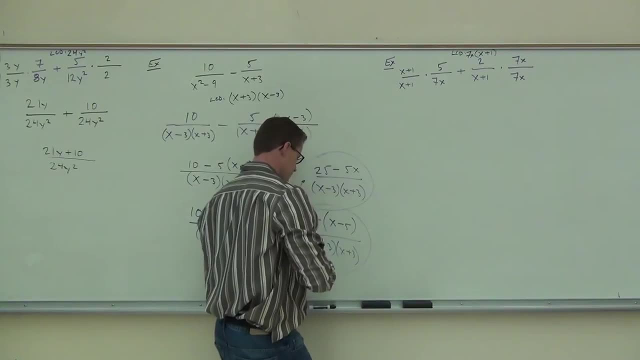 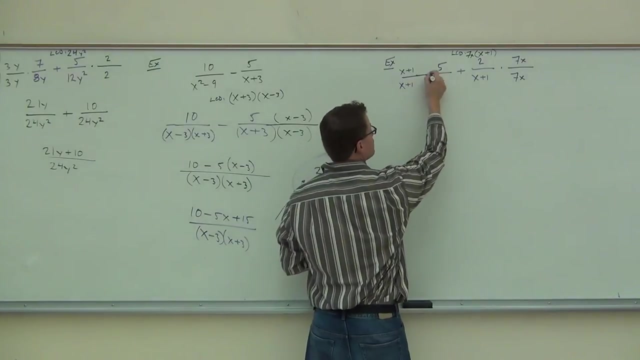 and the denominator, And over here we already have the 7x, but we don't have the x plus 1.. We're going to multiply fractions, like we know how to do already. We're going to extend the line. We're going to put the dot dot. 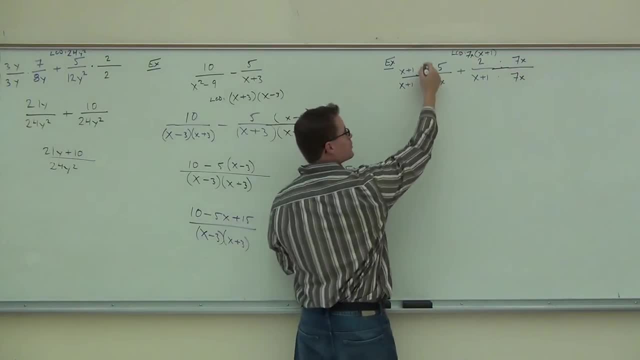 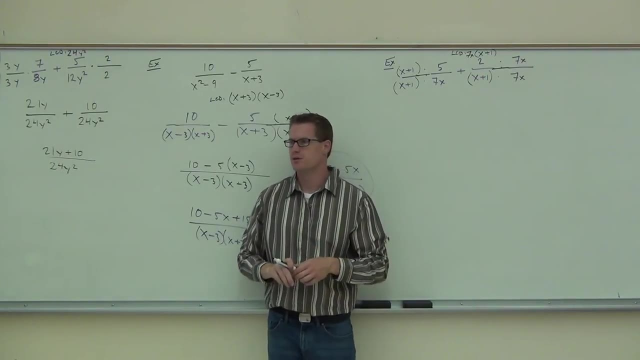 Extend the line with the dot dot. Make sure we have some parentheses where appropriate, like here, you have to have them, and here and here. Ladies and gentlemen, do I now have a common denominator? Yes, Do I now have a common denominator? 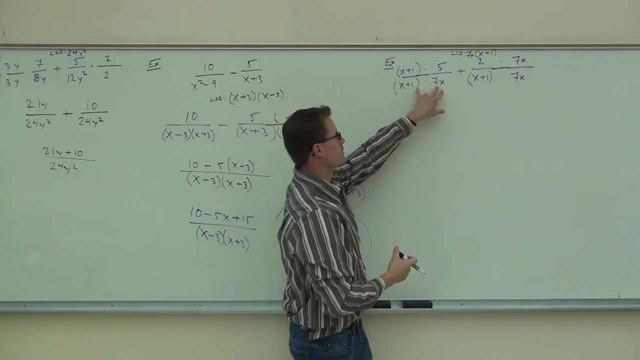 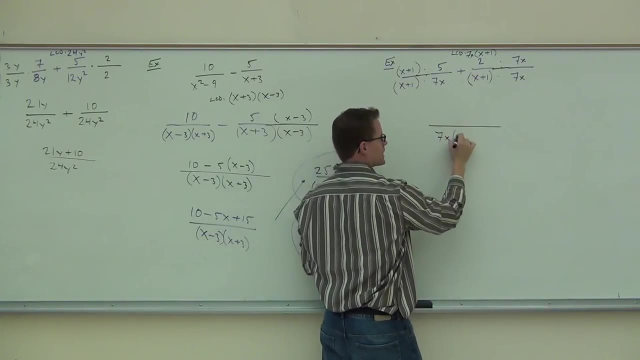 Does it have all the stuff there? Yes, So I have this and I have the same. I'll probably write it a little different in the next fraction. Instead of x plus 1 times 7x, I'll write 7x times x plus 1.. 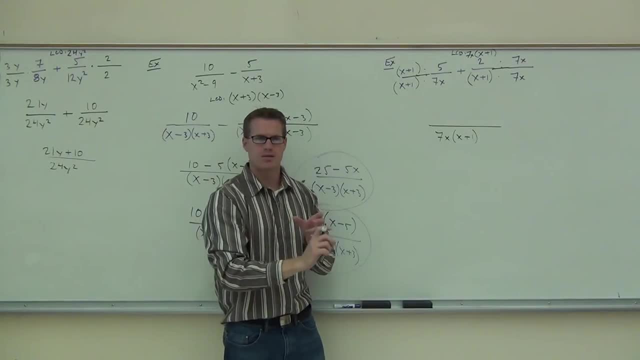 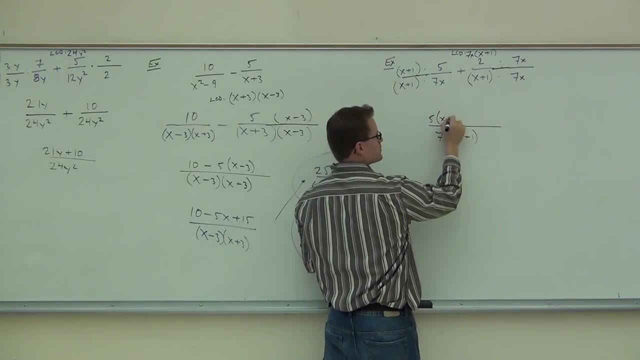 Since multiplication is commutative, it really doesn't matter how I write that. I choose to write the 7x first. On the numerator, I'm going to choose to write the 5 first. 5 times x plus 1 plus. how much is that? 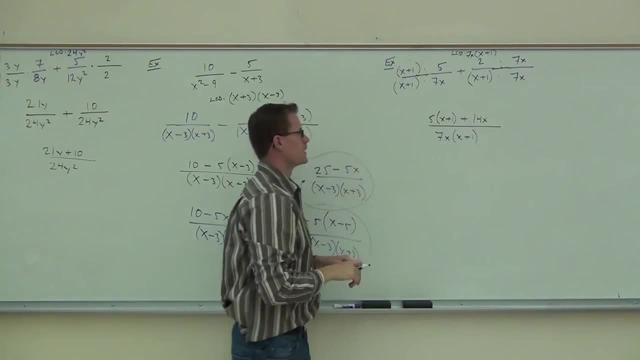 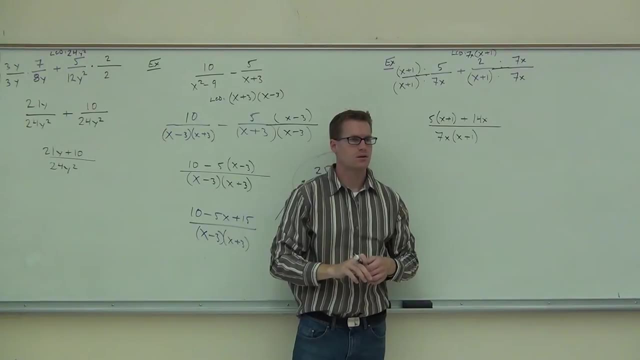 14x, 14x, 14x, 14x, 14x. Ladies and gentlemen, raise your hand if you're okay on making it this far Question. Sorry, I'm wondering if I could pass away to show you. 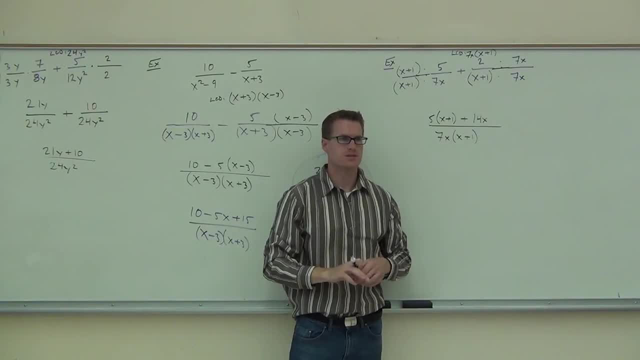 what each of those steps are Absolutely, And then you just do it. No, Yes, Because this is how I check to make sure, Because not everyone's going to get these right. I wish that would be the case, but it never has been, ever. 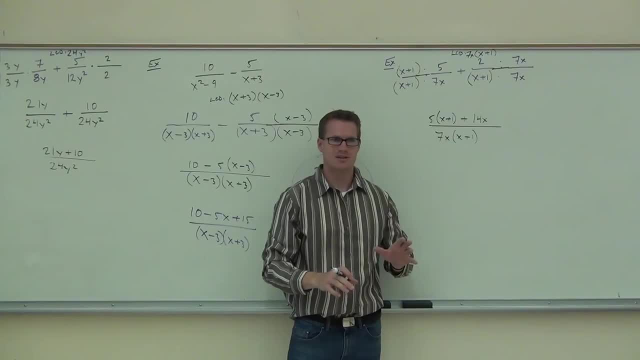 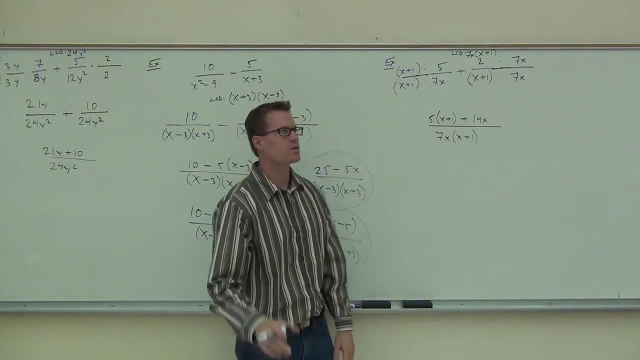 in the history of the world. Just kidding, But I need to see where people are making mistakes, So I can't let just single people not do that, right, Yeah, Yeah, Okay. one other question I have for you in the last. 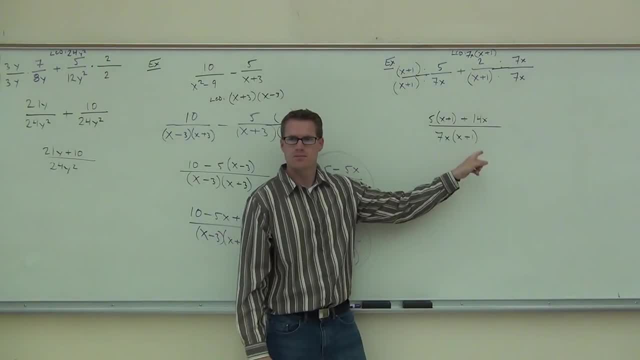 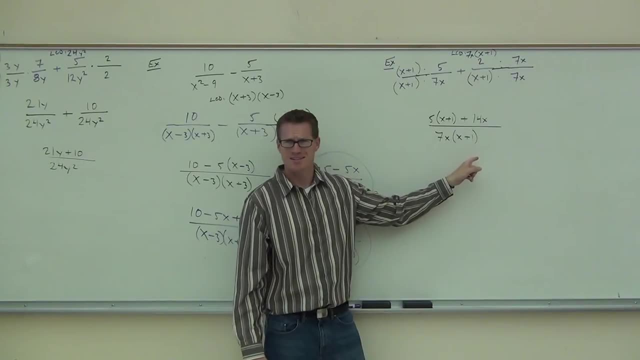 oh, two seconds. Can I simplify those? Yes, No, Shake your head. no, No, No, Mr Leonard, Are you crazy? No, Can I simplify those. No, One more time. everybody, Can I simplify those? 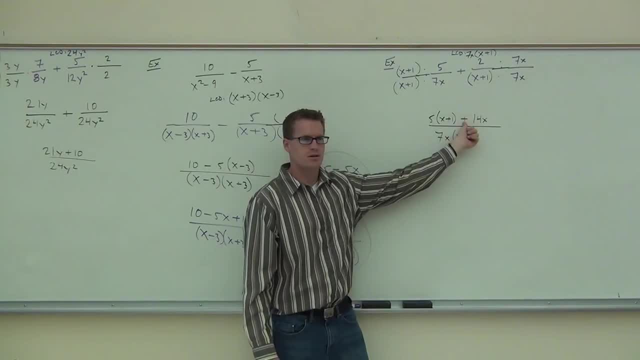 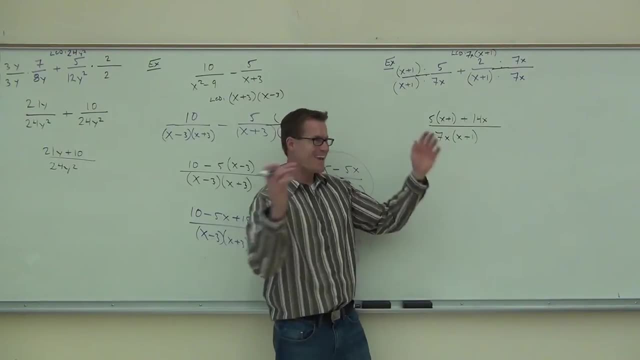 No, No, The reason why. do you notice that that's connected by addition? Yes, This is one of the biggest mistakes in calculus. I see, okay, In calculus, this is one of the biggest things. People go: yay, We're done. 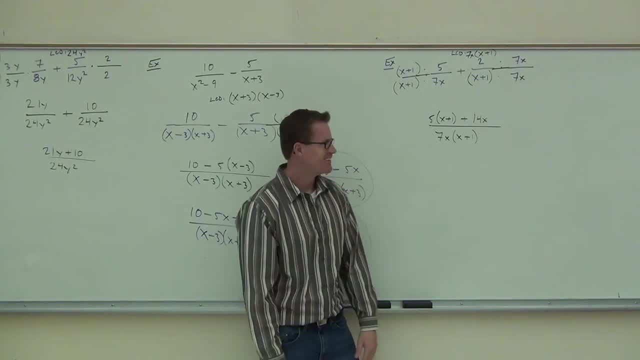 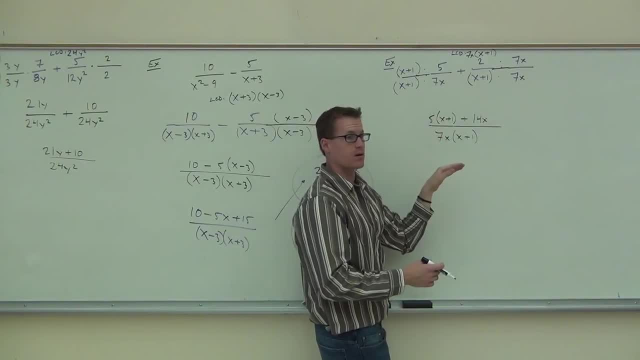 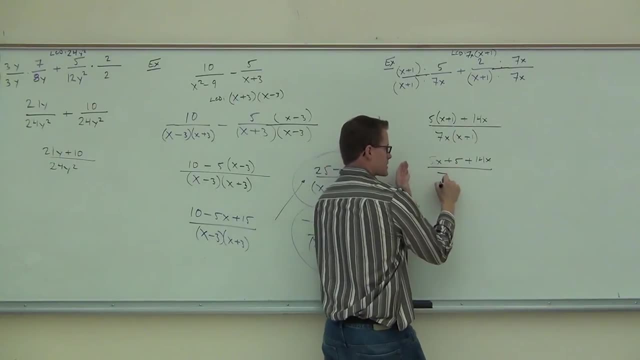 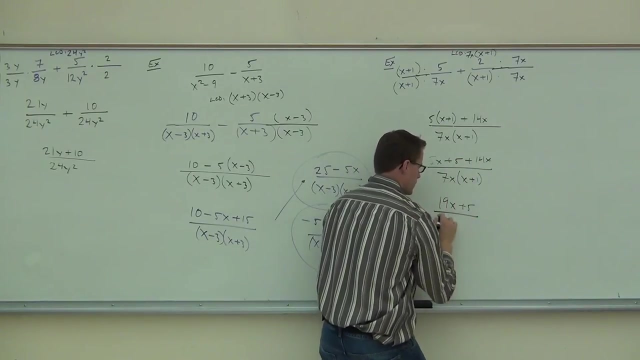 term and a term you cannot. you cannot cross it out. what you can do is distribute 5x plus 5 plus 14x over. leave this the same. 7x x plus 1 combined like terms 19x plus 5. 7x x plus 1. okay, next question: can I simplify these X's? no, no. 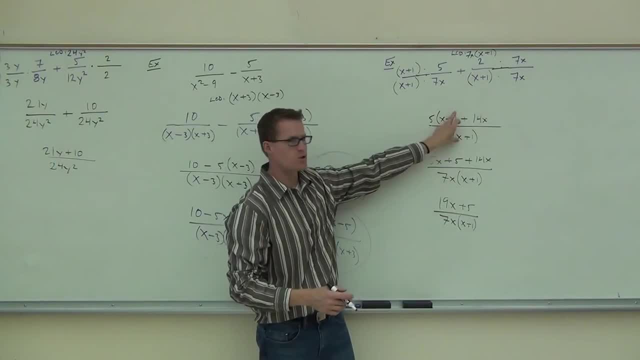 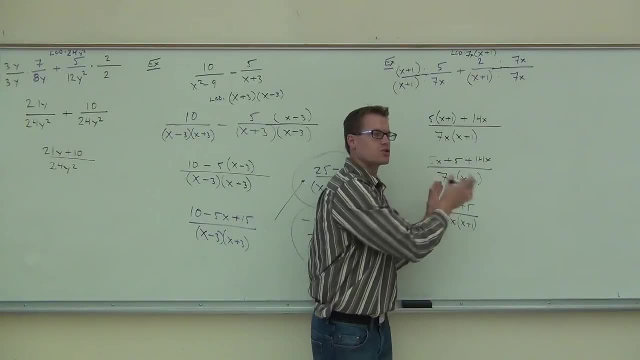 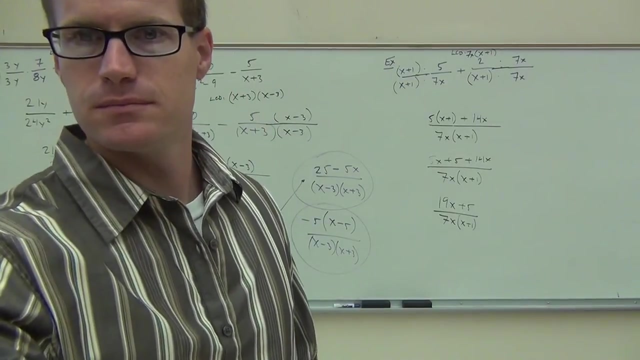 no, this is actually more clear. this is a plus. okay, that's the same question I said here in a, still connected by a plus. you cannot do that stuff to the very last step. after you factor and cancer, we can't factor this, you're done. so you want it written like that at the bottom. that's the one, okay. 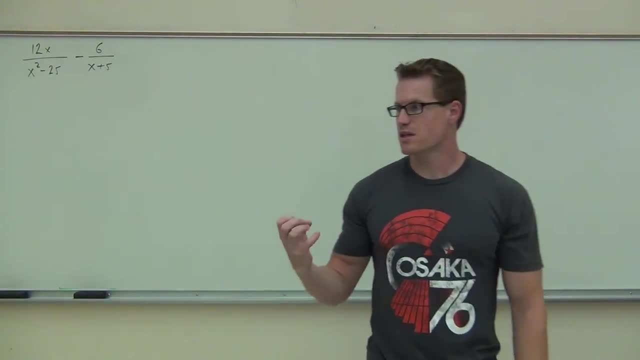 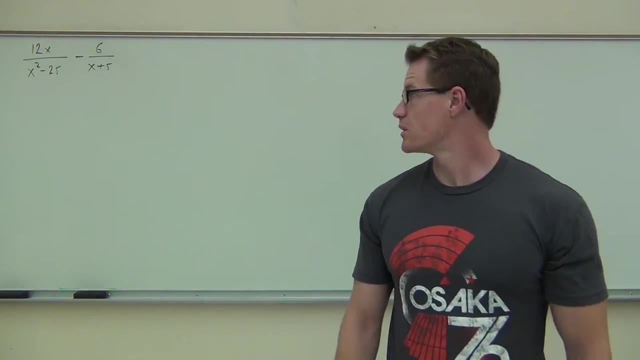 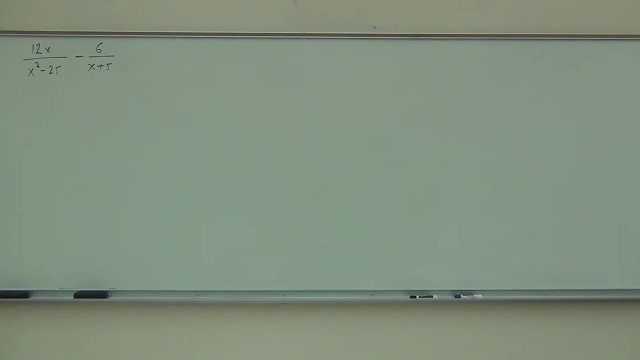 all right. so, if you remember, we're trying to factor the denominators of these things, find out what the LCD is using that to make up an equivalent rational expression and then we get to add and subtract those add or subtract those fractions. if you finish that one quickly, there's another one that you can work on. 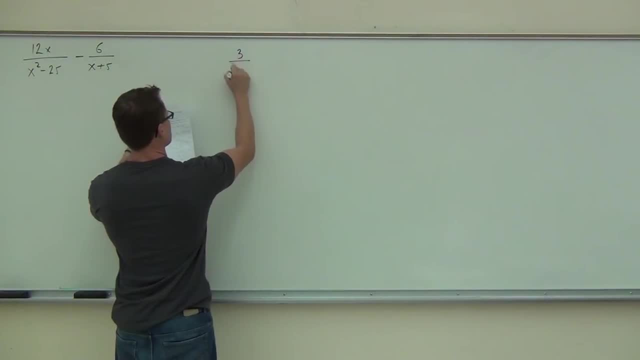 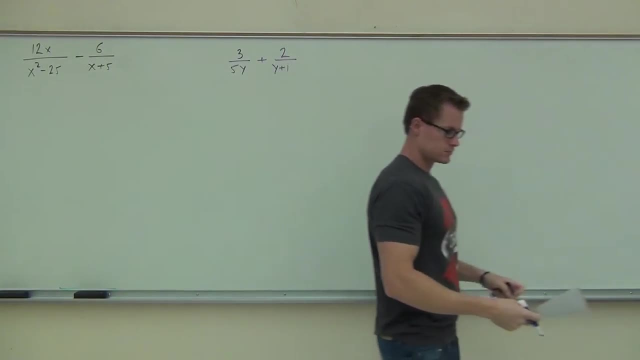 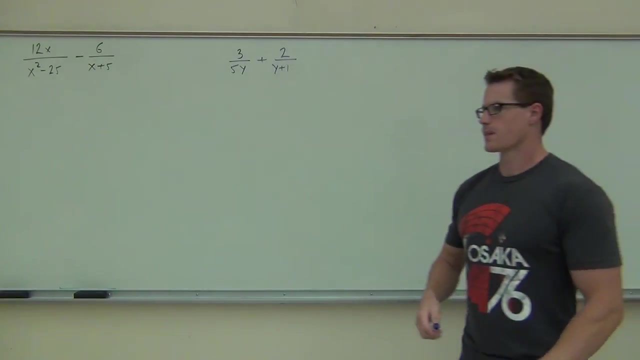 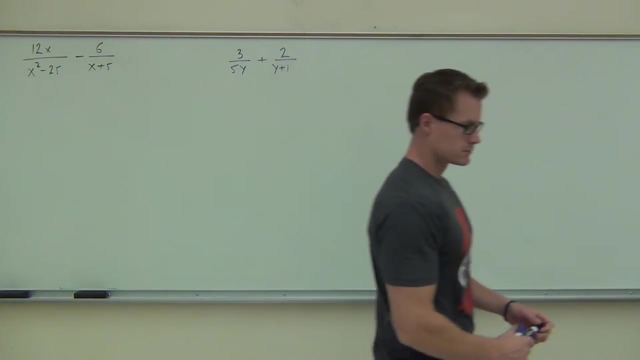 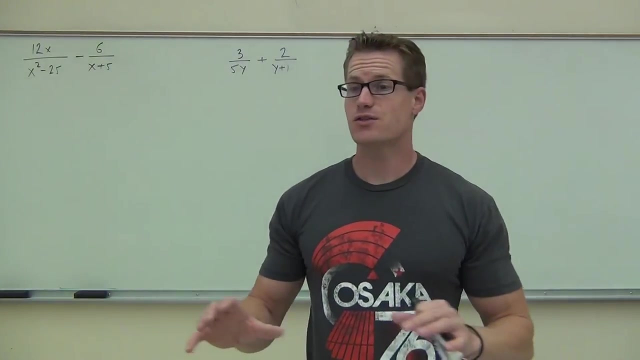 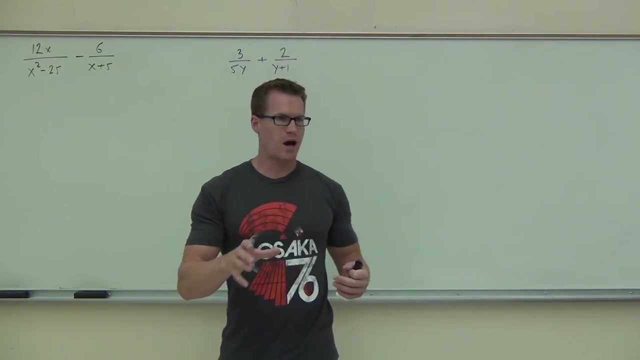 later. Thank you, Alright, guys, let's get started with this thing. So we know, when we're dealing with rational expressions, the first thing we always do is at least factor the denominators, And especially in this case, because if we're looking for the LCD, what we know is that the LCD is the largest power of each different factor. 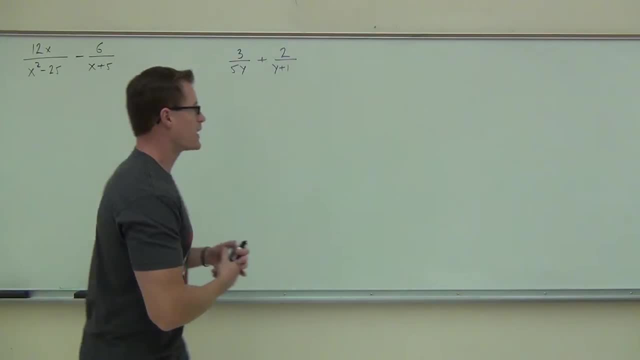 We can't find factors unless this thing is, of course, factored. So when we factor our first example here, the x plus 5, we leave that alone. there's nothing we can do there. However, the x squared minus 25, that should just be instant for us. 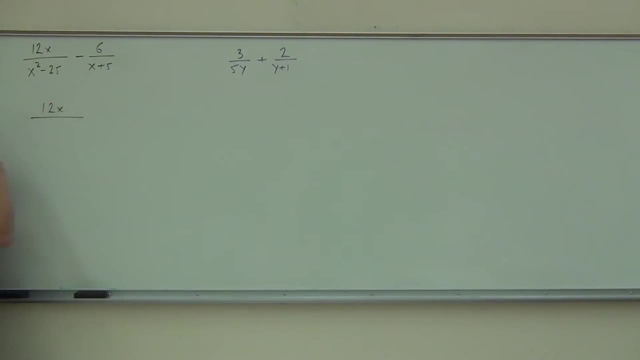 We're going to get 12x over. what's that? Factorize Sure, And you know it really doesn't matter the order, you can switch those things around. it's fine. Did you factor? that? okay, Then we go and find our LCD, because we realize right now we do not have a common denominator and we need one. 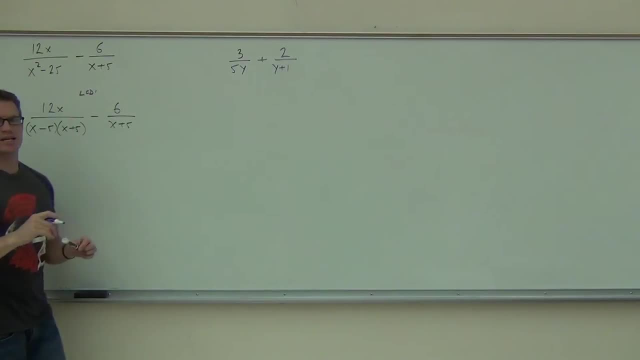 So our LCD is basically just a listing of all the different factors. So when I look at this thing, I see the x minus 5.. I see the x plus 5, and then I have an x plus 5 over here. but because that's in a different fraction, it's already counted. 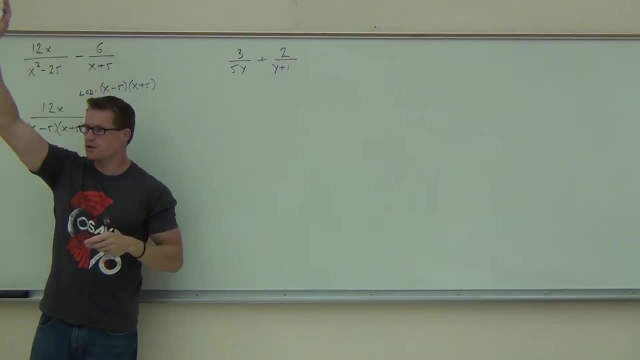 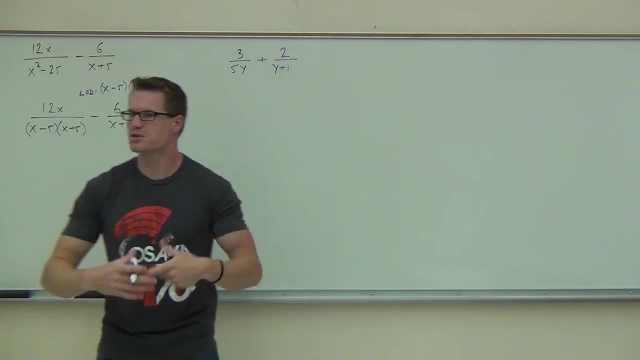 We've already got the LCD. how many people were able to find the LCD Good? Now we're going to use that to make some equivalent rational expressions. That means fractions of the same value. it just looks a little different. We're purposely unsimplifying here. 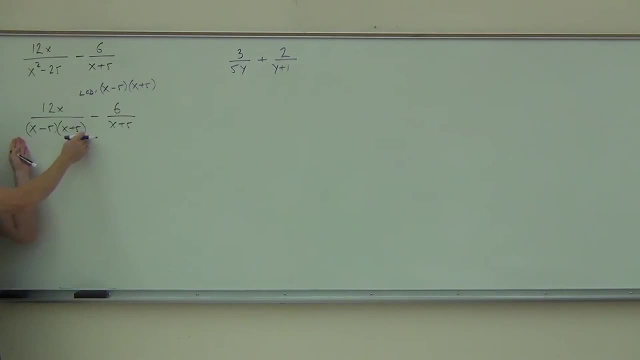 On the left-hand side, I already have the LCD down there. that's great. I don't need to do anything to that fraction. On the right-hand side, though, well, I have x plus 5, that's great. I don't need to do anything to that fraction. On the right-hand side, though: well, I have x plus 5, that's great. I don't need to do anything to that fraction. On the left-hand side, though, well, I have x plus 5, that's great. 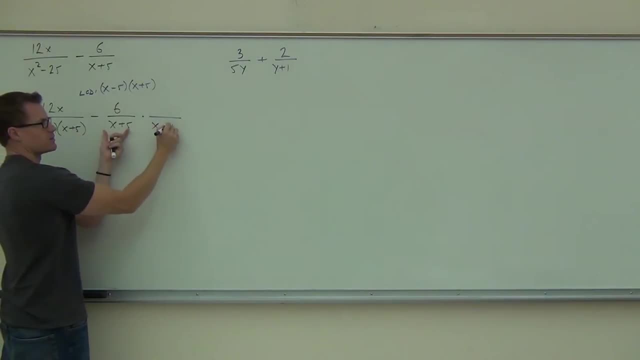 But what else am I missing? And that's what I'm going to be multiplying by. Of course, we know how to multiply fractions. we extend our line, we put parentheses where appropriate, And what we get to do now is, instead of distributing right now, instead of distributing right now. 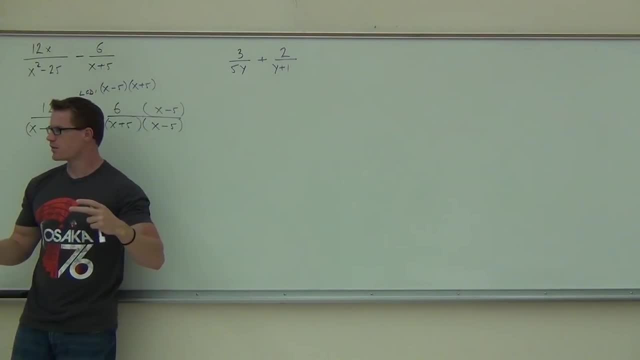 we're going to make one fraction out of it first, And I think I've shown you the reason why. right, It's basically because of that minus sign. If you distribute now and you get 6x minus 30, and you keep that minus 30 all the way. 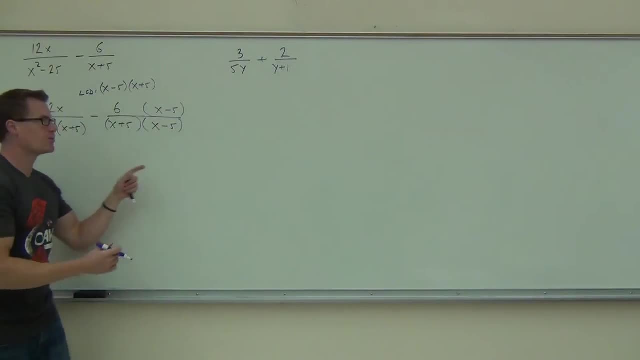 down, you're going to get the wrong answer. What's going to happen in this problem is that when we write this as one fraction, you're going to see this: We'll get the 12x, sure, we'll get the minus, and we'll get 6 times the quantity x minus 5.. 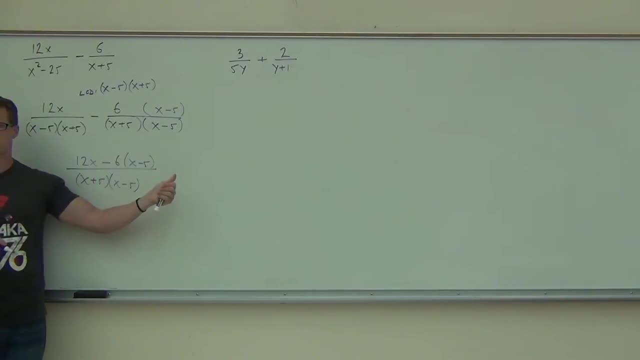 But when you look at that, do you notice that that minus has to distribute? We had that, I think, ending yesterday, where we really do want to write it as one fraction, because we change a fraction problem into just a combined like terms problem. 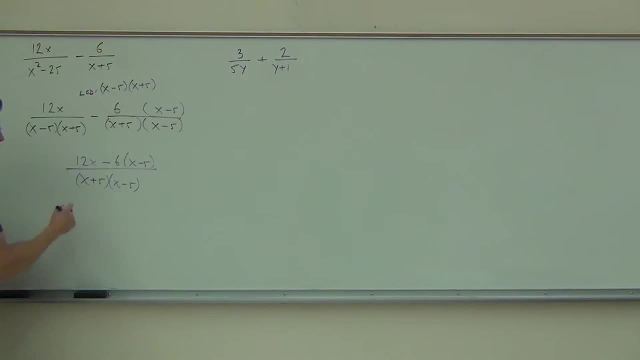 with a little bit of distribution. That makes things a little bit easier to see for us. So we'll keep going on this. We'll have, of course, 12x minus 6x and then plus 30.. Oh, x plus 5x minus 7.. 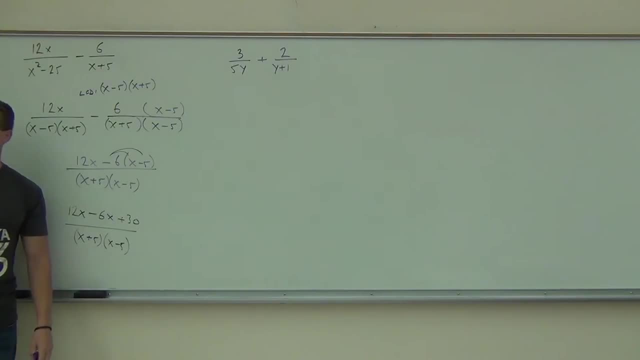 Did you make it that far? OK, what now? Great, so we can do that. We've got a couple of them. We certainly don't want- I hope you didn't do- this- but back on the last step. we certainly don't want to simplify. 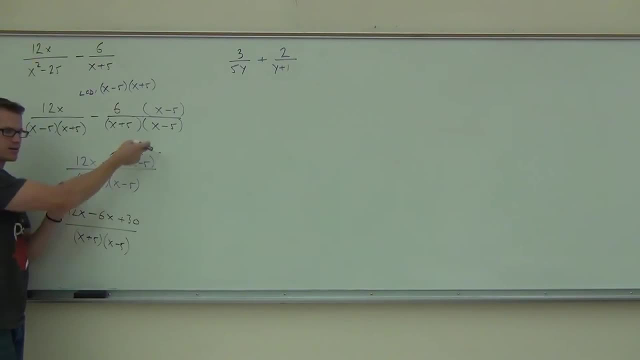 here. We talked about that last time. But why can't we simplify it here? Because the top simplifies the subtraction zone. Very good, Yeah, it's linked. This is like a term, It's like one big term. You can't cancel parts of terms. 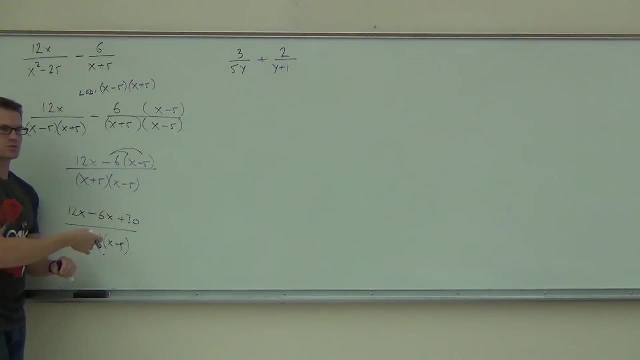 You can't simplify that Because of that minus right there. we cannot do that, So we'll combine our like terms here. We'll get 6x plus 30.. We'll get 6x minus 7.. We'll get 6x minus 7.. 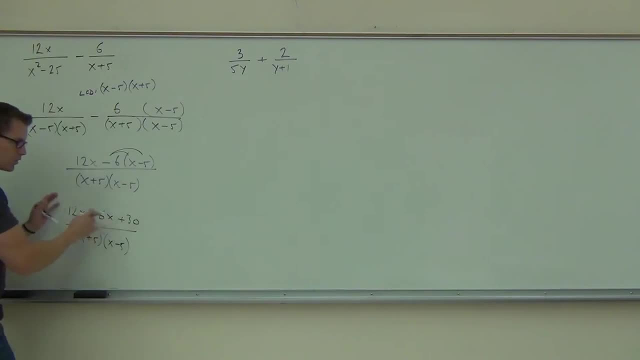 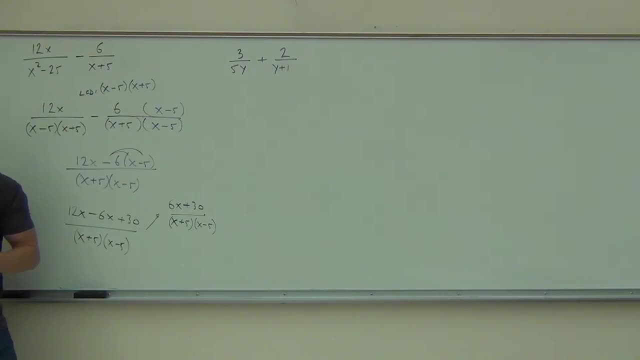 Is there anything else that we can do? What's that? Sure, Yeah, yeah, We can back to that thing. We can back to the 6 out. If we do, we get x plus 5 over x plus 7.. 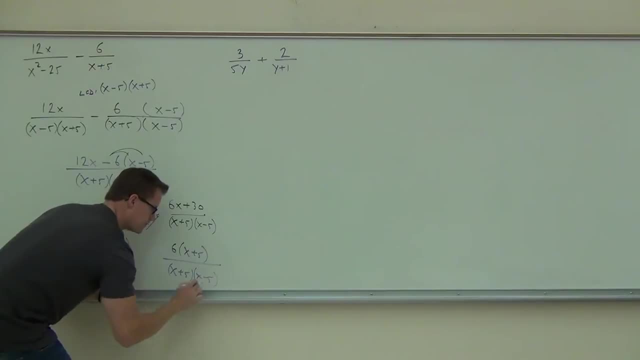 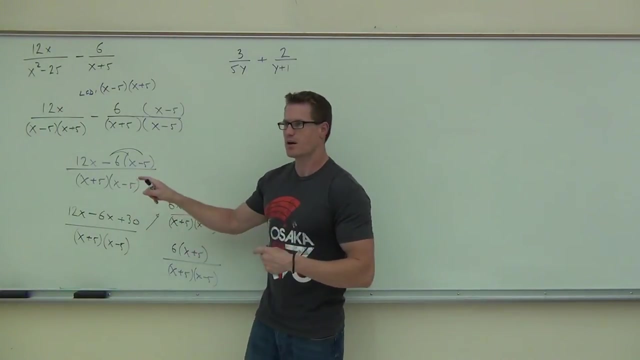 Yeah, x plus 5 times x minus 5.. Does anything simplify? Yes, It was worth our time to actually go and back to that thing, because x plus 5 is going to go away. Do you notice something on here? These problems, they can get you if you're not watching the sign, because check it out. 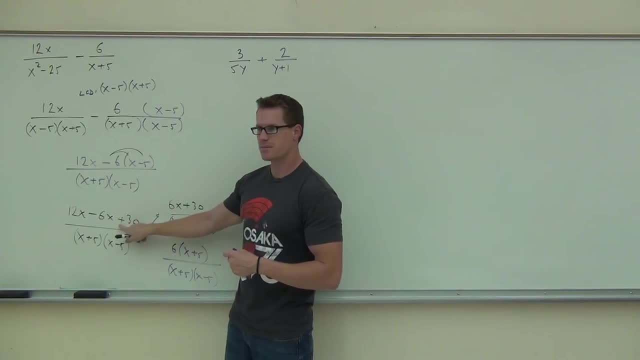 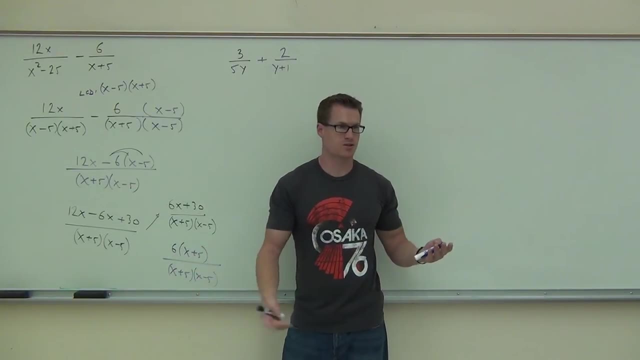 Even if you had not distributed the negative and you got minus 30, it's going to look like you can factor it. if that's a minus 30, right, and you're going to simplify the wrong thing, It's still going to look like you can simplify it, so you're going to probably think you're. 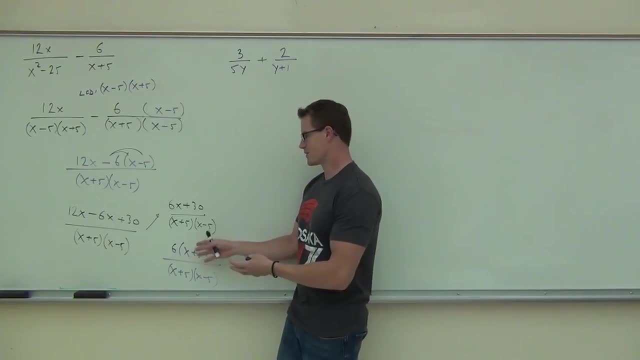 doing it right. Maybe you're real careful on this stuff. that way, you get down to here and you're not like, oh yeah, I'm crossing out the x minus 5s. No, we're not. We're crossing out x plus 5s. 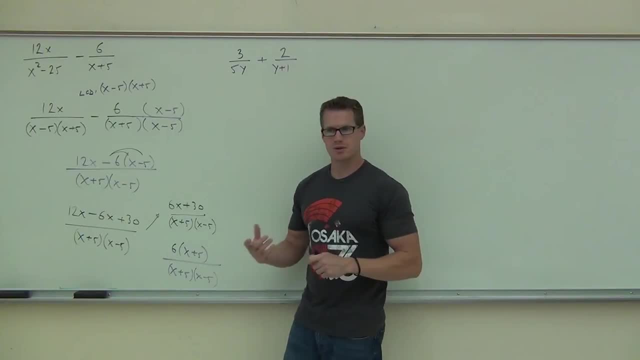 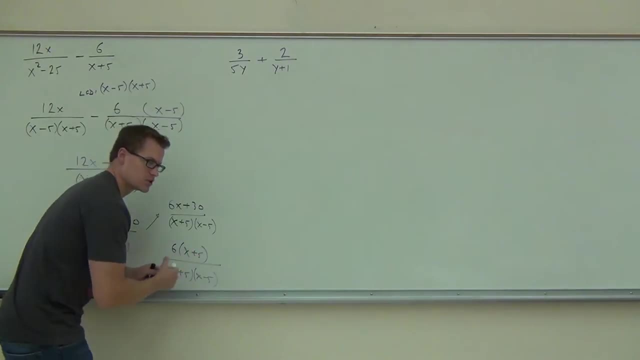 Also one more thing. I've noticed this on some of your homework. Some people have been doing this where there's like an x plus 5 and pretend that's an x plus 5.. Let's pretend for a second I'm going to change it back, but let's pretend this was an x plus 5.. 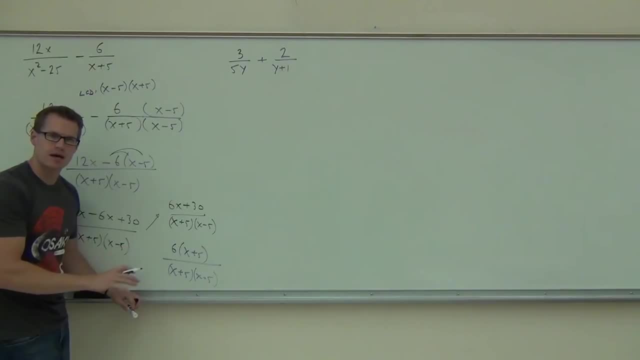 I have some people who are crossing out all three of these and we can't do that. It matches up one for one. If you get rid of this one, You can't also get rid of the other one. Are you with me on that? 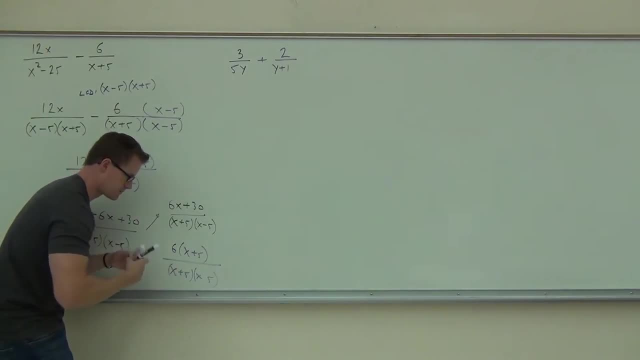 It's one for one on this, So let me change it back to the minus. That's what it's supposed to be. And then, of course, we can simplify the x plus 5s, and our answer is 6 over x minus 5.. 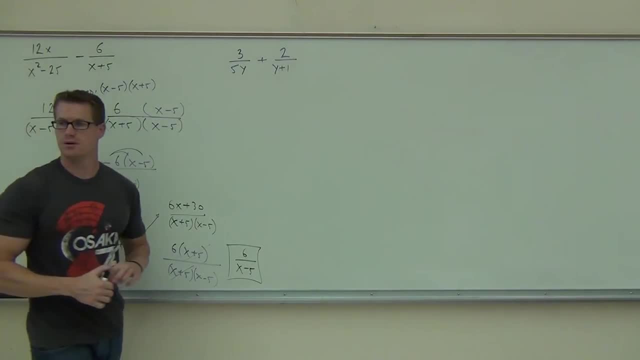 Did you make it down that far? How many of you made it to? let's all raise our hands, because I know you all did the problem right. Everybody raise your hand. That means we're good. Raise your hand, Okay, good. 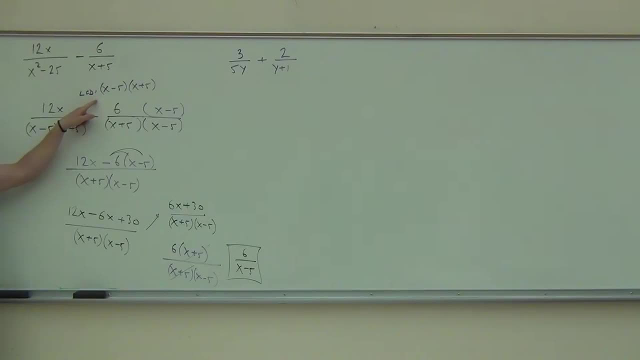 How many of you made? can you give me a hand? Good Here, Drop your hands if you didn't Here. Good Here, Okay, Here, Okay. That's the minus sign. Watch your minus sign Here And all the way down. 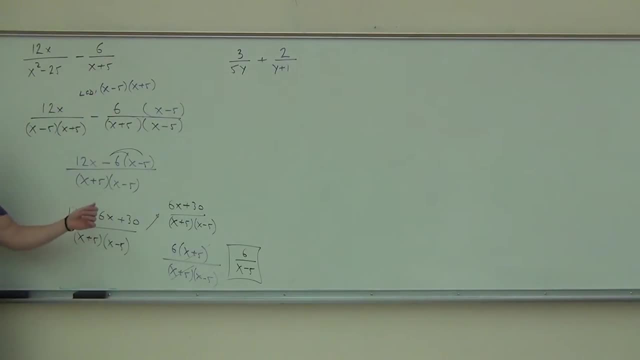 Good for you, Okay. So I saw a lot of people drop their hands between this step and this step. If you are one of those people, then that's where you're making a mistake, right? You need to know that. You need to kind of understand where you're making a mistake. 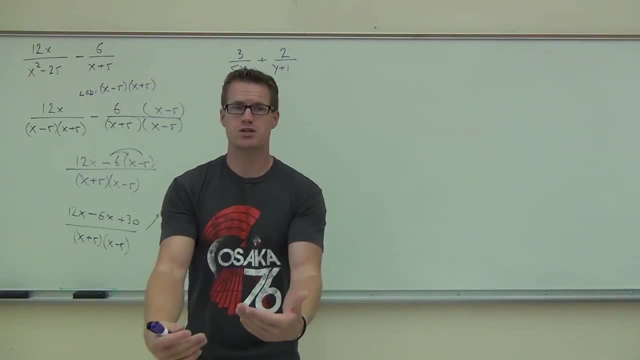 It's not all about me just telling you what to do. It's about you understanding where those problems are coming in. That way you can fix them. You're in college now and I'm not supposed to hold your hand. You're supposed to kind of realize what's going on. 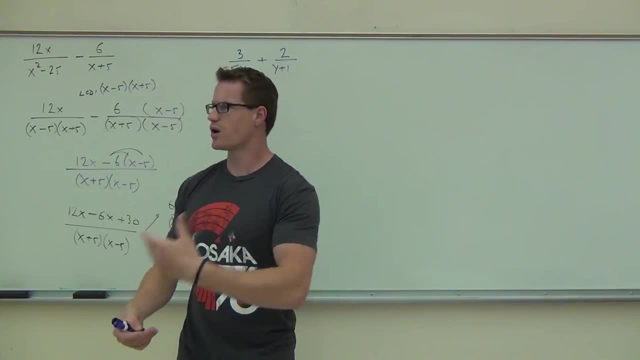 Okay. So if that's, you notice next time that your distribution is kind of going wrong and keep a special eye on that Question. Never mind, I just thought I was wondering what happened to the 12 X, but then I realized it went to a positive. 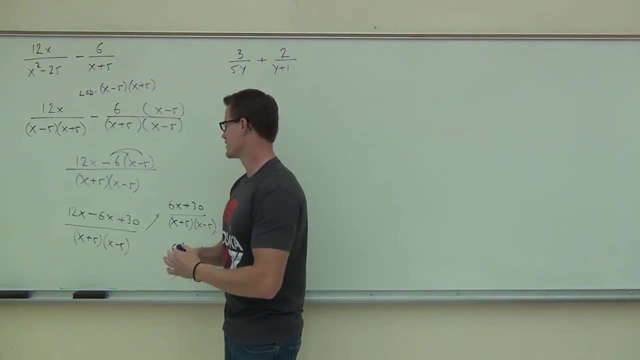 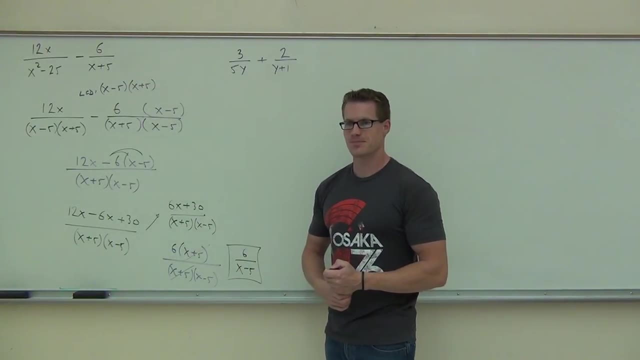 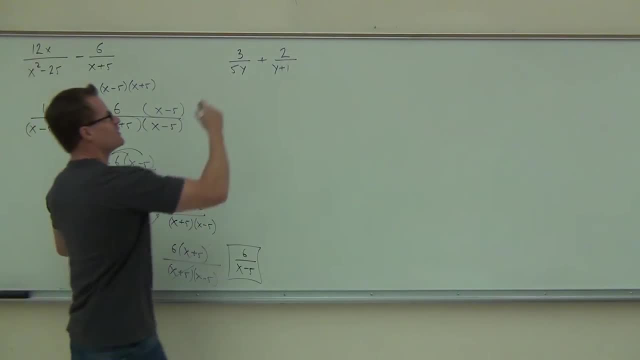 I just want a fresh memory on what to do. Firstly question: is our LCD 5Y plus one? No, we can't do that. The 5Y has to be a factor. right now, The 5Y is a term. 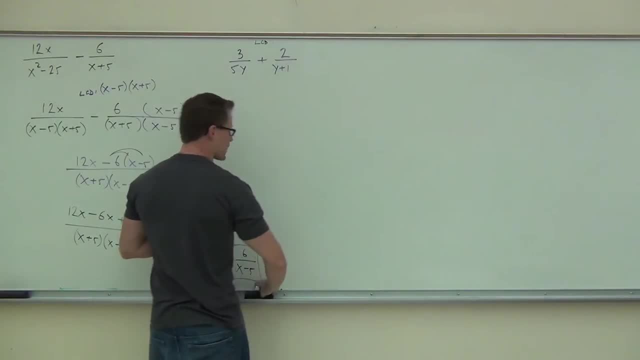 That doesn't work for us, So our LCD. in this case we do need the 5Y and we also need the Y plus one. those both have to be there. Then we check and we go: do we have the 5y? 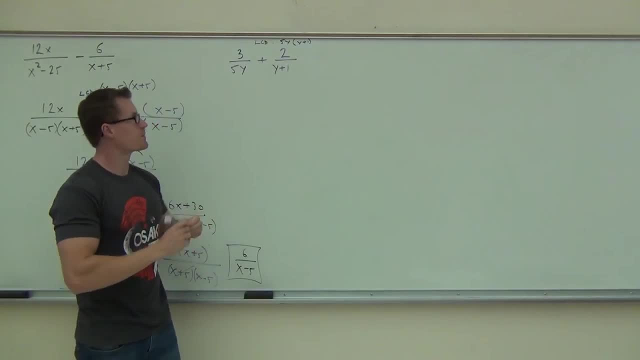 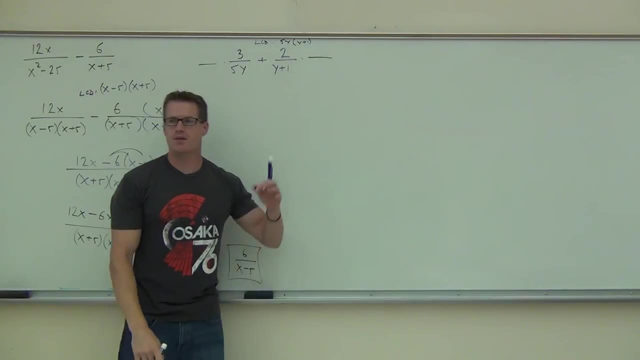 Yeah, Do we have the y plus 1?? Yeah, That's our LCD in this case. After that, we're going to multiply both sides because we need some extra stuff over here. We don't have everything we need On the left-hand side. what do I multiply by everybody? 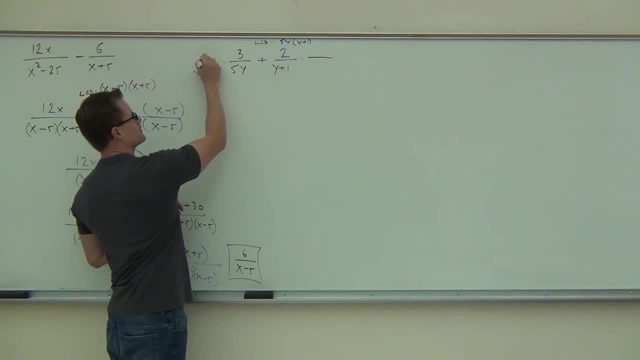 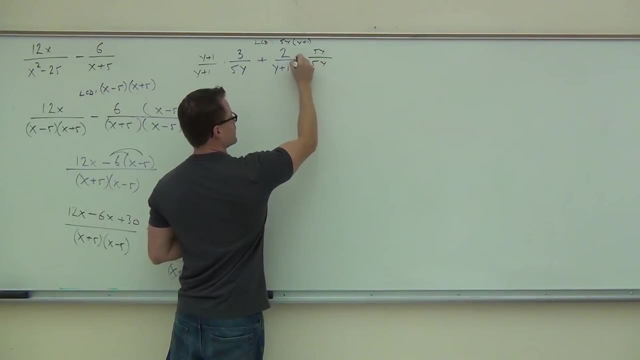 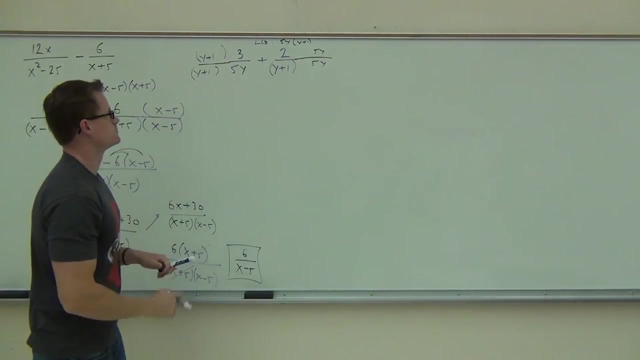 One. That wasn't everybody, but I'll take it, Okay. And on the right-hand side, what are we multiplying by One? Good, Again, we extend our fractions. We put our parentheses where we need them On the numerator we're going to get. 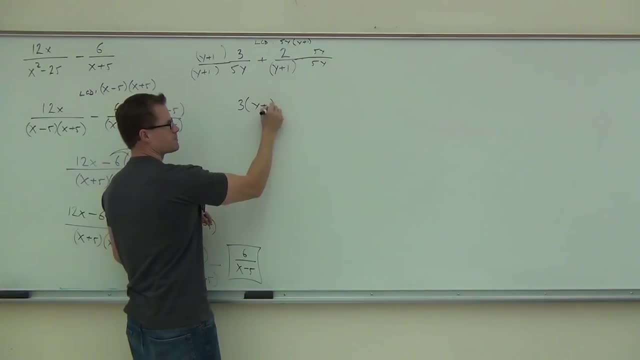 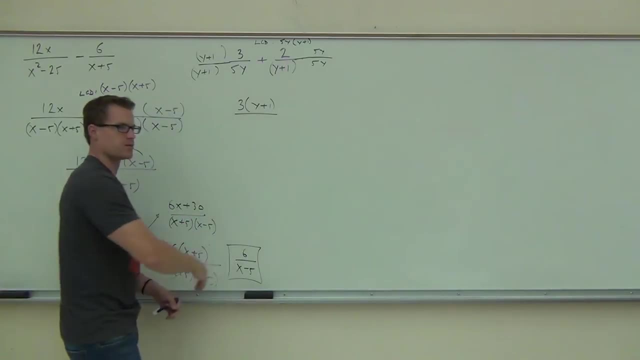 I'm going to write the 3 first 3y plus 1.. On the denominator: am I going to distribute the denominators, folks? No, No, never distribute denominators. My goodness, we're trying to simplify them, right. 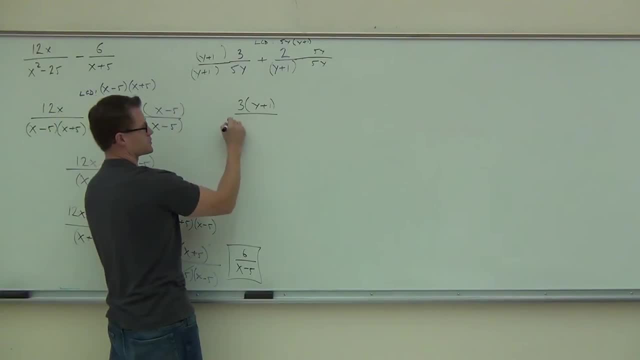 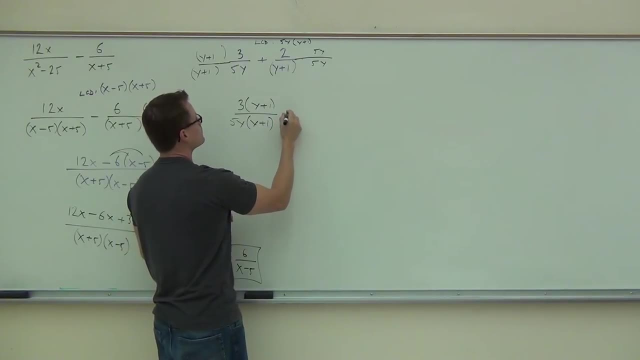 So leave those denominators the way they are. All I'm going to do is write the 5y first. And what's on the second part of our numerator, 2 times 5y? Sure, I'm just going to write 10y in this case. 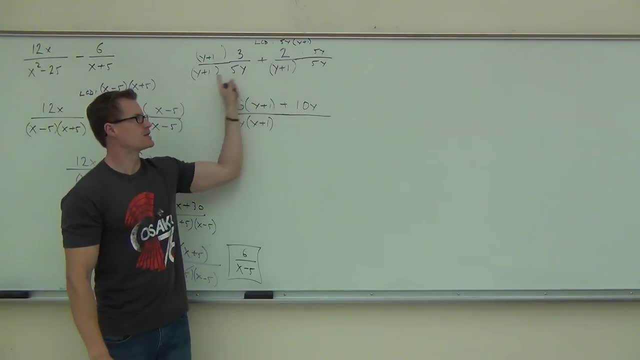 Since we had our common denominator, we have our 5y times y plus 1.. That's our common denominator. here We've combined to make one fraction. We have the 3 first. That's the only difference. We have 10y. 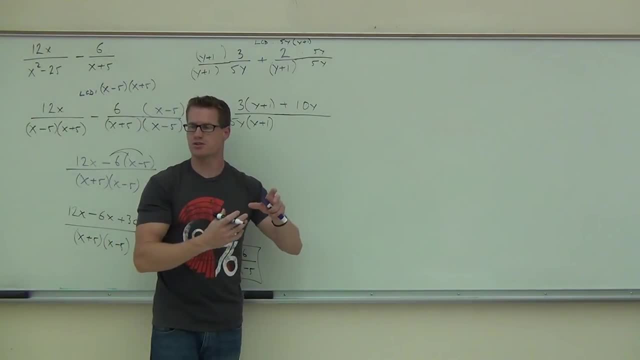 So I've skipped the intermediate step of reorganizing both my fractions. Not sure if you're still okay with this. Okay, One question I have for you. Can I cross out the y plus 1s? No, No, No. 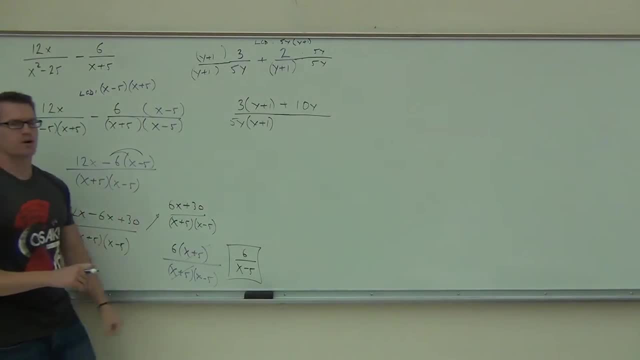 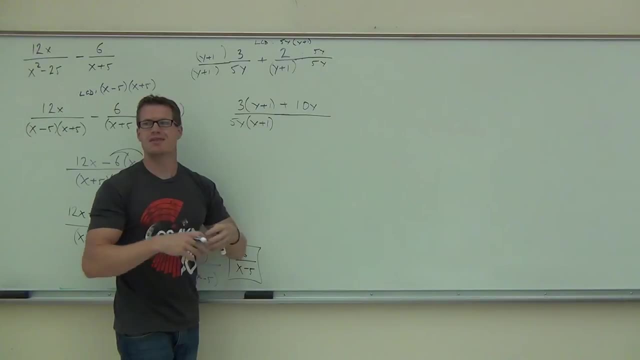 Definitely not. That's the same question as this: Can I cross out the x minus 5s? No, It's connected by that plus. I can't do anything about it. One thing I can do is distribute the numerator and combine like terms and then see if I can factor. 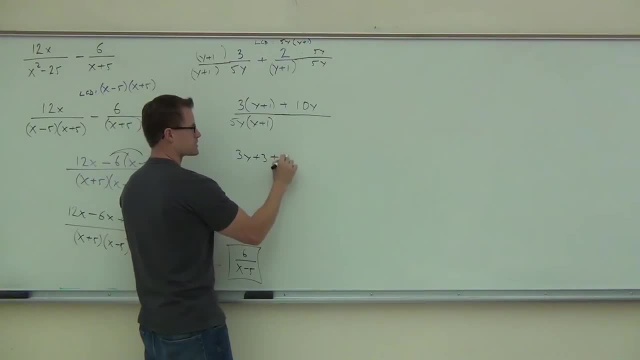 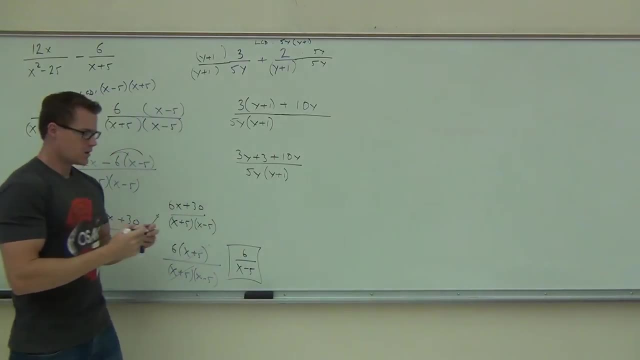 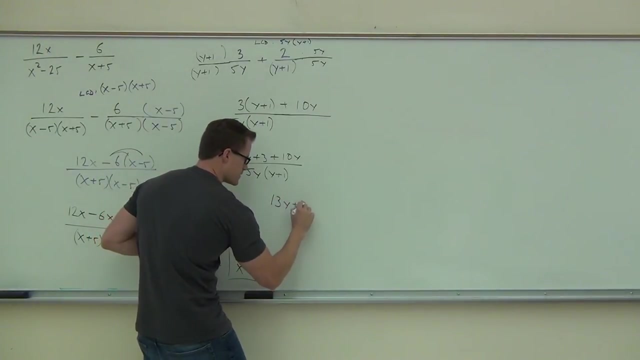 So we will do that. We'll get 3y plus 3 plus 10y over 5y y plus 1.. When we combine some like terms, we're going to get 13y plus 3.. Now, 13y plus 3, can you factor that? 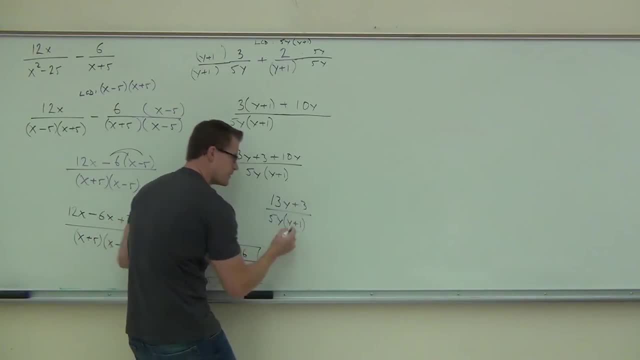 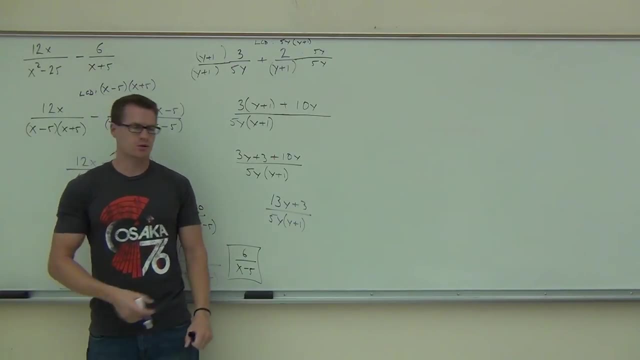 No, No, No, Then that's your answer. That's all you can do with it. If you can't factor the numerator after you combine the terms, you're done. You're done. Don't distribute the denominator. Don't start canceling out y's. 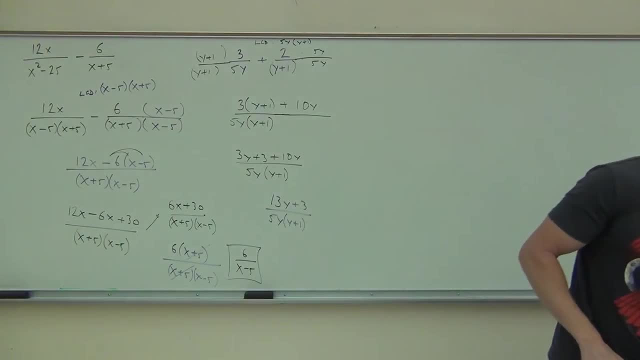 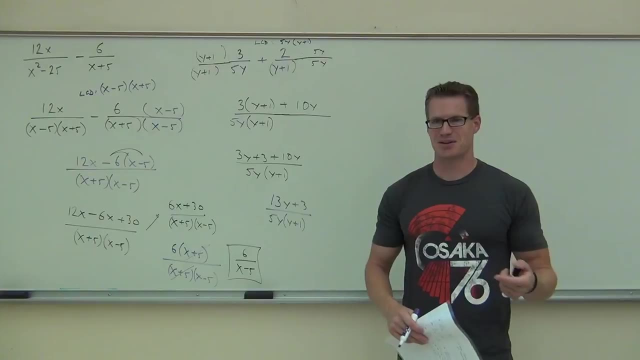 You're done on that problem. Okay, Now we're almost done with adding subtracting rational expressions. There are a few more examples. Then we'll get on into solving, which is it's kind of fun. I think you're going to like solving. 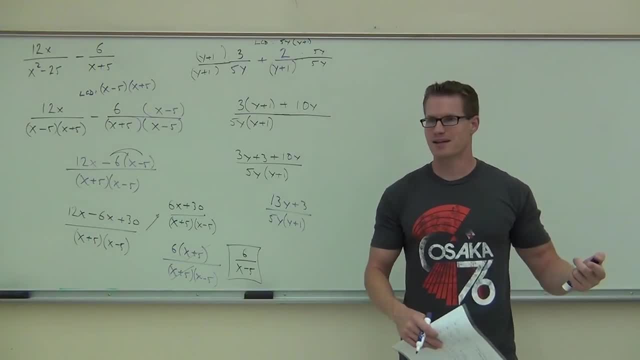 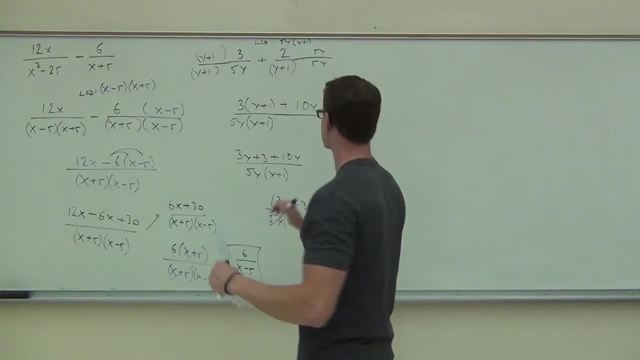 You'll like it more than this, And if you like this, that means you're going to love solving right, Obviously. There is one thing I do want to show you, though. It's two different problems. Neither of them are very hard. 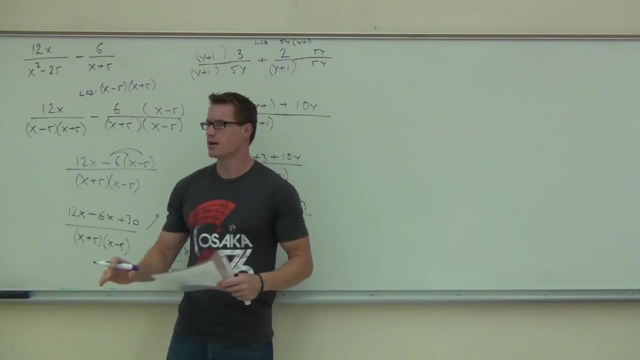 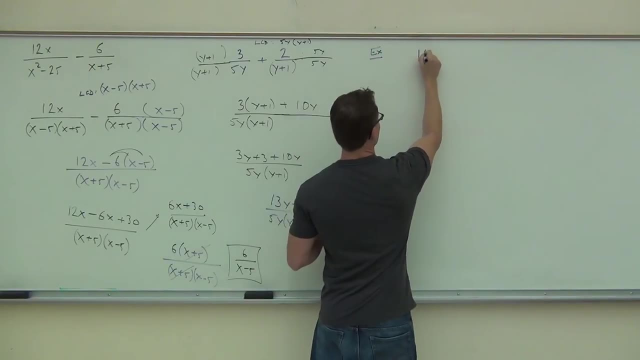 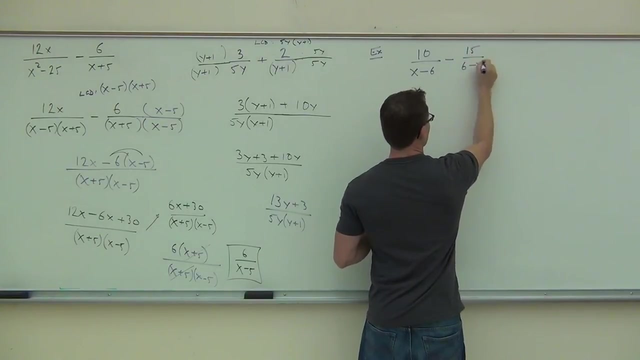 Well, if you remember what I tell you, neither of them are very hard. Okay, I just want to make sure that you see them at least once. I kind of previewed this example Last time in class, or the time before that one or the other. 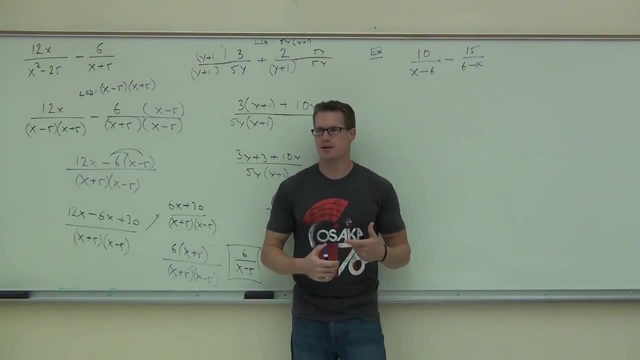 that we don't exactly have an LCD here, but it's very, very close. Do you see that You could do this one of two ways? Okay, You could find your LCD the same way you did over here and have LCD is x minus 6 and 6 minus x. 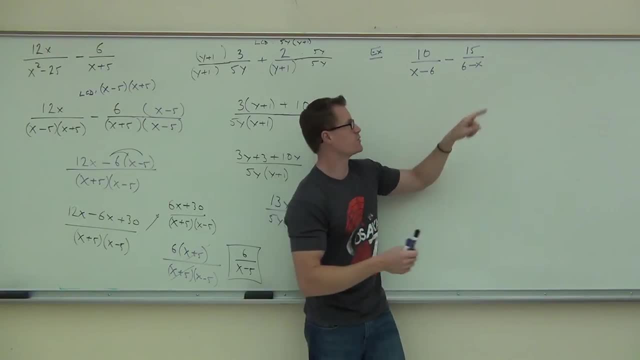 Do you see what I'm talking about? You could do that. It would take you a lot more work because you have to multiply here. Do you see what I'm talking about? X minus 6 over here? You have to multiply here 6 minus x. However. 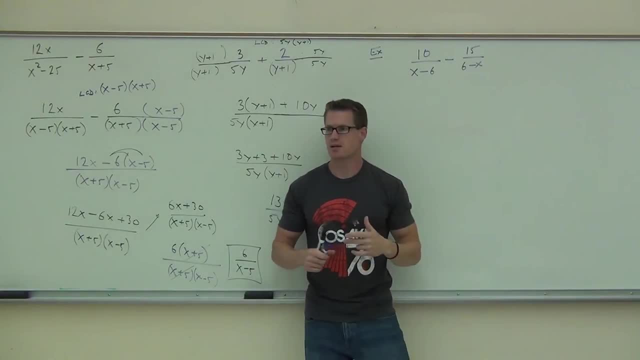 if you do a little more work, you're going to get x minus x. If you do a little manipulation and do what I told you about keeping the largest power of x, if you do that, then you don't even need to find your LCD. 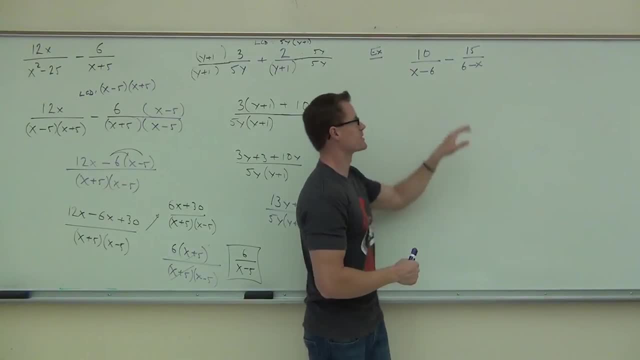 It already really has one Specifically. what I'm talking about is not here. This is great, It's what we want. But here, notice how the x has that minus in front of it. If we factor appropriately, we can get rid of that. 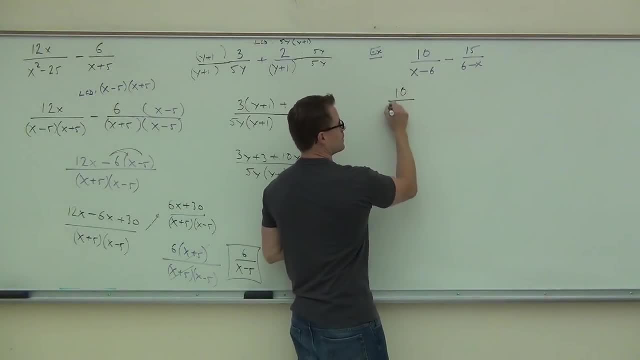 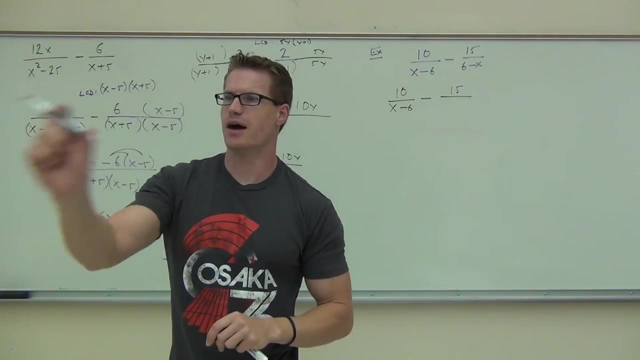 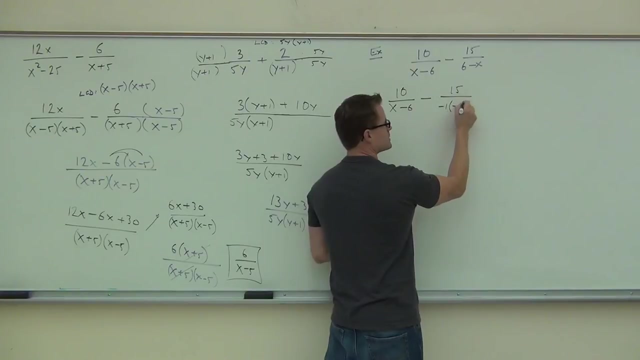 So I'm going to leave the 10 over x minus 6, but this 15 over 6 minus x. I'm going to factor a negative out of the denominator. If I do that, it changes from positive 6 to negative 6. 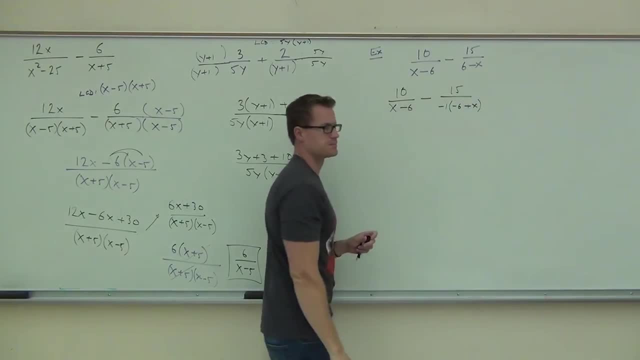 and negative x to positive or plus x. I'm going to show you step by step on this so you really see what's going on. Are you okay with that? I've done that several times in class, so hopefully this is not a big deal. 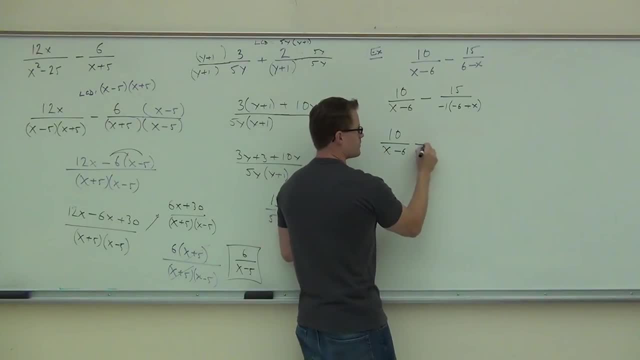 If we keep going, we have 10 over x minus 6 minus 15 over negative, 1 times 10 over x minus 6.. I'm going to switch those around. I've done that a couple times. also, Instead of negative x plus- I'm sorry- negative 6 plus x. 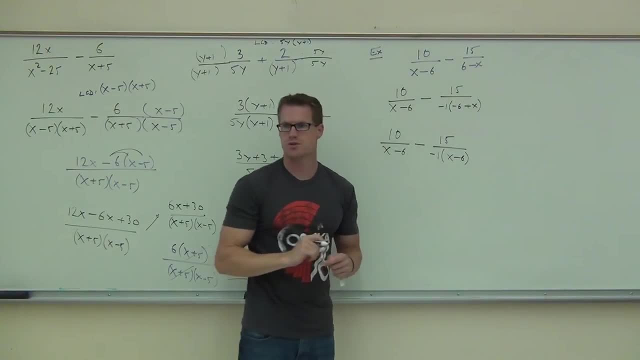 I'm going to get x minus 6.. We've seen that before too. right Now, here's the cool part. Just like you have an example like this: 7 minus negative 2.. What's 7 minus negative 2 really mean? 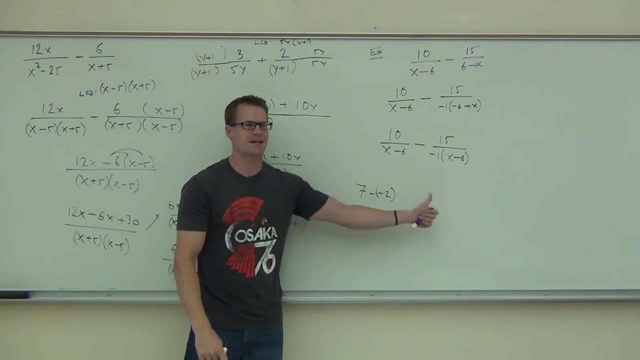 7 plus 2.. Good, because you're really taking away a debt, or you're adding like, if I took away your debt, it's like I'm giving you money, right, I'm taking away, subtracting a negative, I'm actually adding to it, so this becomes 7 plus 2.. 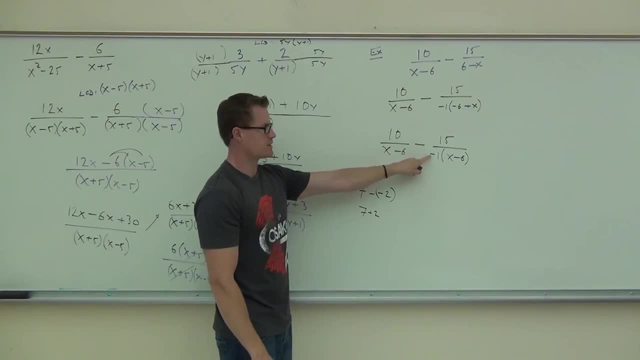 Same thing happens here. You are subtracting a negative. This negative doesn't have to necessarily be on the denominator. It could be here or in the middle, or on the top, It doesn't really matter. So we have subtracted a negative. 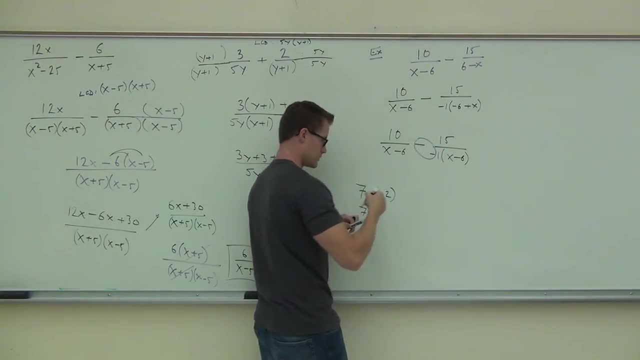 These two signs are going to become what Good Plus. that's where the plus is going to come in. that makes a plus 15 over x minus 6. Where that negative went, it combined with the minus sign to make that plus. 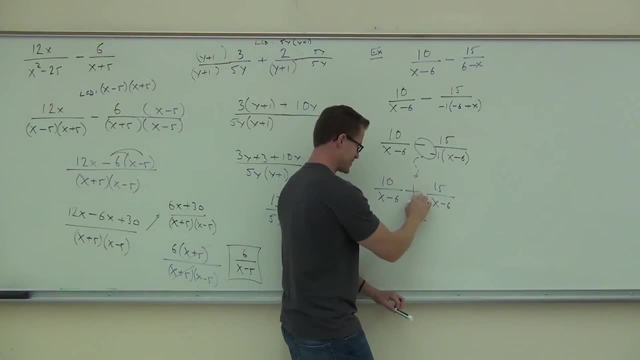 I actually kind of overdrew the plus a little bit. I want to make sure you saw that. Okay, All right, And now, look, we've got a common denominator. You don't even need to do any more work than that. No, distributing on the numerators, nothing like that. 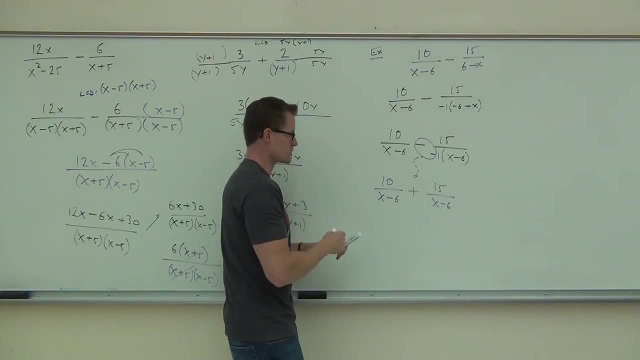 because we still have single numbers. It's kind of nice. It makes it a little bit easier. So when we combine this, we'll get the 10 plus 15 over x minus 6. When we add those together we get our 25x minus 6, and we're done as far as we can go. 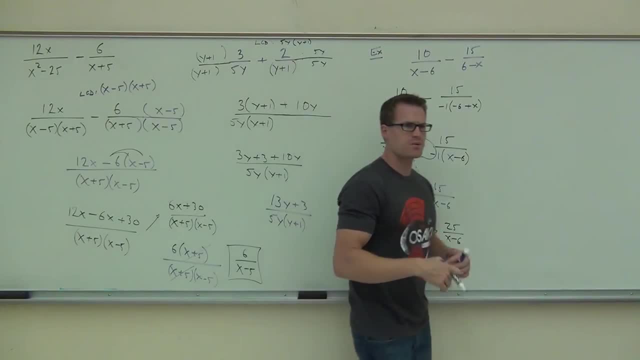 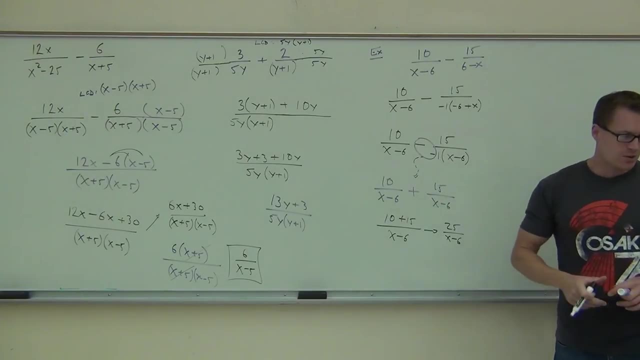 No need to simplify. You're good, Are you with me on this one Kind of nice right? So remember about factoring that negative in. Sometimes it can save you a lot of work. Okay, Last type of example. then we'll just do a couple practice problems. 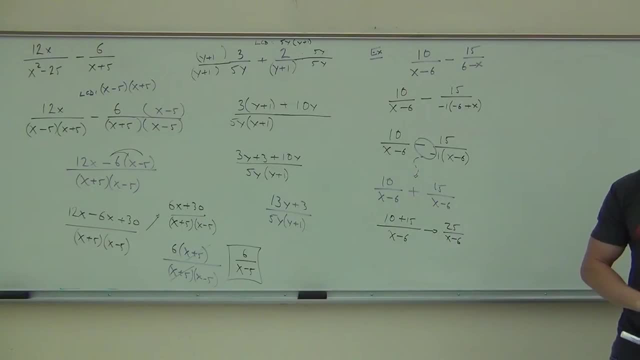 The only thing I was thinking about is the negative 1 that we have to factor out That way. we have to times whatever we factor out on the right side to the left side, So we don't times the 10 times the negative 1?. 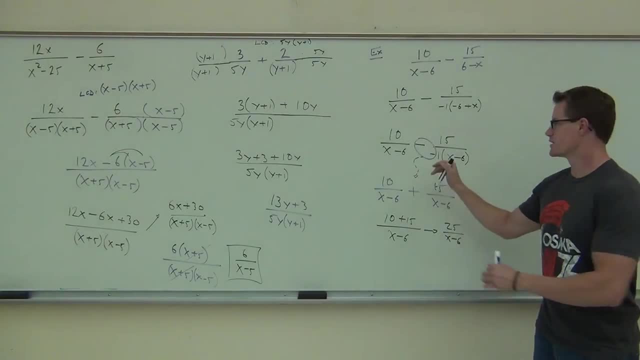 No, You're just working on this fraction. right now. It's actually kind of like you're ignoring this part of it. Okay, You're just working on this one itself, all right? Okay, You really aren't multiplying anything by negative 1.. 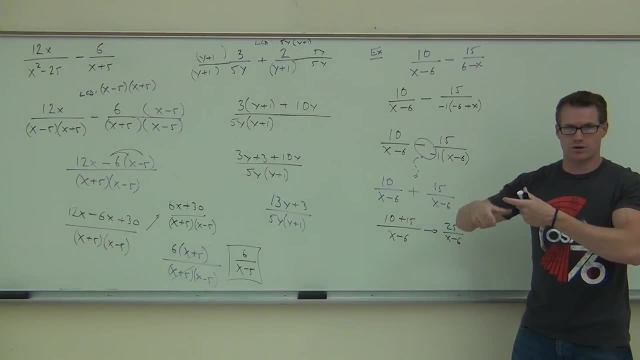 What you're doing is you're actually dividing by negative 1 on one fraction. I can see how you get confused, because before, when we had equations, we multiplied every fraction by the same thing. right? We don't have equations here. We're not going through and multiplying everything. 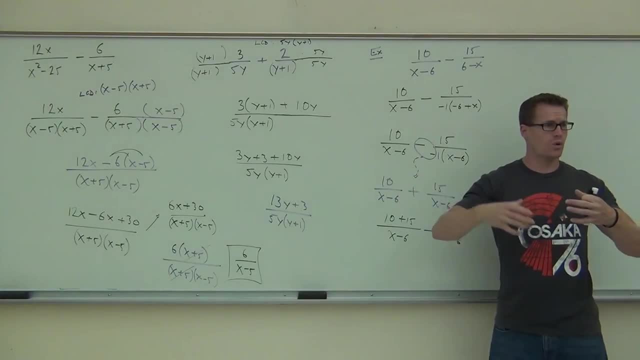 We can't do that because we don't have the two sides, And so what we're doing is just manipulating one fraction in order to change the side. That's what we're doing here. It's a good question. Okay, Let's look at one more. 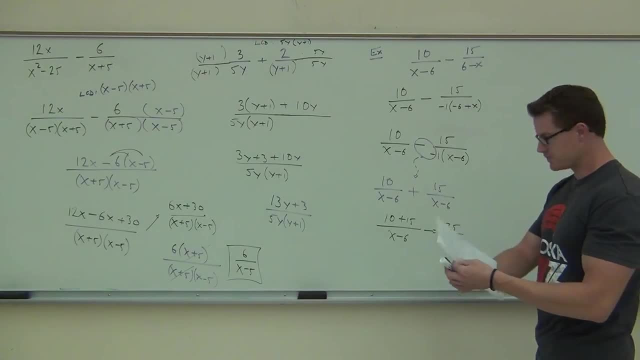 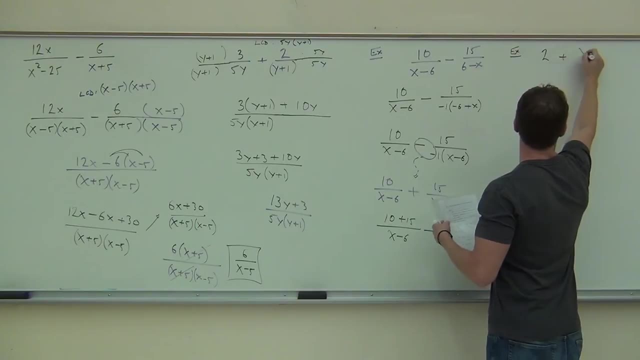 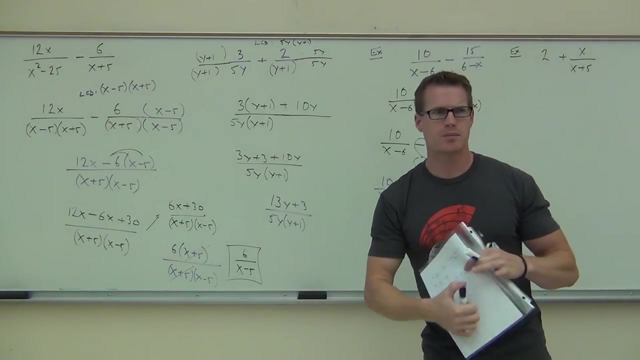 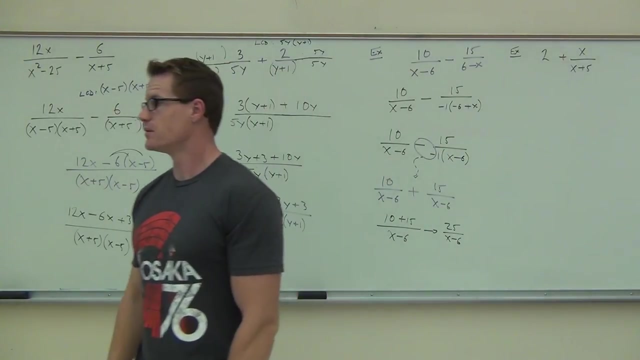 We'll do a few examples, like I said, and then we'll move on to our next section. Is it possible to add just a whole number to a fraction like that? What do you think? What now? Put a 1 there. 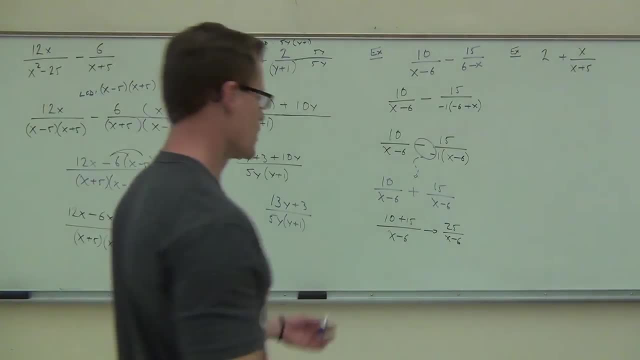 That's right, Great, So we can change a whole number to a fraction. We can change a whole number to a fraction itself by putting a 1 underneath it. All right, So I can't just do this, right, I can't just go: oh, this is x plus 2 over, x plus 5.. 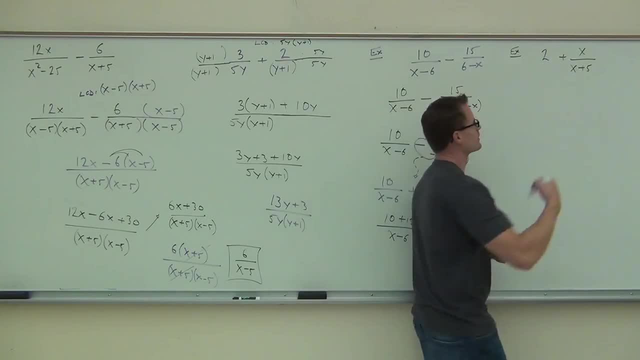 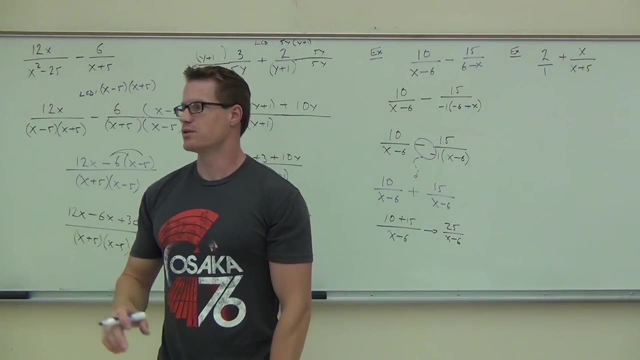 Can I do that? That'd be easy, That'd be nice, right, if we could do that. What the 2 really means is: yeah, that's 2 over 1.. So now we can go back into the same process. 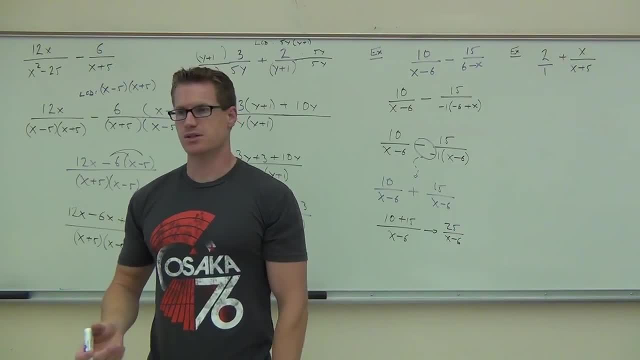 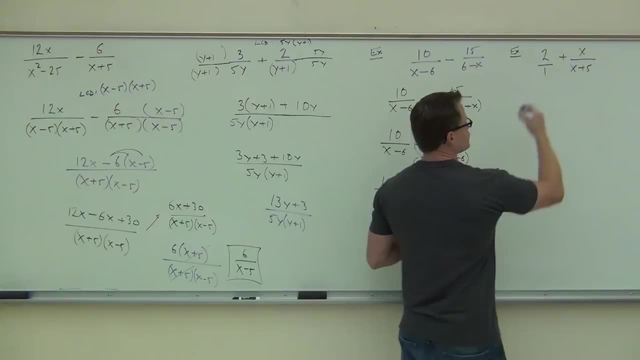 Can you find a common denominator with this? What is our LCD here? It's nice, right, When the other one's a 1, the LCD is a parent. It's just the other denominator. So our LCD is The 1, doesn't really count. 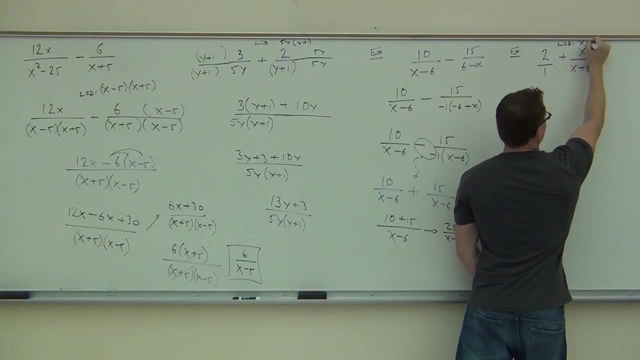 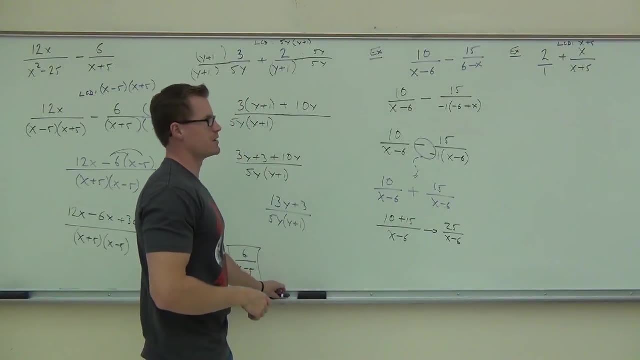 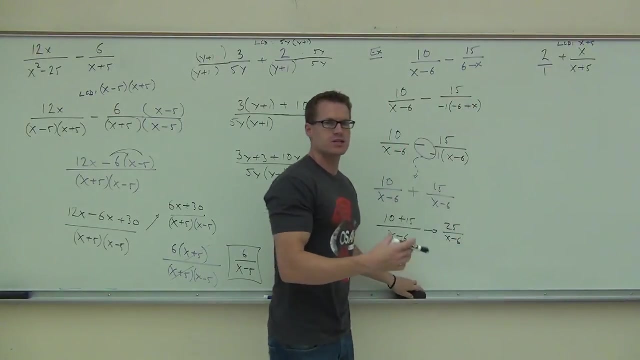 We don't include the 2.. That's a new winner. We do x plus 5.. Which fraction or fractions do I need to multiply? The left, the right or both? The left, Good, yeah, The right already has our LCD. 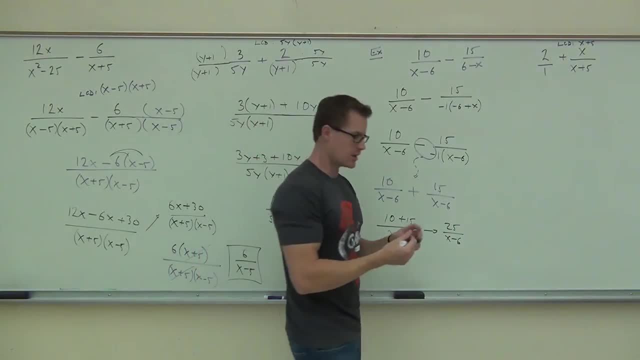 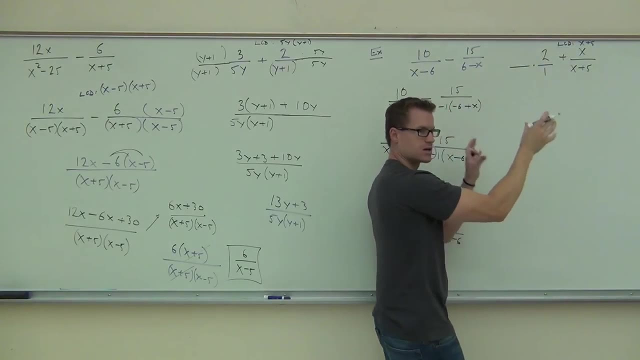 That's actually how we got it. So we don't need to multiply the right fraction by anything. The left fraction we will And we know we're going to multiply it by whatever it takes to multiply it. So we're going to make the LCD come up in that fraction. 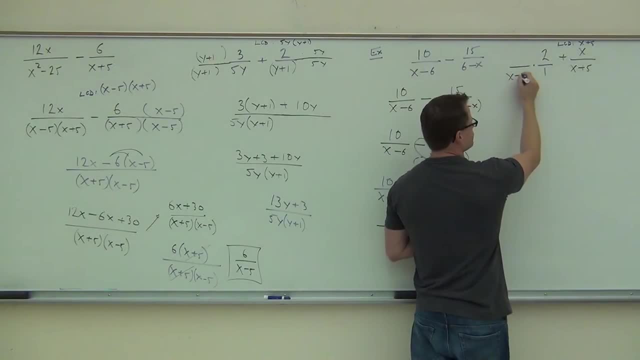 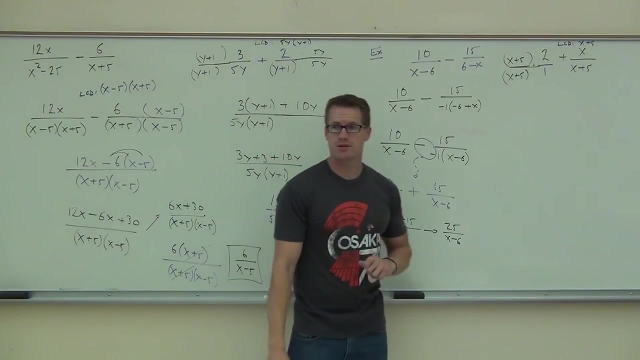 So if I have a 1 here, I'm missing the entire x plus 5.. Of course, we'll extend our line. We'll put some parentheses where we need them. Do I have an LCD now? Yes, Yeah, I have x plus 5 and x plus 5.. 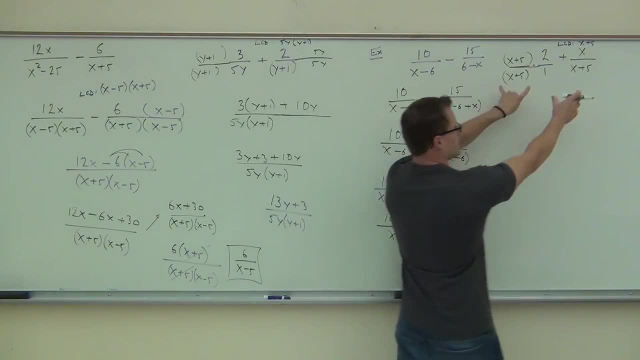 We get to now make 1 fraction out of this. So because my I have my LCD, I can write 1 fraction. What does my LCD give? x plus x. So that goes here And on my numerator I'm going to write my first numerator, just. 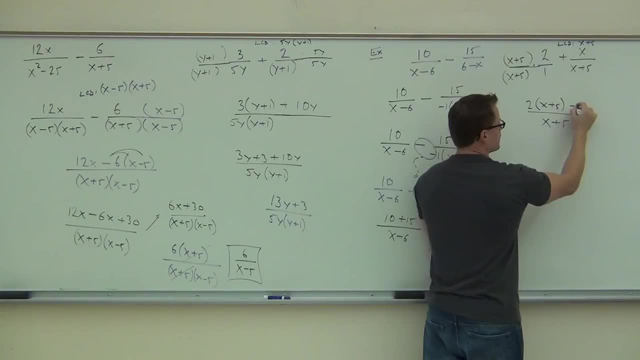 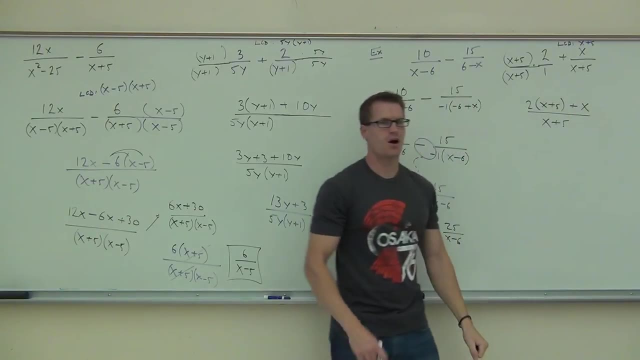 with the 2 first plus my second numerator. So first numerator plus second numerator, It's all over the x plus 5 that I already had on the denominator. What do I do now? Do I simplify now or do I distribute now? Distribute and copy. 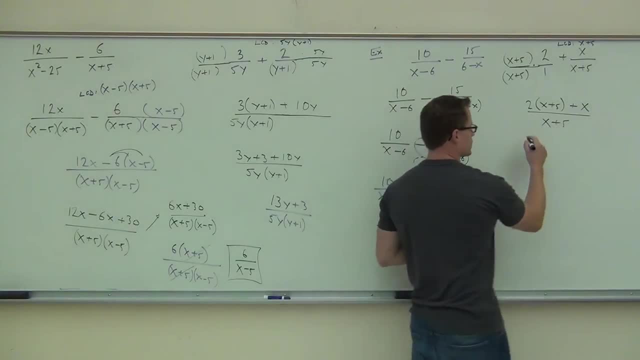 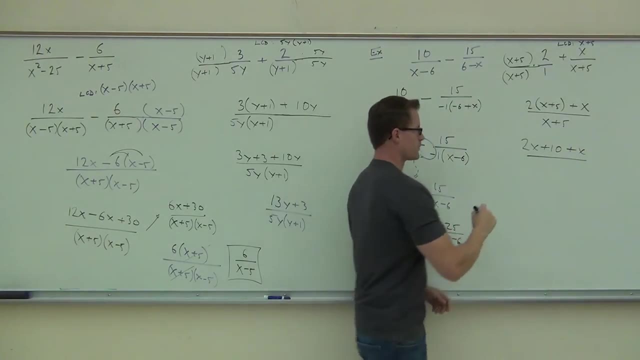 Numerator. Yeah, I can't. I can't cross anything out. yet I need to distribute first 2x plus 10 plus x over x plus 5.. Our last step in this case is just combine like turners, because it's not going to factor. 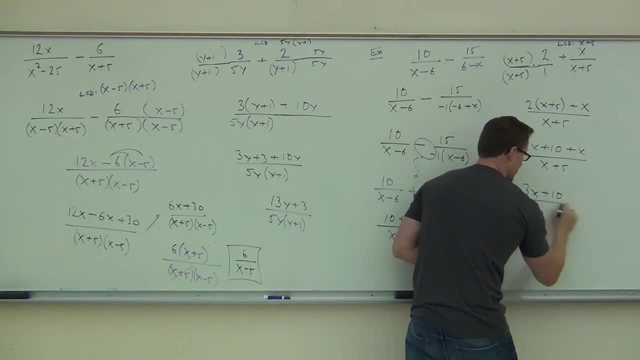 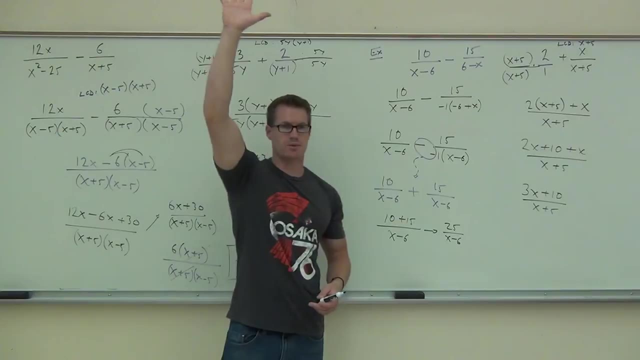 We're going to get 3x plus 10 x plus 5.. And that's as good as we can do. How many people feel okay with what we've talked about so far today? Okay, Okay. Would you like to try one of these on your own? 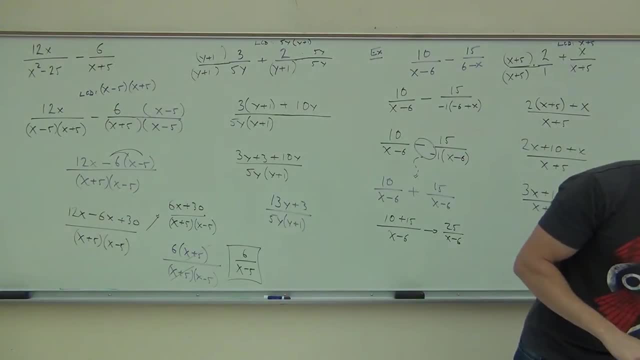 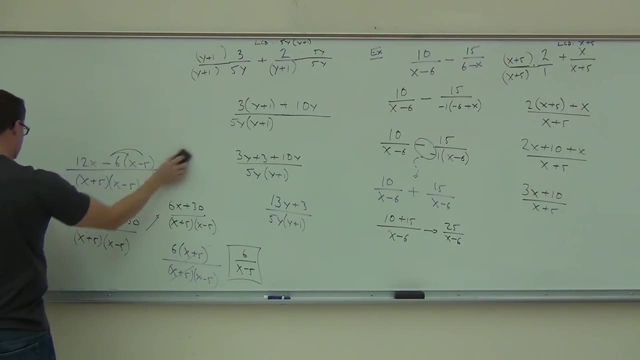 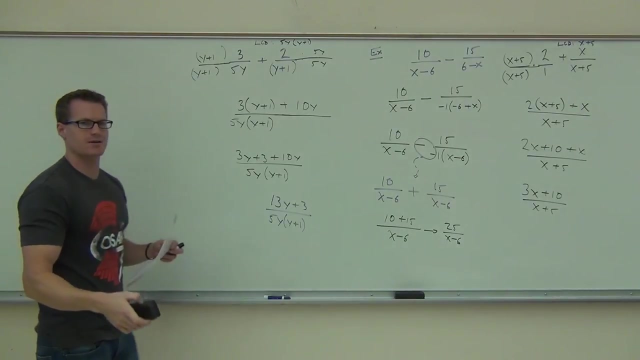 Yes, Okay, We'll do one like that one And then I'll write up a few more. Actually, you know what? Maybe we'll do one more together and then I'll give you a couple to do on your own. that way you have some more time for that. 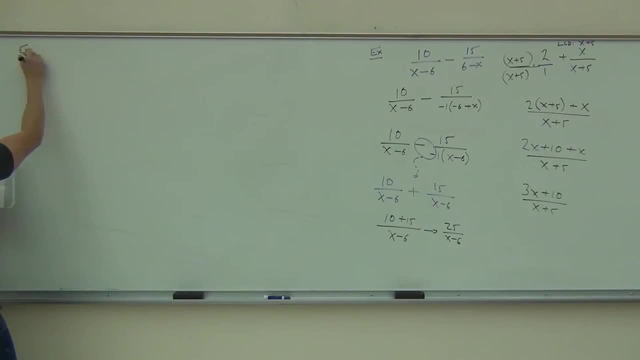 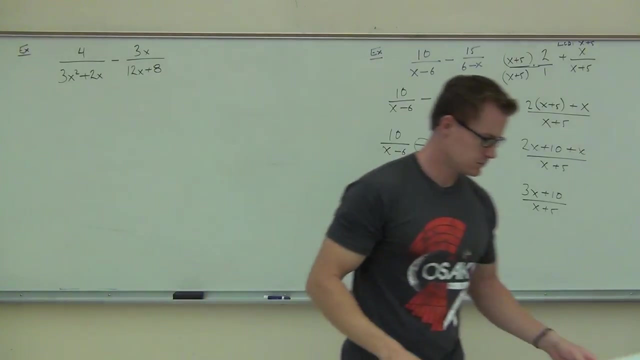 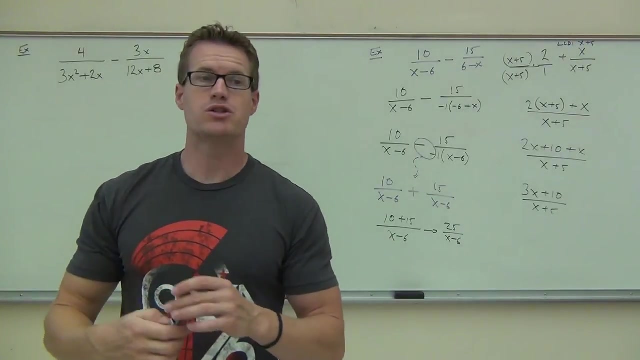 There we go. Okay, We're going to do this completely together on this one. We're going to Step-by-step through this, but I want you to tell me the steps and then we'll work on it together. What's the first thing that I might want to do if I'm trying? 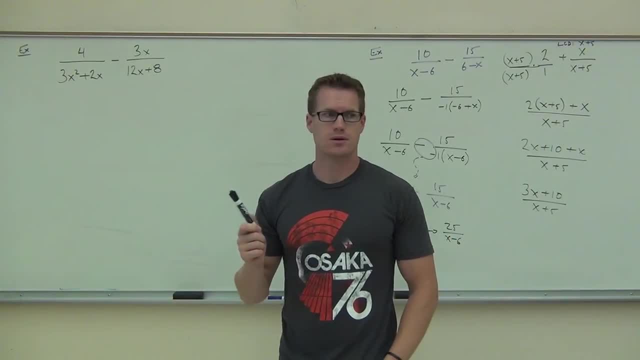 to subtract these two rational expressions. What's the first thing you do every time you get a rational expression? You well, yeah, but before you do that every time, you factor Every single time. Yeah, you guys are right, You're going to factor every single time. 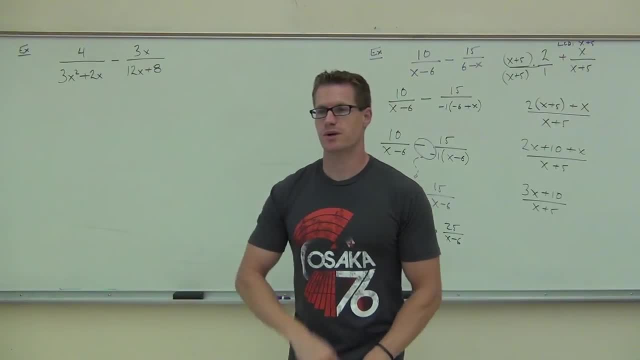 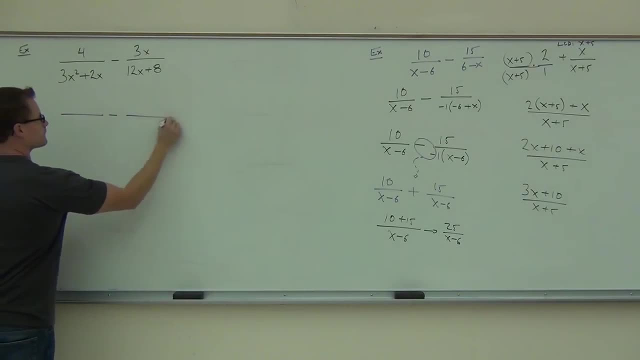 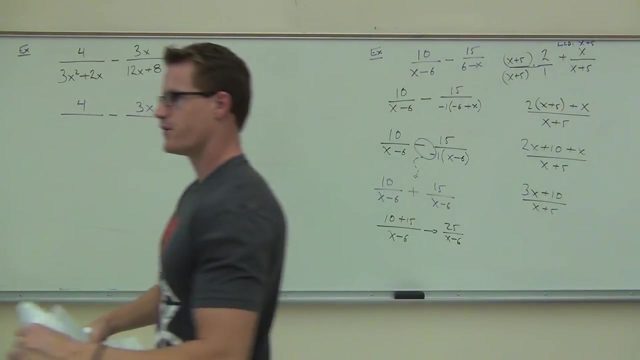 At least the denominators. So let's go ahead. I want you to factor right now. We're not talking about the numerators, Those will stay the same. We're talking about the denominators, So factor. Let's start with the even fraction, the one on the right. 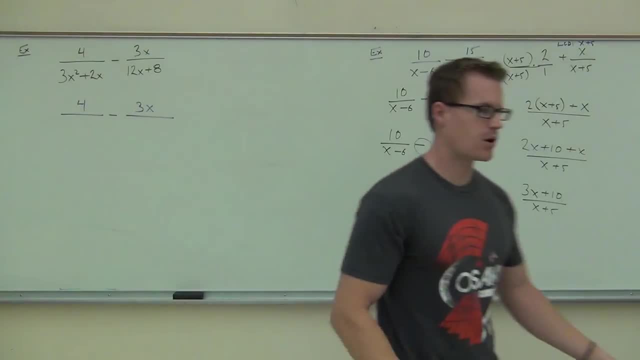 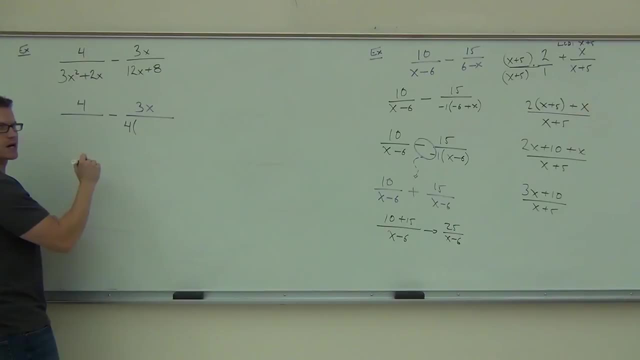 Ladies and gentlemen, what factors out of the fraction, the denominator, How many are on the right-hand side? Four, Four, Okay, very good. So we're going to get four times what folks? Three, Three times, Perfect. 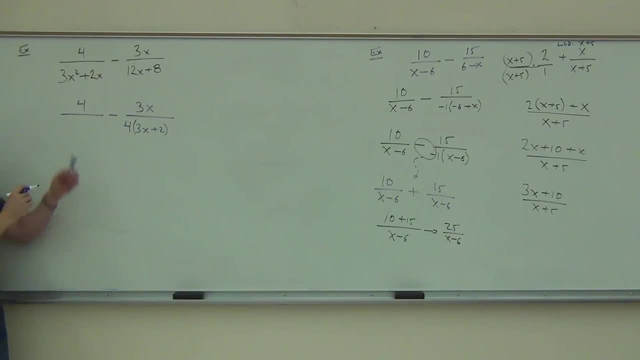 Did you get that? Yes, Sweet. How about the left one? Do I need a diamond problem for that? No, It doesn't even have three terms. It's certainly not a difference of squares. It has two terms, Not a difference of squares. 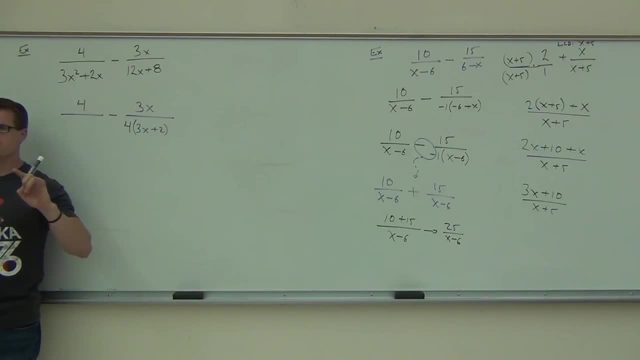 It has a plus in the middle. It's not a sum of cubes or anything like that. It's not that hard actually If you're thinking those ideas like: oh, we're forgetting one thing, We're forgetting about the GCF. 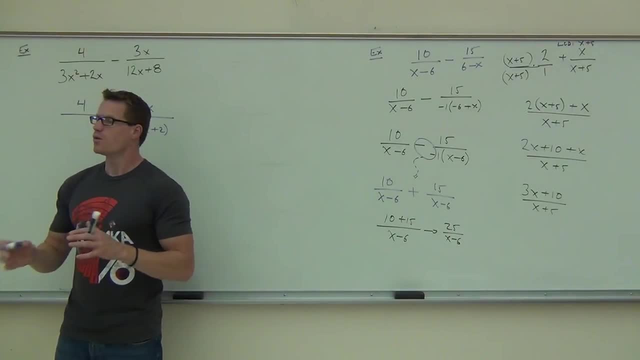 Remember the greatest common factor that we're supposed to look for every single time. What is our greatest common factor here? X. So don't forget about the X. We can factor that The X is in common to both. We get 3X plus 2.. 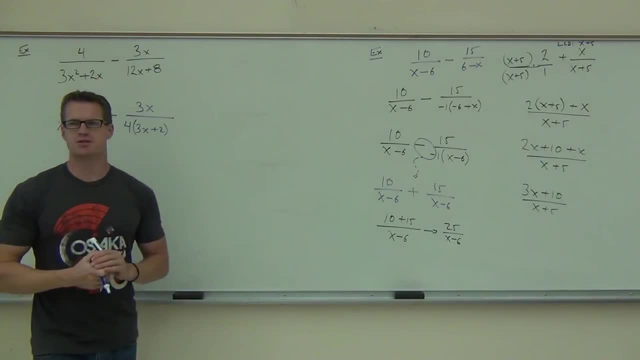 Did you make it that far? What's the next thing we do after you factor? You tell me LCD. Let's go ahead and find our LCD for me. Okay, so write LCD right up top. Look at our denominators. We're going to take the largest power of each different factor. 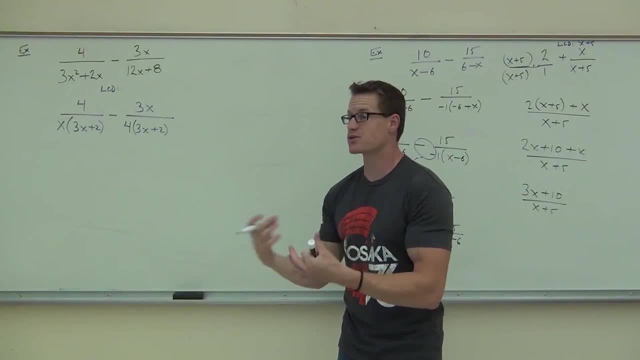 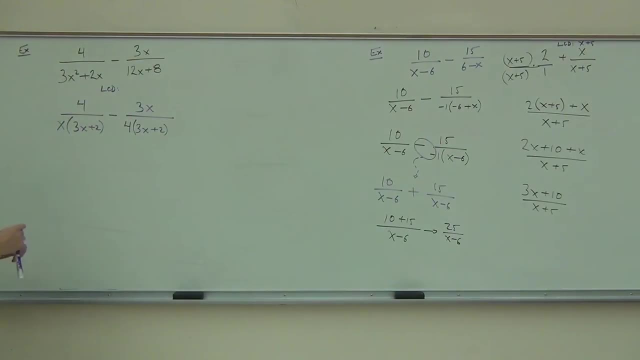 So write that down right now if you haven't already. This should not be the hard part. The factoring is actually in the next step. It's kind of a hard part. This is a nice and easy part. LCD just lists out all the factors. 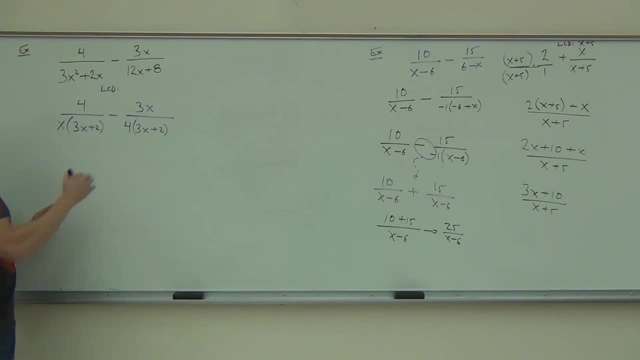 Tell me one factor. I'm going to have 3X plus 2.. Okay, You all saw the 3X plus 2, right? Do I need it squared or not? No, No, it's in different factors. It's fine. 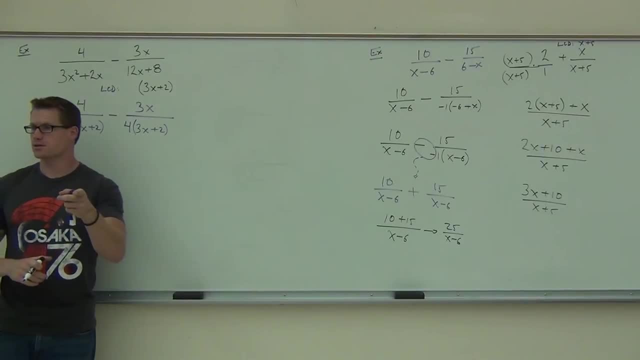 We just need it once. What else? 4. 4. Anything else? X. So what I'm going to write is 4X, like that. I've got the X Check. I've got the 3X plus 2.. 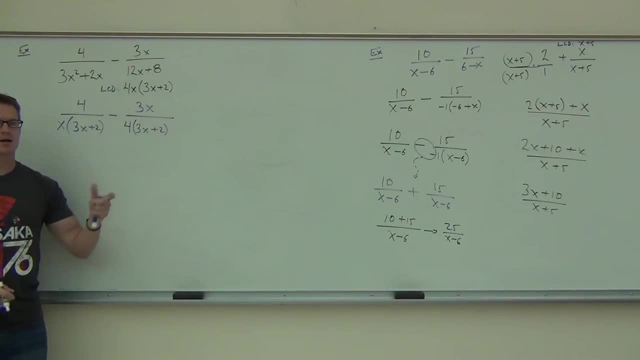 Yep, I've got the 4.. Yes, I have 3X plus 2.. I've already got that, So that is my LCD. Did you find that on your own Good? Okay, Now we use that to make some equivalent rational expressions. 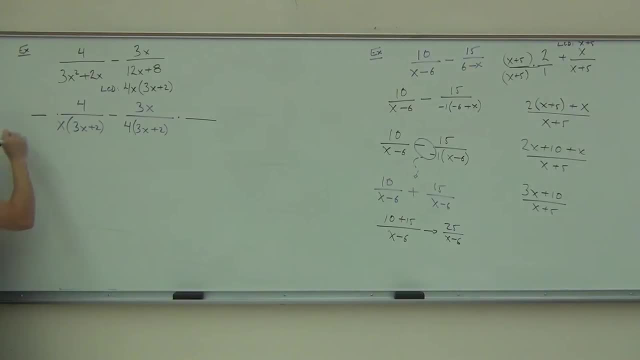 That's our next step. So basically, we're just multiplying by whatever we don't have in the LCD. So go ahead and write that down, Okay. So go ahead and write that down on your paper, if you haven't done that already. Okay. What gets multiplied on the left fraction? ladies and gentlemen? 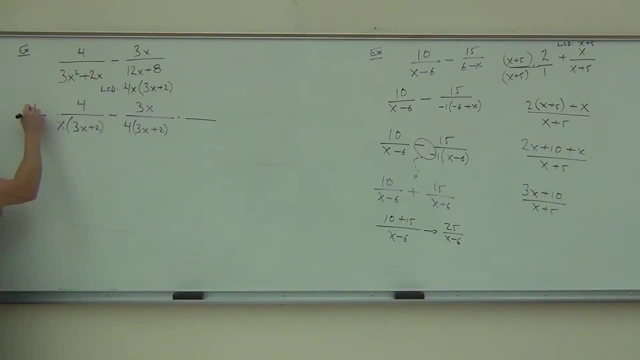 4. 4.. Oh, that's not too bad, right, Just a little 4.. We can do that. How about the white, The white On the white? we have this fraction: What gets multiplied over here, X. 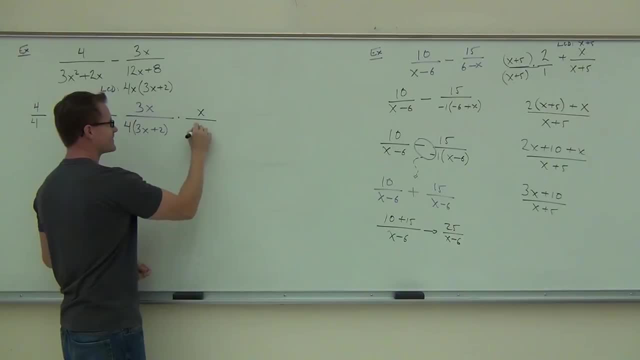 X. I'm going to stop saying right anymore. Did you find this also? Yes, Okay, So now that we have what's missing, we can see this: We're going to have our 4X and we have our 3X plus 2.. 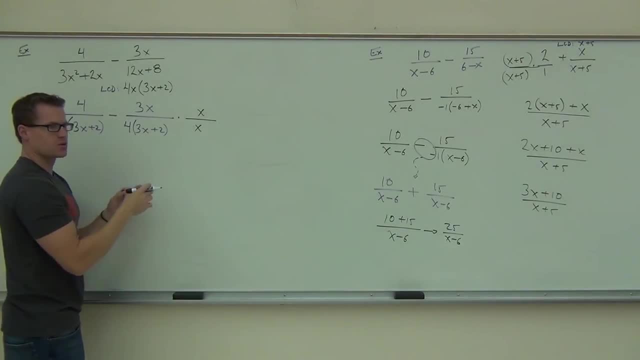 That's the same. We have our 4 and our X and our 3X plus 2.. Let's go ahead and let's multiply these fractions. We're going to get 16 over 4X, 3X plus 2 minus. what did we get on this fraction? 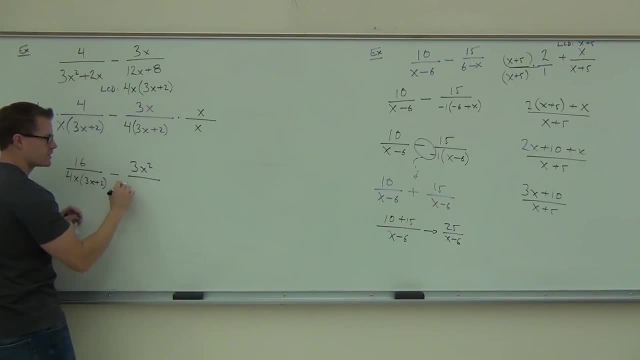 3X squared- Oh good, Don't forget about the X squared- And we get 16 over 4X. 3X plus 2 minus. what did we get on this fraction 4X? I'm just writing this in the appropriate order for us: 3X plus 2.. 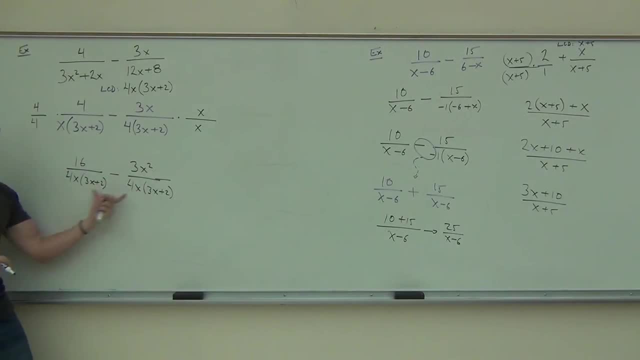 And you can see that we've done it right, because we have our LCD in both spots and it's the same as the one we had up top. That's great. That's exactly what we want. Now, what do we do? Write one fraction. 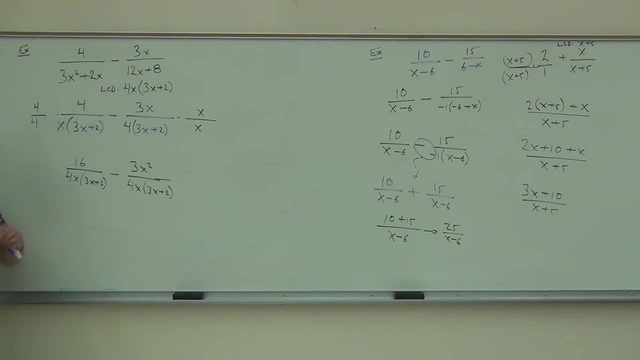 Great One fraction. We've already got this set up right. We have the same denominators. That's fantastic. 16 minus 3X squared is just the first numerator minus the next numerator, 4X, 3X plus 2 minus. what did we get on this fraction? 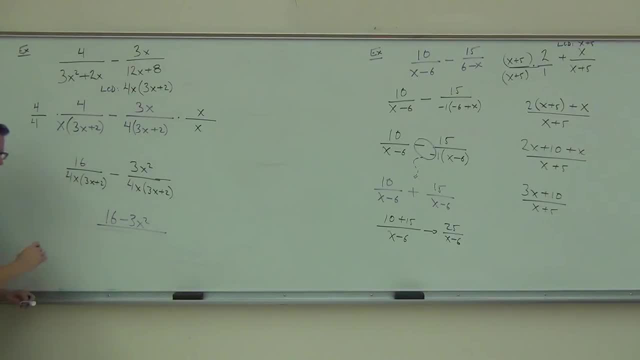 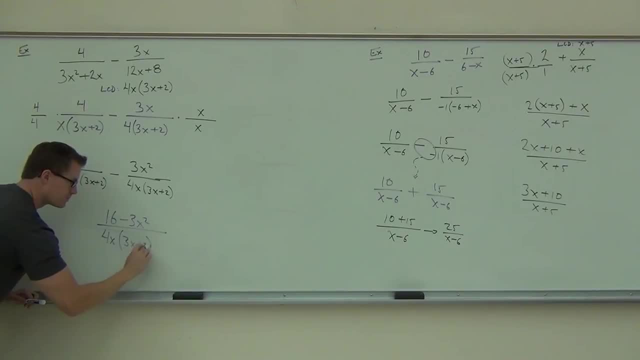 3X plus 2 minus. what did we get on this fraction 3X plus 2.. 4X 3X plus 2 minus. is this the first numerator minus the next numerator, 4X 3X plus 2.. 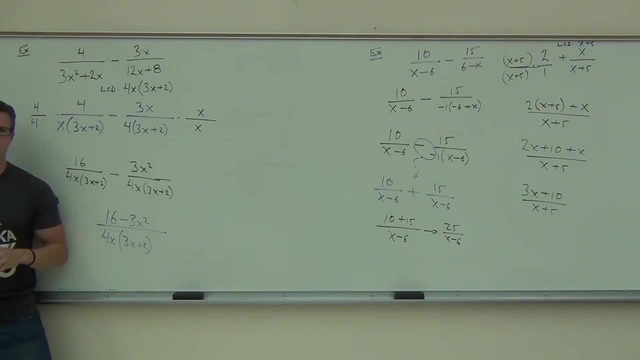 What are you going to try to do now? What would you try to do at this point? Try to factor Now. even though it's minus, even though that's a square, that number is not a square. This is not a difference of squares. 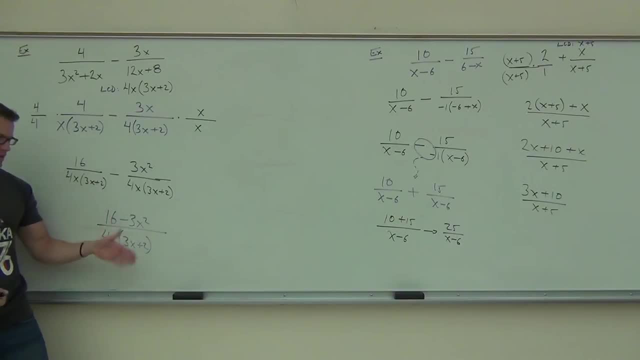 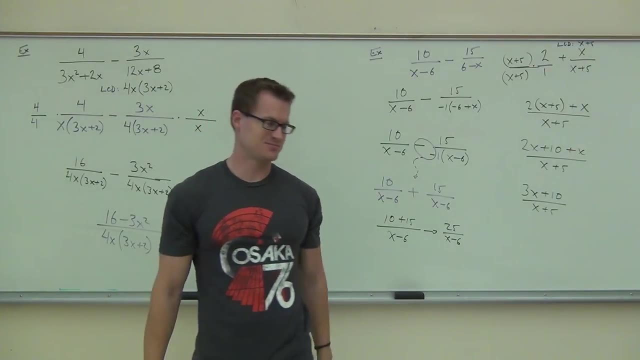 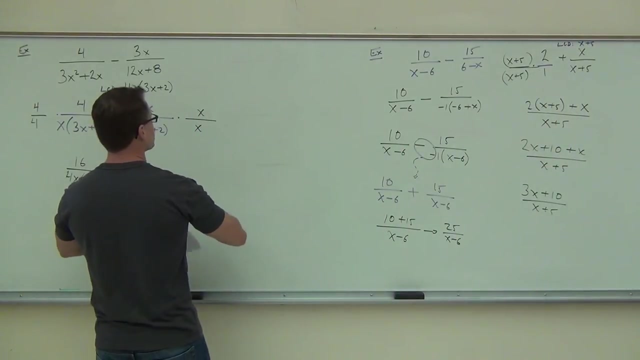 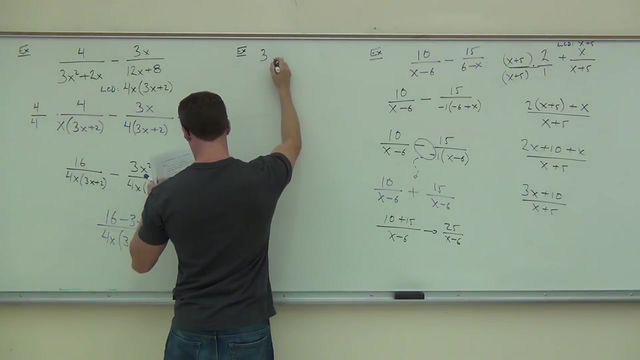 We can't factor this one, All right, So you're done. If you can't factor that, you can't simplify anything. You're done. as far as you can go, You okay with that one. Okay, now I'll give you two to try on your own. 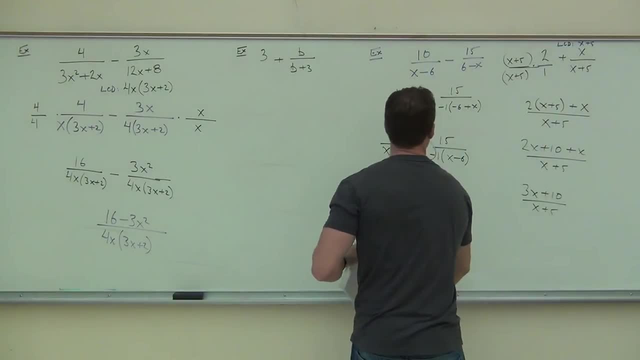 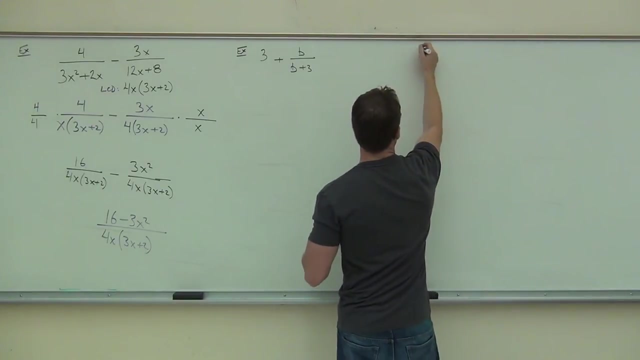 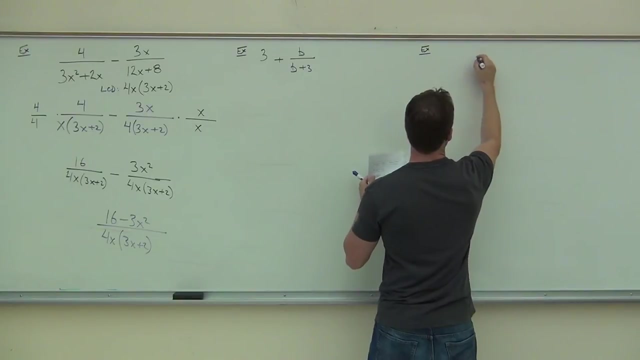 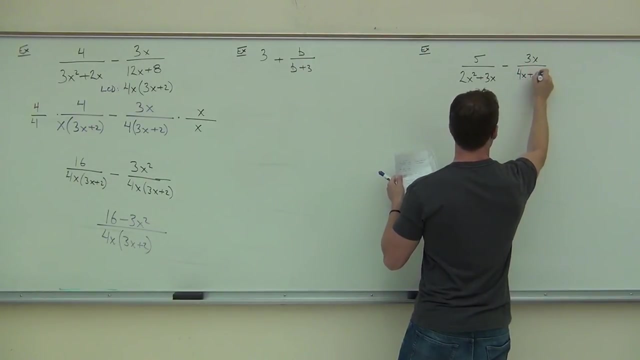 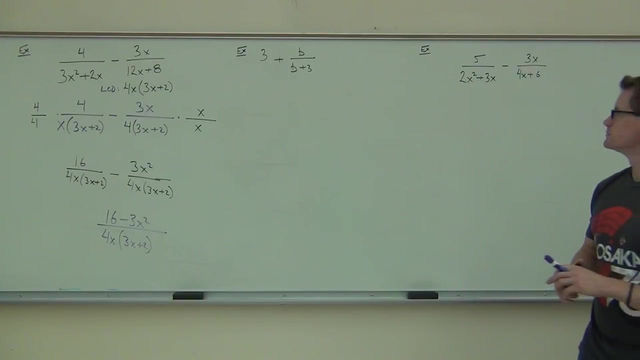 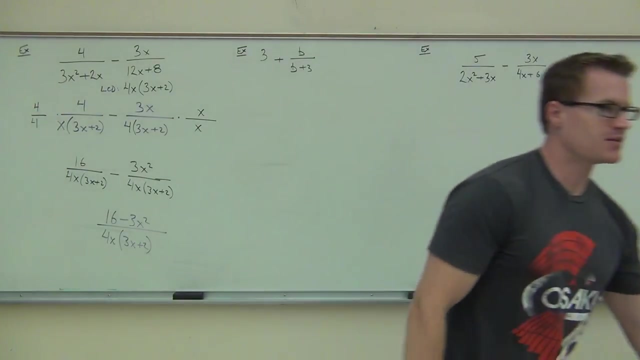 So we're going to start on that one and I'll write one more up on the board in just a second. All right, here we go. So work on those two. If you're feeling brave and you finish those two and you want to try another one, we are. 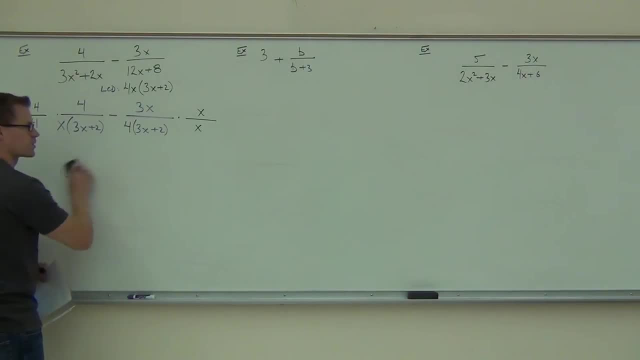 going to do this one in just a second, but I'll write one over here If you finish those two for sure. then, if you feel brave, try this one. if you're feeling good about this stuff, All right, Well, try it anyway, whatever it is. 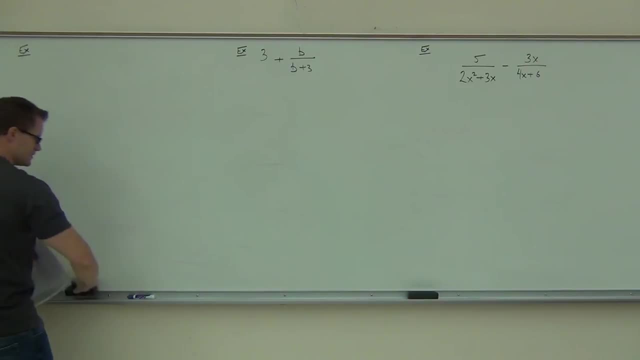 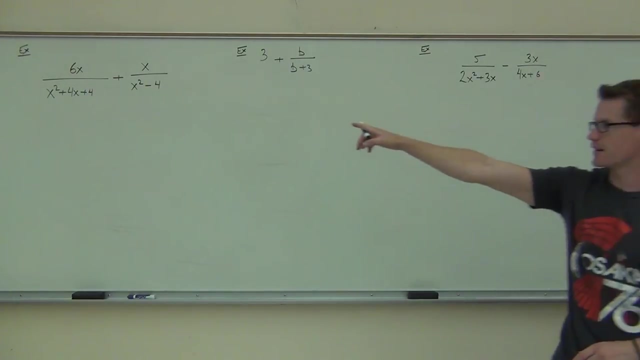 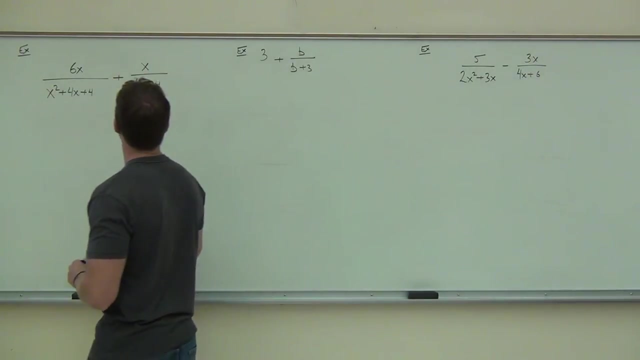 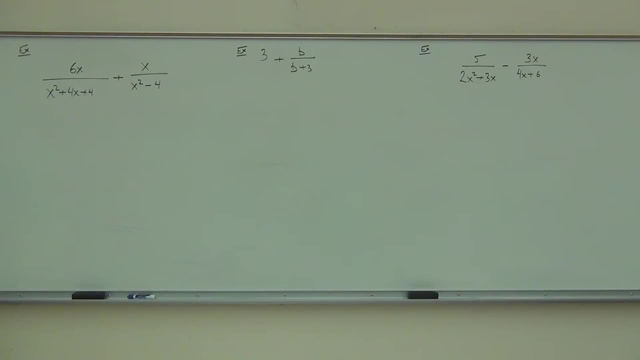 All right, All right, We're factoring if we have to. We're definitely finding an LCD. We're using that to make equivalent rational expressions. that's purposely unsimplifying. to put them together, We're making one fraction out of it. 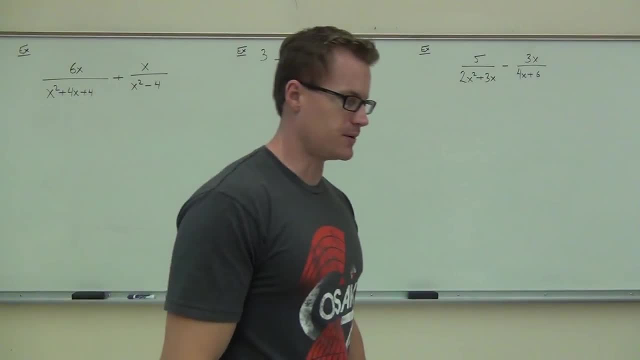 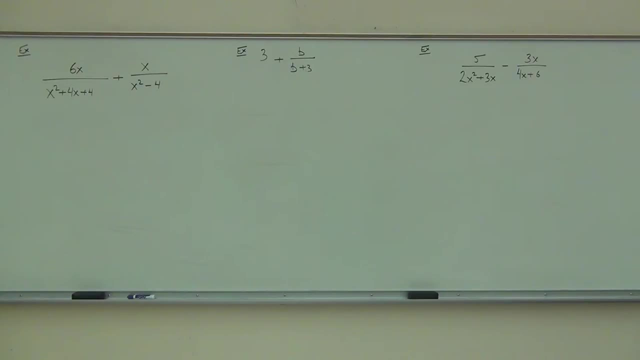 distributing, if we have to, combining like terms and then we start simplifying. Yeah, I see lots of good work so far. That's great. By the way, is there any more homework to turn in? All right, We'll take about another minute. 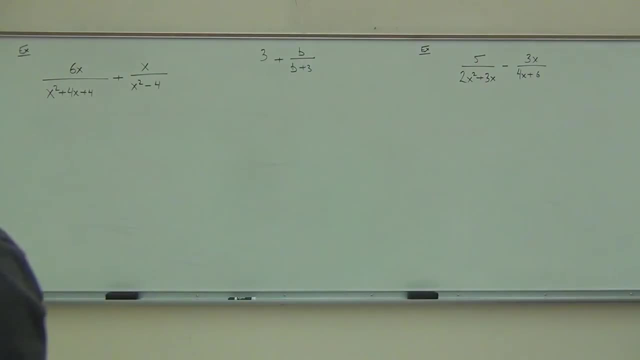 Another minute to try to wrap up the problem that you're on. Hopefully you've done the first one and you're working on the second one. at least, If you're done with the second one, I do want you to try the third one. 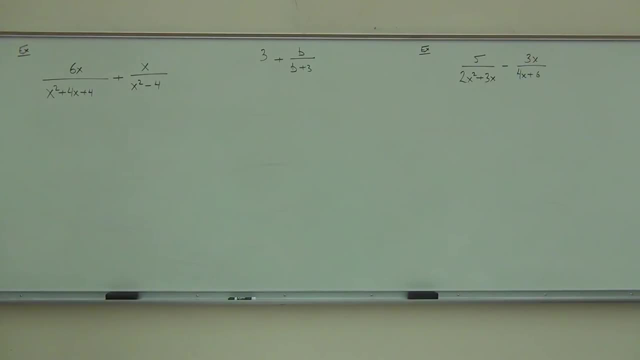 All right, Okay. So in every example we're going to try to factor. If we don't have to, that's great, If we do have to, we do that, But in either case we look for the LCD right after that. 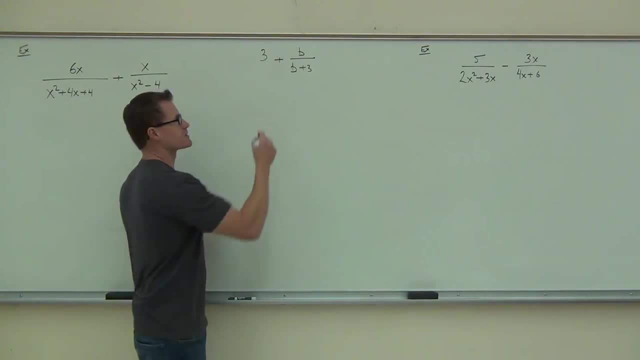 So our first example: well, hopefully you saw this and said, well, I need to make that a fraction. Did you do that? Good, Then we go ahead and find the LCD, because one you can't factor B plus 3.. 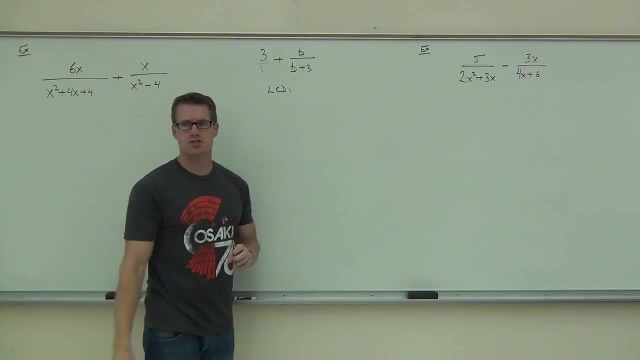 So our LCD? in our case, not too bad, It's just the B plus 3.. That's the only denominator we have. Therefore it has to be the LCD. Did you find that as well? Yes, Next we go ahead and multiply. 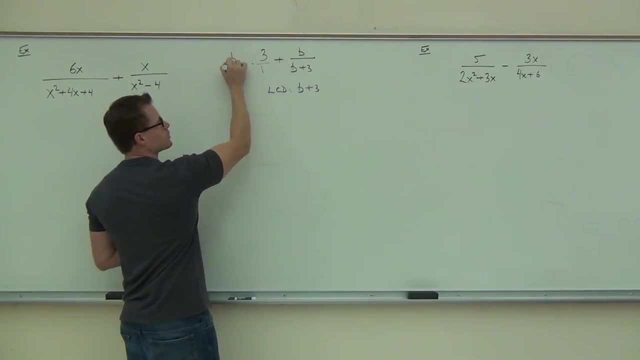 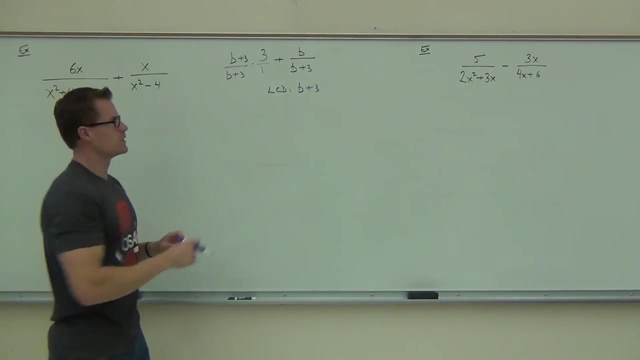 This fraction is great. It already has the LCD. With this fraction, we're going to multiply B plus 3 over B plus 3.. Do you get that far as well? We extend our line. We put some parentheses, like we know how to do. 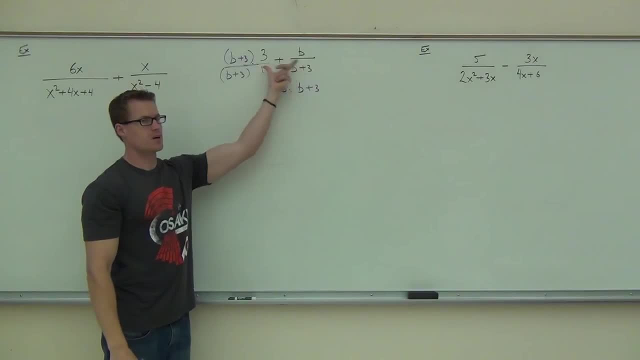 That's not a problem. We notice that, in fact, we do have a common denominator already. That's what we wanted: B plus 3.. This is really just B plus 3, because the 1 doesn't do anything, and that's the same as what we wanted. 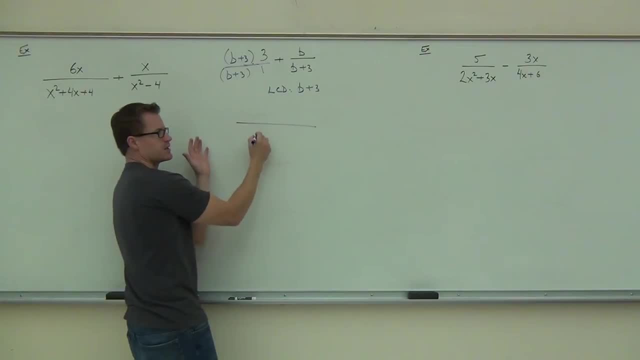 So we'll make one fraction out of this. Our denominator is the LCD B plus 3.. On the numerator, we're going to have B plus 3 times 3.. I'm just going to write the 3 first because that's easier to see. 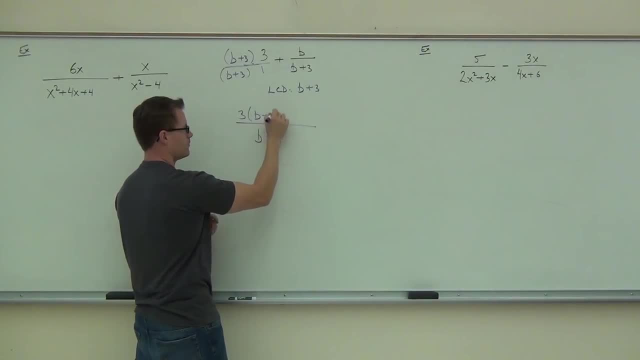 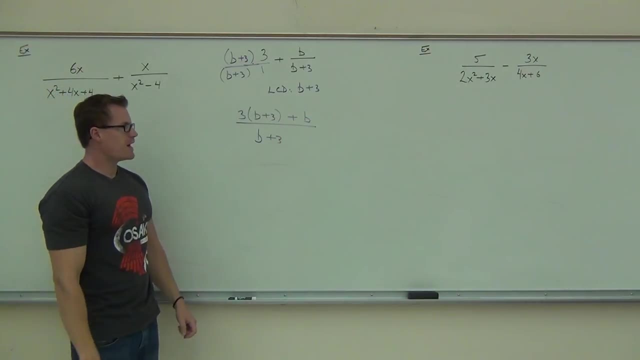 that we need to distribute. That's the only reason. And then the plus B. That's our second numerator After that. we certainly can't simplify. We're going to distribute, So we're going to multiply. We're going to multiply. 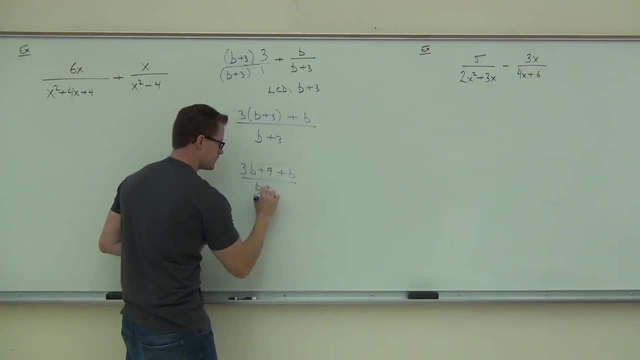 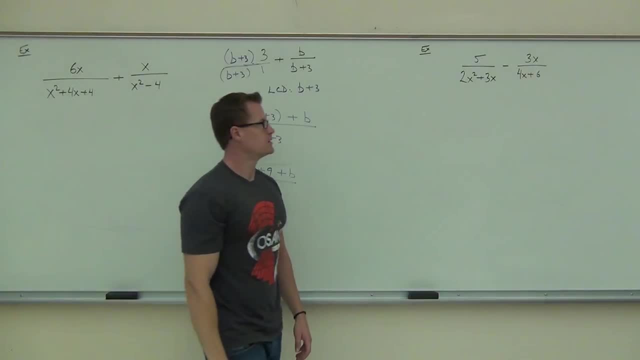 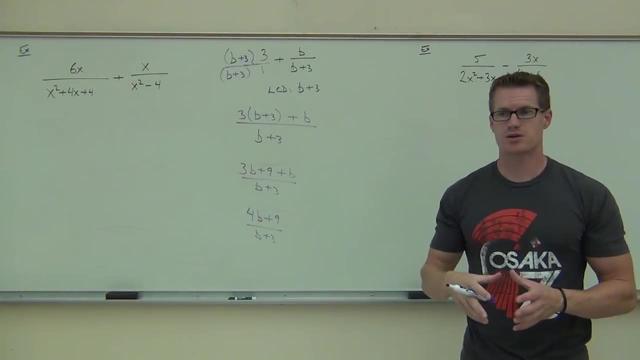 That's great, That's fantastic. Good for you. Okay, next one. Where we couldn't factor the first one, we can factor this one. So we'll look at those denominators and try to factor it. It's very similar to the one I had up on the board here just a little while ago. 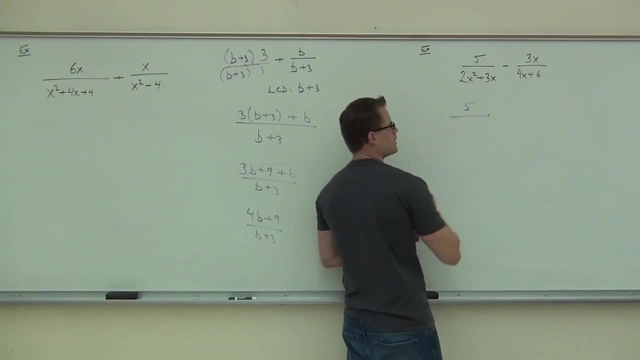 So we'll factor that. The numerator is what we leave alone. What factors out of our denominator here, X. So we factor that out and we get hopefully 2x, 2x plus 3x. Very good, Minus the 3x will stay the same. 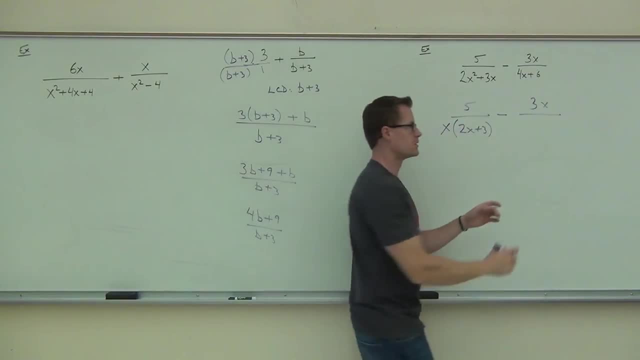 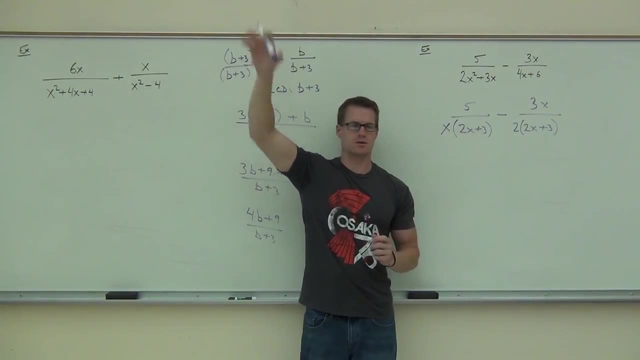 What factors out of this denominator 2. And we get 2x plus 3x. 2x plus 3x- Very good. I don't know how many of you made that part, would you Good, Very good. 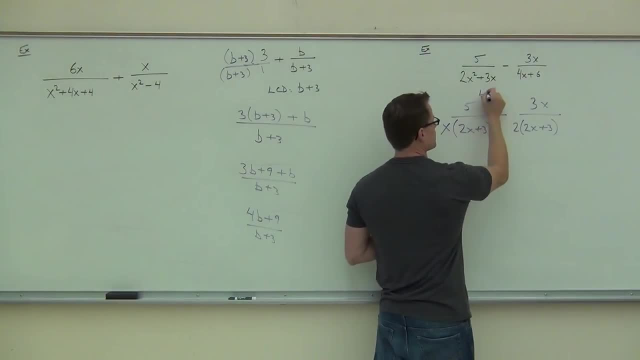 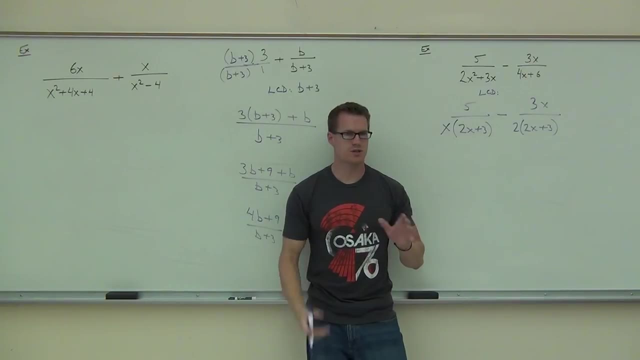 Now We get to find our LCD Again. the LCD is just a listing out of the different factors. So when I look at this problem honestly, the first thing I look for is not the big ones, I look for the small ones. 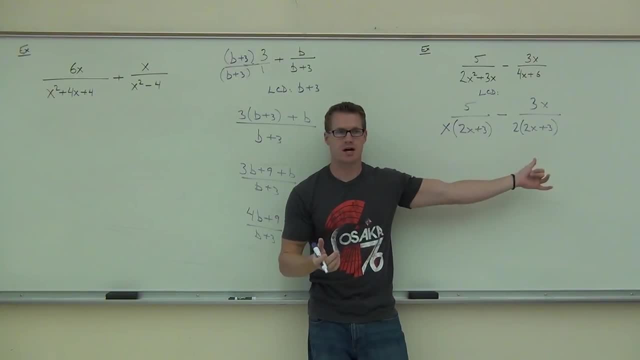 I look for the numbers first. I look for any numbers I have. So here are my denominators. I'm seeing first off the 2.. I'm going to write the 2 first. Then I look for any x's or y's or variables hanging out all by themselves. 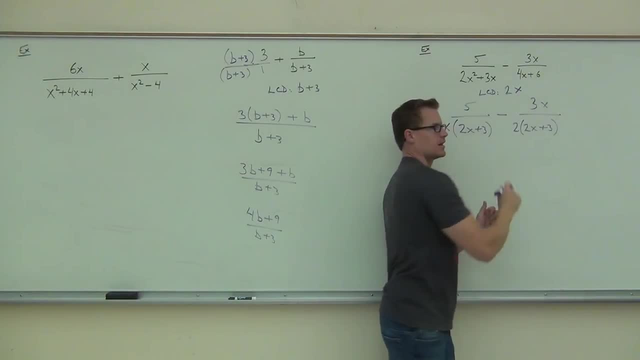 So I've got the 2.. Then I'm going to write the x And lastly, I'm going to write any big factors that I see. I see the 2x plus 3, but I see it twice. They're in different fractions, so I only need it one time to cover both of them. 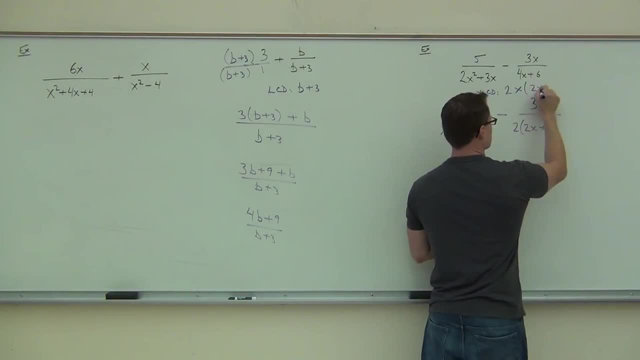 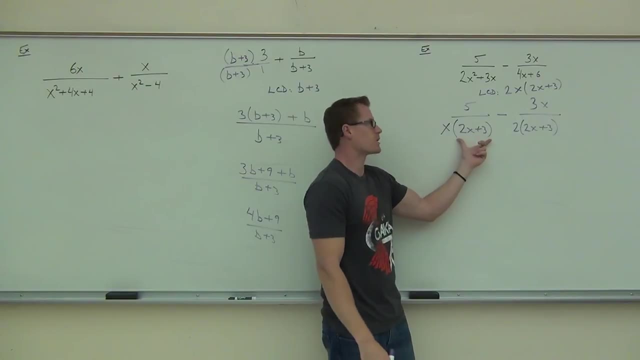 Are you with me on that? And then I double check, I go: all right, do I have the x up there? Yeah, I do. Do I have the 2x plus 3?? Okay, I got that. Do I have the 2?? 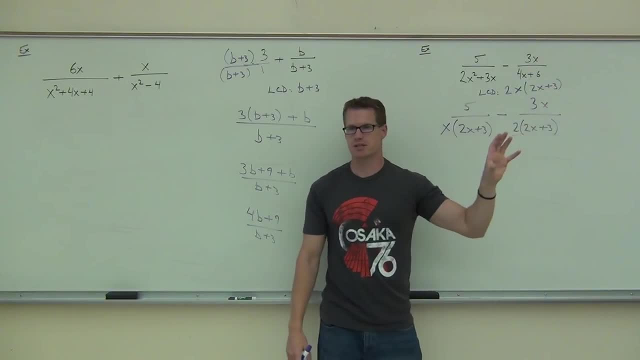 Yeah, Do I have the 2x plus 3?? Yeah, I already covered that, So that's my LCD. Did you make that part? No, Awesome. Now we get to multiply by what's missing On the left side. I notice I have an x and the 2x plus 3, but I'm missing the 2.. 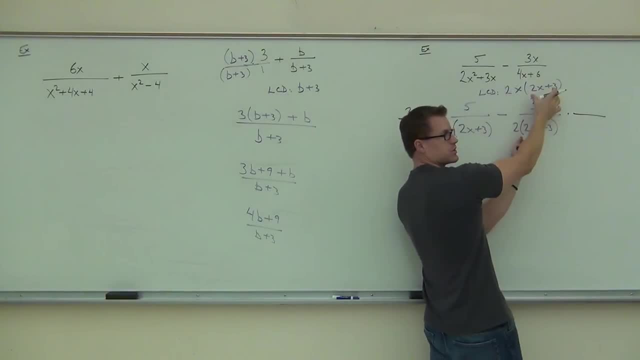 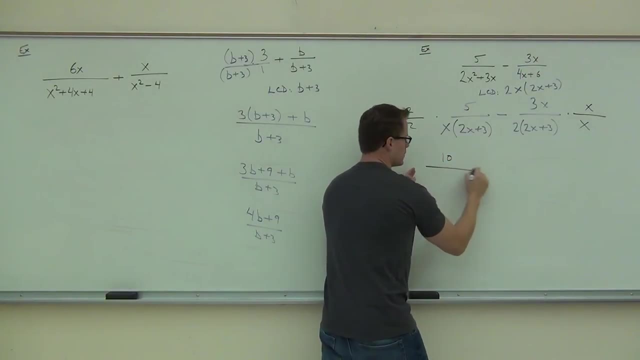 On the right-hand side. I've got the 2,. I've got the 2x plus 3, I'm missing the x. Now we multiply to get our 10 over 2x, 2x plus 3.. Never distribute that denominator. 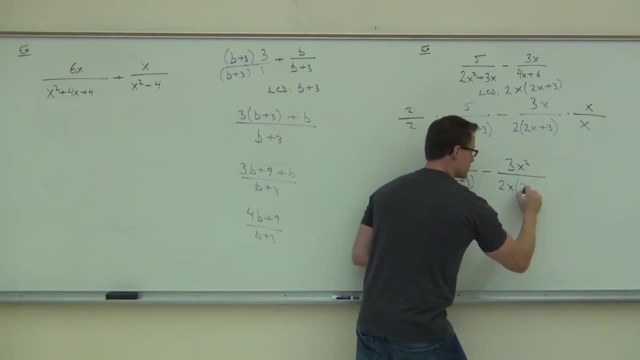 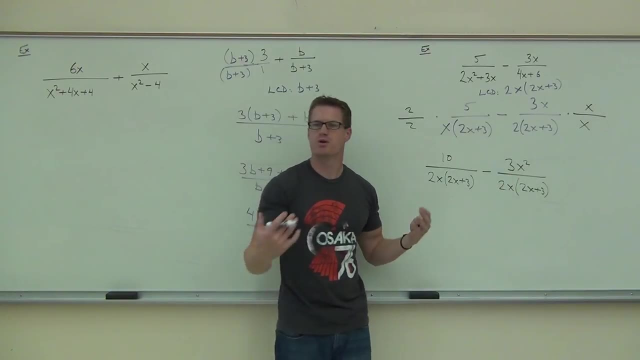 3x squared, like we had last time, And 2x, 2x plus 3 over there as well. We notice LCD occurs in all three spots. That's exactly what we want. We can make one fraction out of this thing. 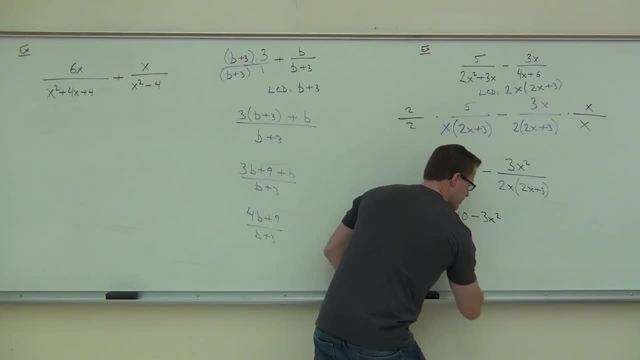 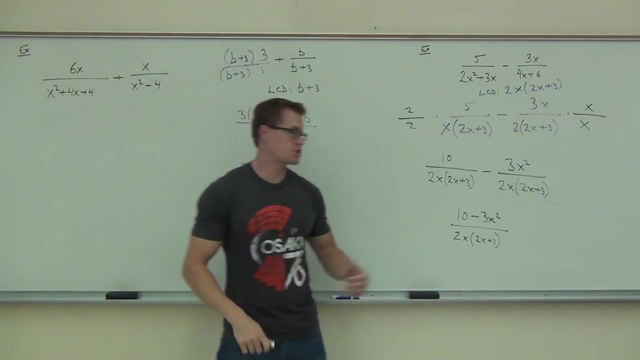 We'll get 10 minus 3x squared over our LCD. We would try to factor, but you can't factor that thing, so you're done. How many of you made it that far? Good, that's fantastic. Did you try the third one? 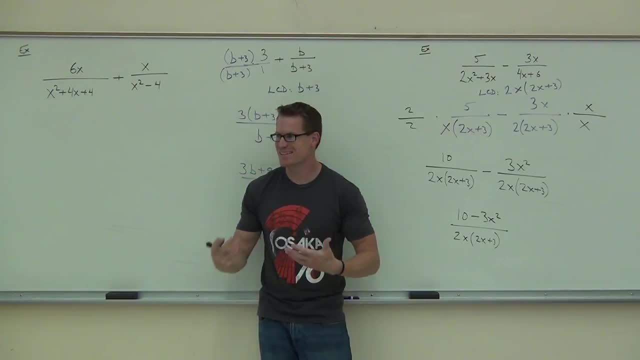 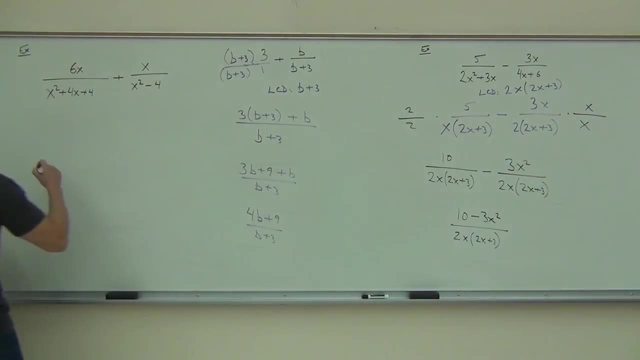 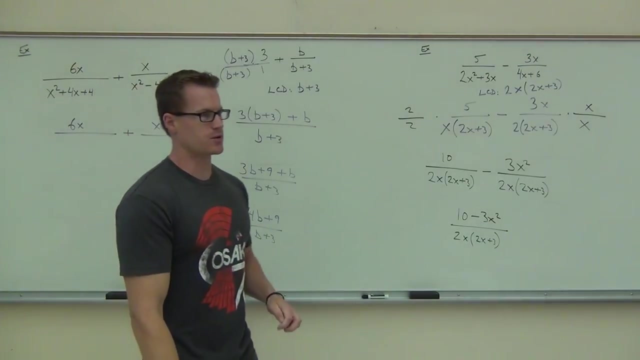 Yeah, It's kind of fun, right. Lots of good factoring stuff. Yeah, We like factoring that You better, right, Because you're doing a lot of this. You know I will. Yeah, of course, the first thing we do do is we factor the denominators. 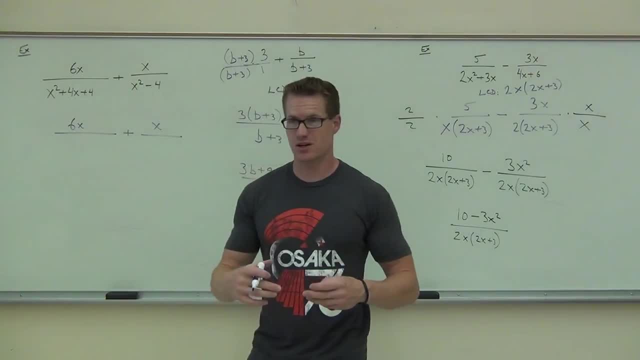 We have to Now one of these things… Actually, both of them are stuff we've seen before. One's a diamond problem with no extra step. Why doesn't it have the extra step on it? They're not in the diamond problem, Great. 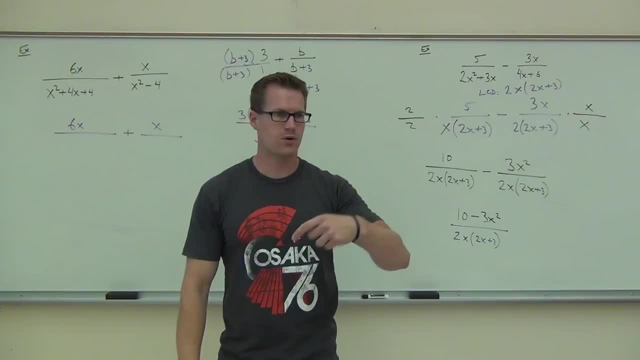 Those are kind of nice, right? Quick diamond problem: four and four, two and two. We just do x plus two, x plus two. Did you get that as well? The other one is the difference of squares, which should just be bam in your head at this point. 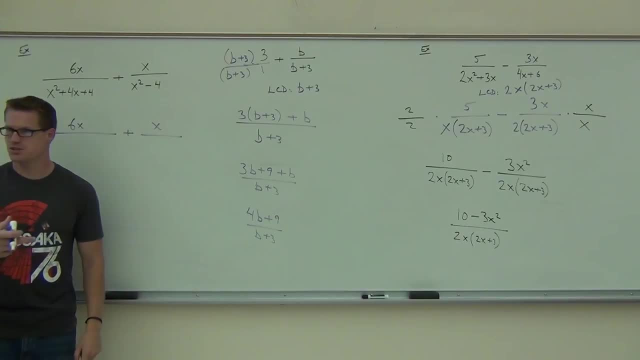 We got x squared minus four, but x plus two, x minus two. Did you do those? Let's go. So here again, we got four and four. The numbers that work there are two and two, X plus two, x plus two. 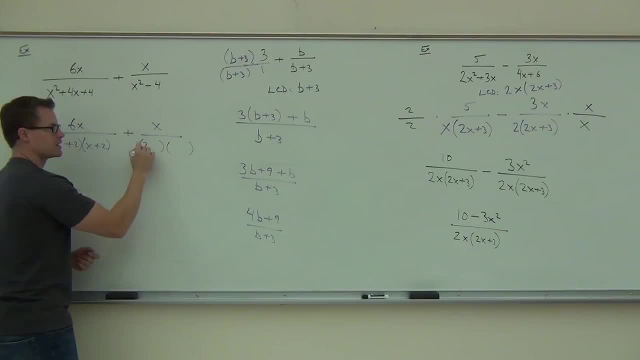 Here we have the difference of squares, and we know how to factor that already as x minus two, x plus two. So the factoring shouldn't hold us up anymore. That should be an easy part of this, not too too bad. 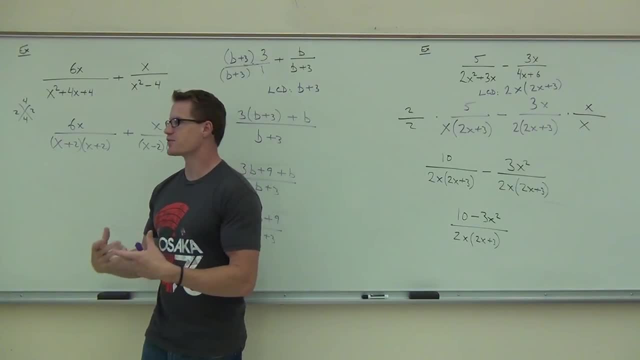 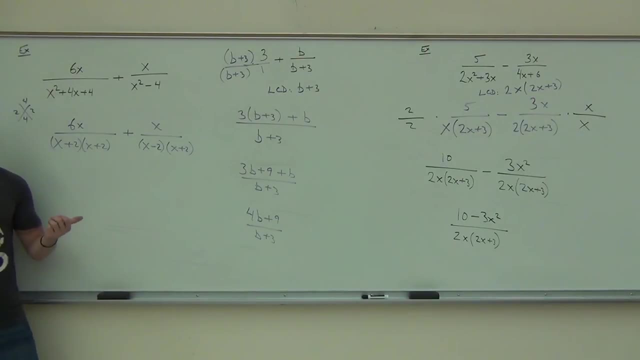 Next we get to find the LCD. Our LCD is going to be every different factor that we have up there and the largest power that occurs. But I mentioned one thing to you and this is why we're doing this example: Before you find the LCD, you have 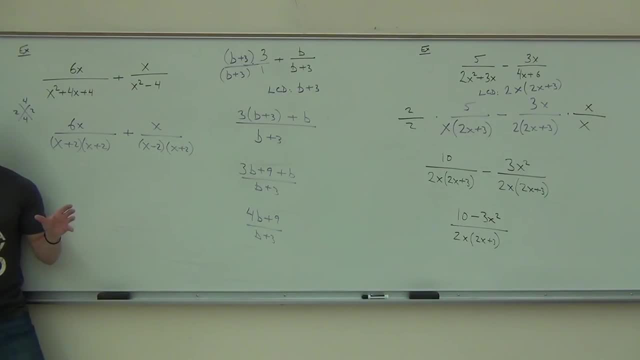 to make the denominators as concise as possible. You have to make them as good as possible. So the problem here is that if you just do this, you don't quite have the LCD yet, And the reason why is because can you write this differently? 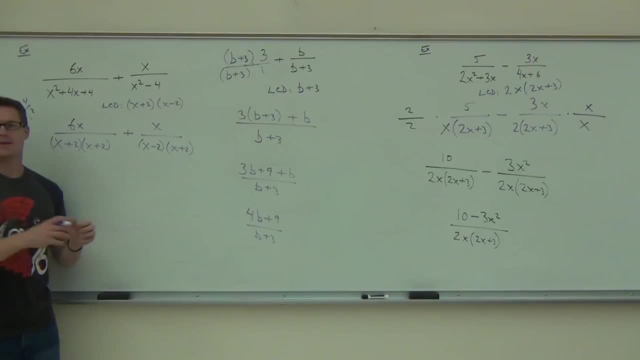 Yes, How could you write it? That's going to make a difference in your LCD because that's a larger power. So here we'll do x squared minus two, And if you do that, this one. we can't put that together. 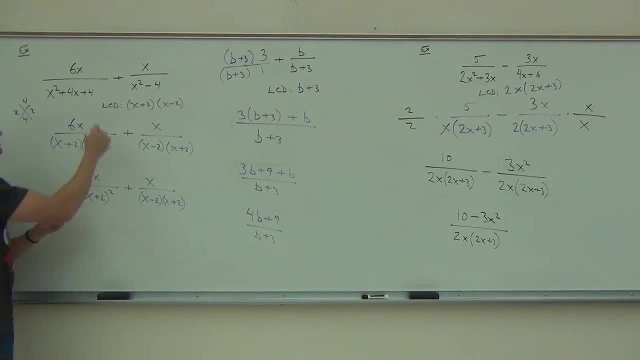 so we leave it, But notice how this is going to change our LCD right here, That, right there that. power two. So now we go through, look for different factors, And here's how you do it. You'd say what are the different factors that I see? 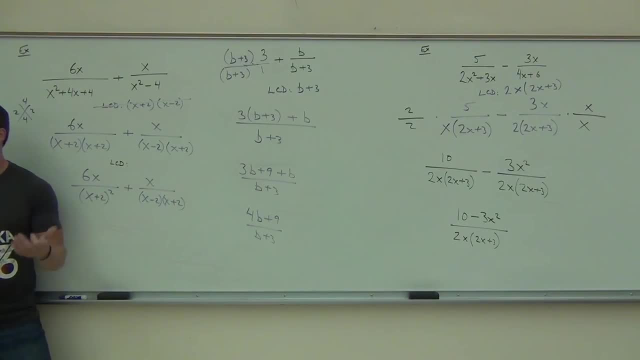 Name a different factor that I see: X minus two. Okay, I get x minus two. What other different factors do you see up there, Plus two, And you're going to take the largest power that you find of x plus two. So, while I have x plus two in both spots, 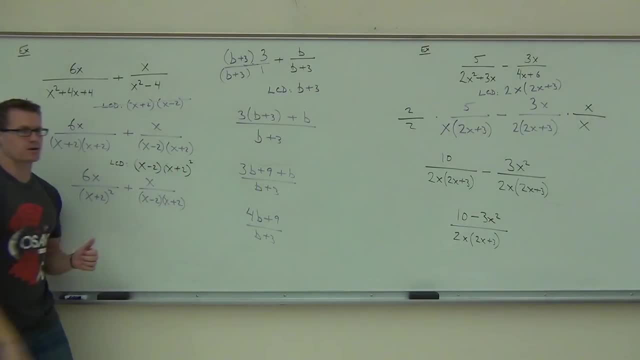 what's the largest power Two. So you have to put the two there. Okay, that's a must. We practice this when we're finding LCD, but you have to remember to do that when they step in front. Yes, Okay. So you have to put the two there. Okay, that's a must. We practice this when we're finding LCD, but you have to remember to do that when they step in front. Okay, So you have to remember to do that when they step in front. 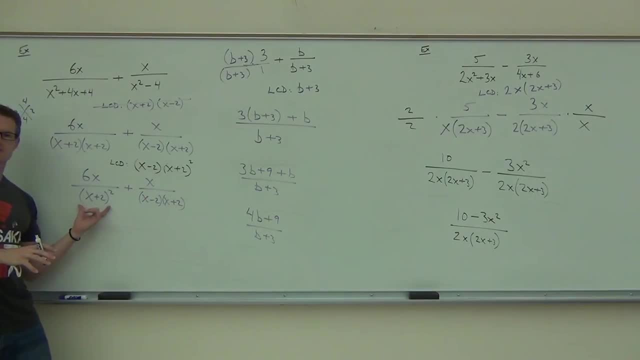 And now we're going to double check just to make sure we got that. Do we have an x plus two squared? Yeah. Do we have an x minus two? Yeah, Do we have an x plus two? Yeah, we have at least that much. 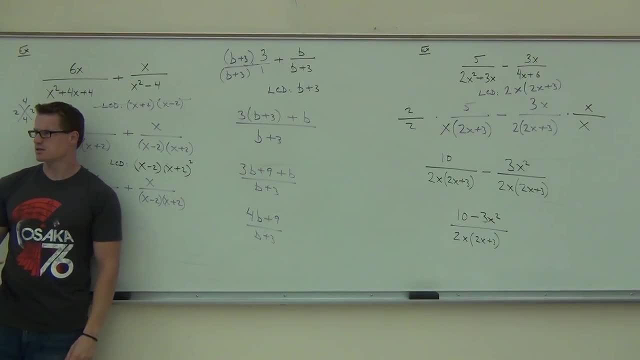 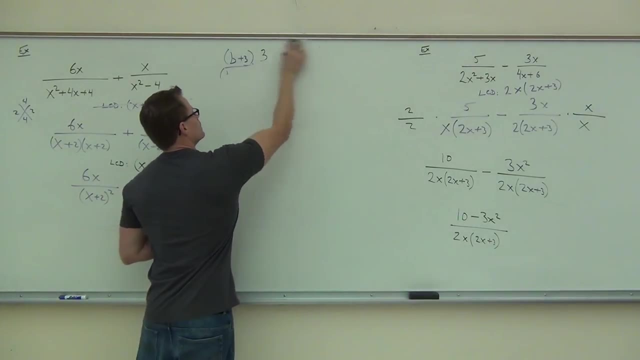 It's right, there. Are you with me on this LCD in this case? Yes, Okay, We're still going to multiply by the appropriate things. now Let's try to figure this out together. On the left-hand side, this one's going to be the easier. 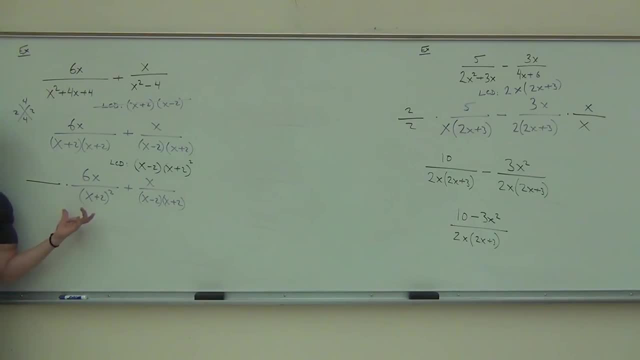 of the two sides to really see. Can you tell me what's missing that I need to multiply by, Please. X minus two. Great, On the right-hand side. am I missing anything? X plus two. Good, I'm missing x plus two because I want squared. 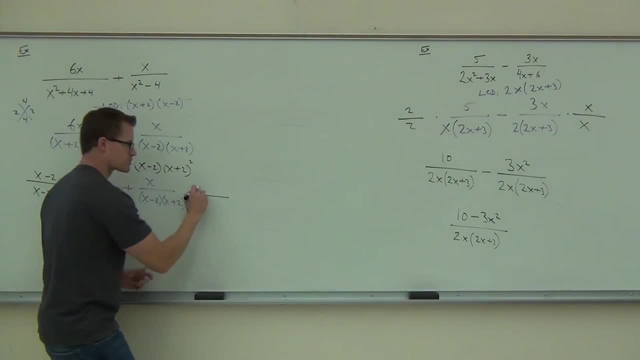 I only have one of them, So it's already got the x minus two, I just need one more x plus two. You okay with this so far? Yeah, All right. Well, we know what to do. We're going to extend our line. 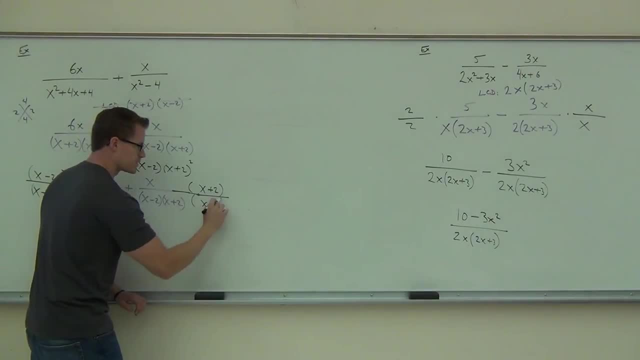 Okay, So we're going to extend our line. Okay, So we're going to extend our line. put some parentheses. I'm going to do an extra step here, just so you can see the concise form of this, to make sure that we actually do have LCD. 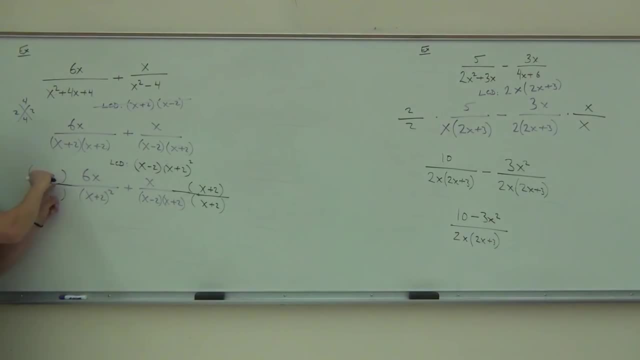 I am going to write this part first: my 6x. I like that first because we're going to be distributing that in a second, My x. I'm going to keep that in front. So we're going to have 6x x minus two all over x minus two. 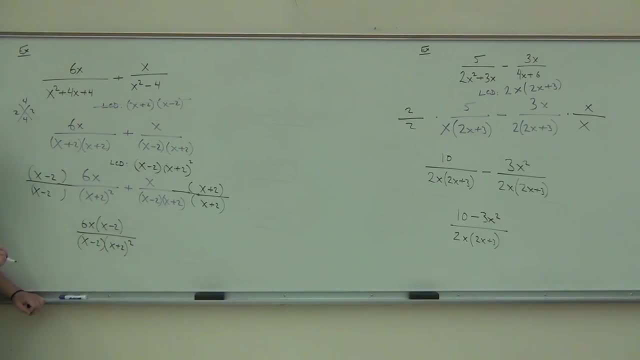 So we're going to have 6x plus two squared. x plus two squared. Ladies and gentlemen, should I simplify this? No, No, I'm purposely unsimplifying to keep my common denominator Plus x times x plus two over. this is x minus two. 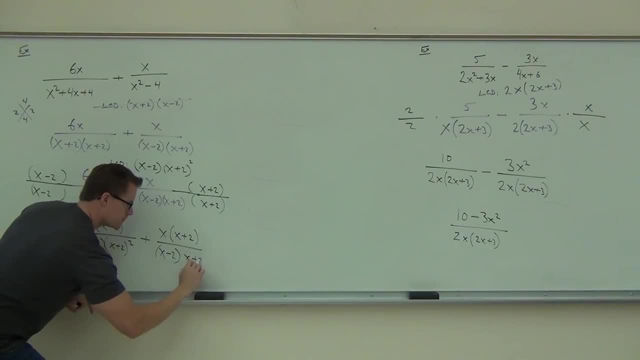 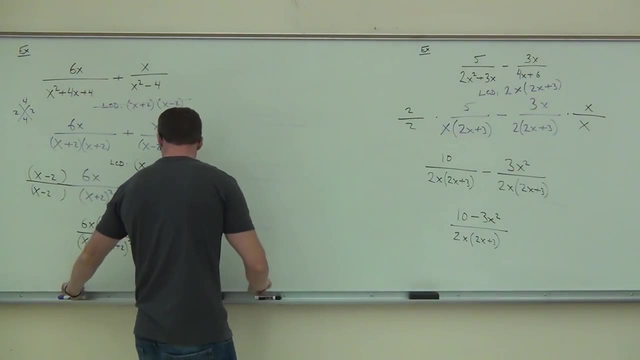 And look it, that's x plus two squared, And right there we can see that I do have my common denominator. That's what we wanted, All right, So we'll continue up here. We're going to write this as one fraction before we distribute. 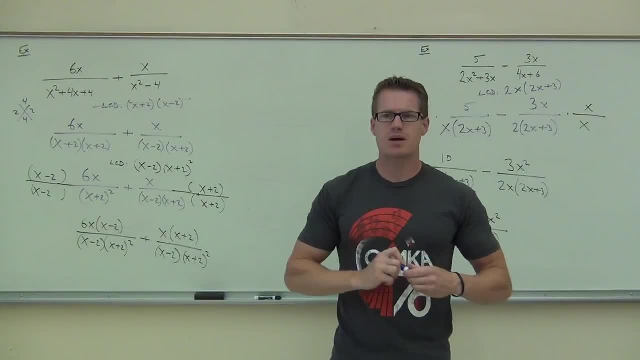 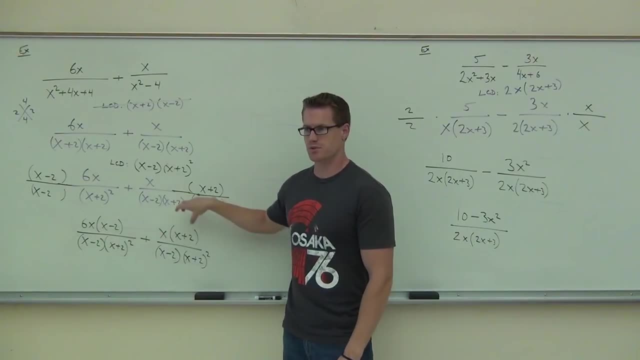 Now I know some of you are thinking: why do we actually do that? In this example it's not so crucial because we have a plus sign. But do you notice that if that would be a minus sign, that minus sign would distribute to both terms? all right, 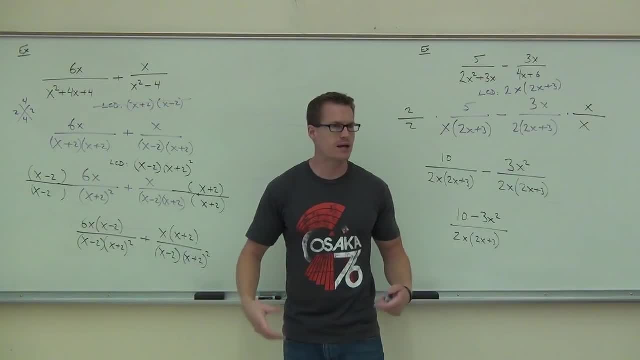 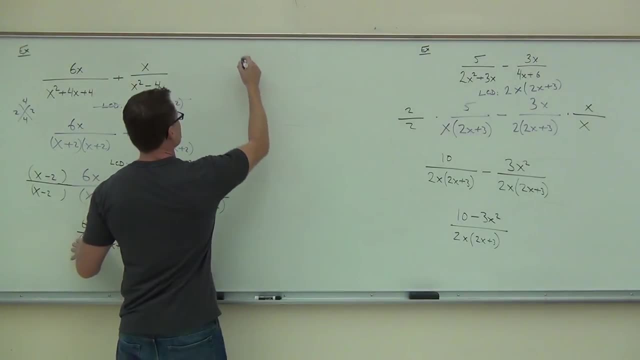 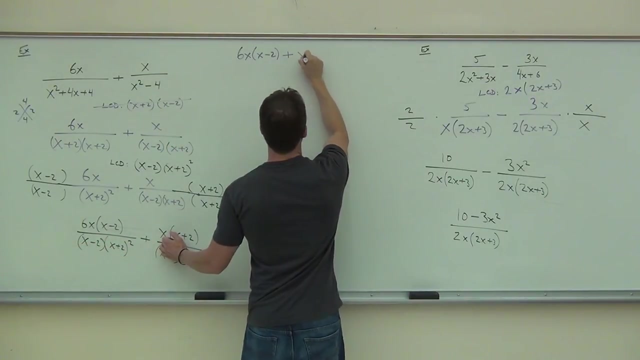 And if you distribute now, some of you are probably going to forget that. I can't have you forget that. So we wait until we get one fraction before we distribute in combined like terms. That's the idea. So now we get to distribute. 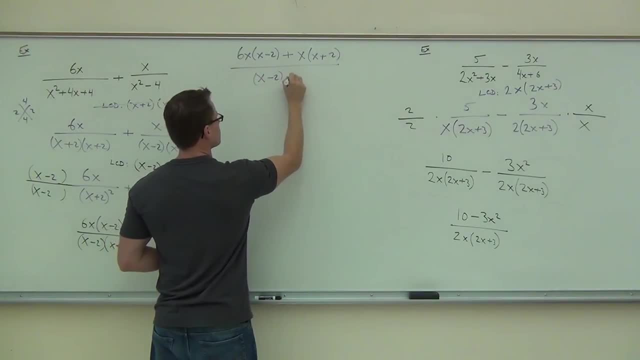 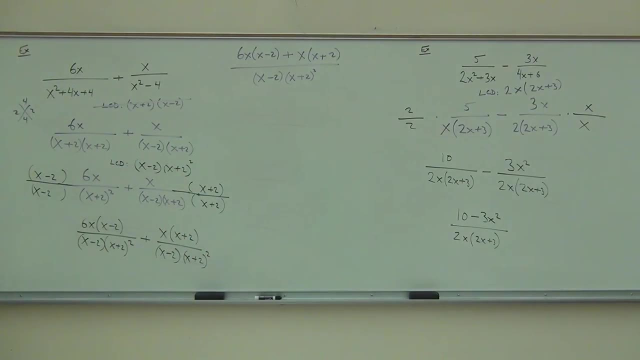 Now we get to distribute. So can you tell me what we're going to have? if I distribute this thing on the numerator, What am I going to get? Six squared, Beautiful, all right. And then Minus one, Perfect, keep going. 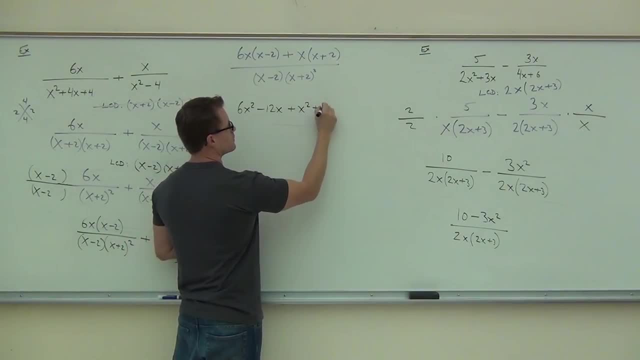 Plus x, squared plus x or plus 2x. OK, not so bad, not so painful, right, Just distribute. Denometer stays exactly the same. In fact, once you find your LCD, you really don't change it until the very last step. 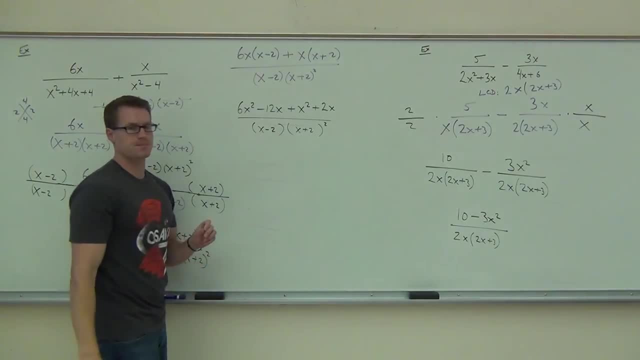 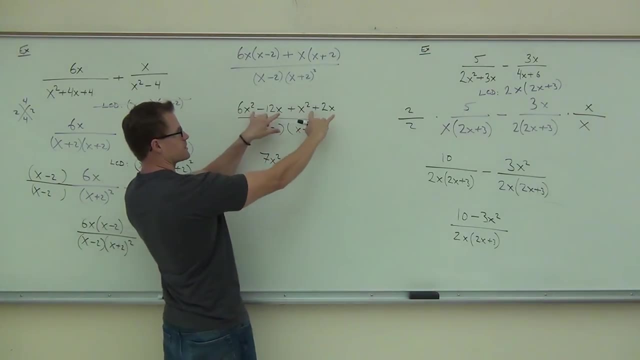 if you can simplify some stuff. Next step: I see my x squared, so it's giving me 7x squared. I see this gives me minus 10x. Now the next thing you might try to do is at least think through the factoring, OK. 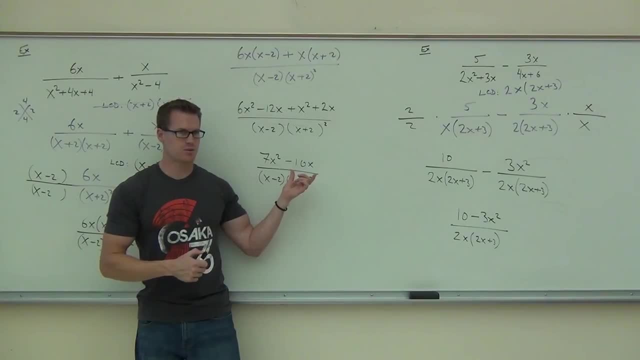 Now, if you look at the numerator, you see you can factor out the x. Do you see what I'm talking about? You can do that, but you're going to get 7x minus 10, which is not going to simplify. 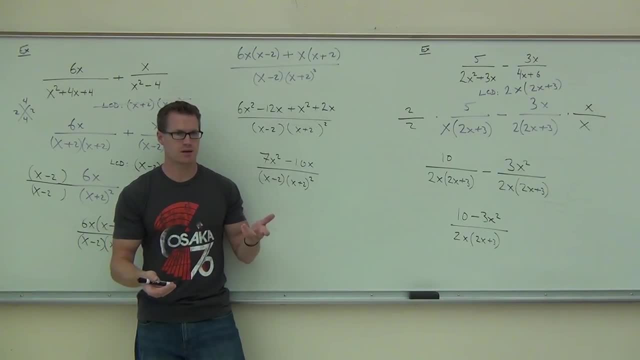 So it's up to you whether you want to factor it or leave it. in this case, Just check it. make sure that if you did factor it, it wouldn't simplify, And then you can leave it If you factor and it can't simplify. 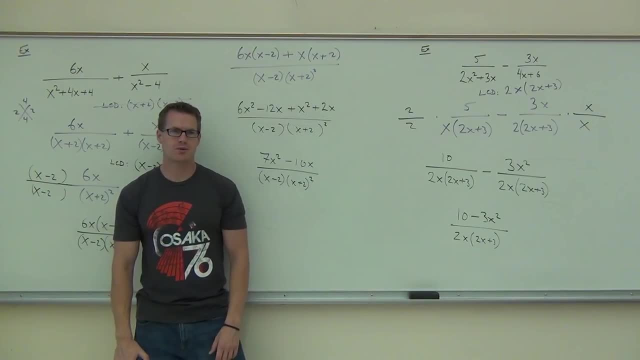 then of course you do that. Would you like to try one on your own? OK, let's do one on your own And we'll go step by step. Well, I'll have you do each step and we'll see how it goes. 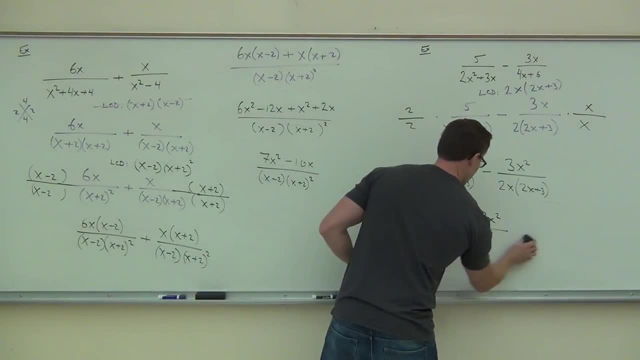 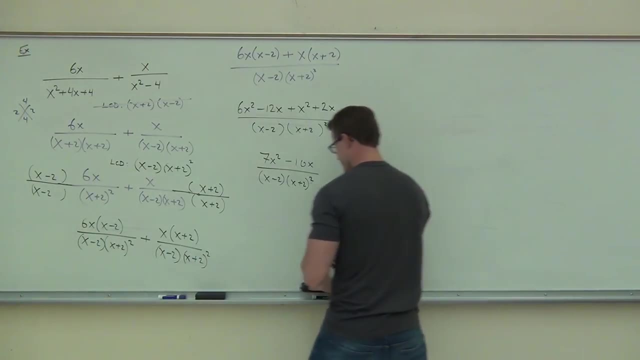 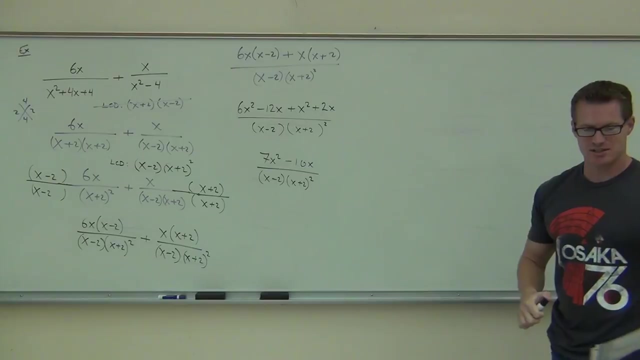 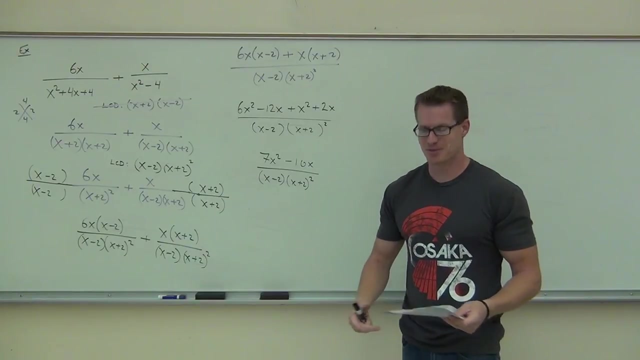 We need to move kind of quickly here. Me asking that question is kind of like the nurse asking so: do you want a tetanus shot Because you know it's good for you, but you really don't want it because it's painful. Yeah, the nurse actually asked me that the other day. The doctor's like: do you want a tetanus shot? I was like no, She goes. well, you're going to get one. anyway, I snuck out before she could give it to me. 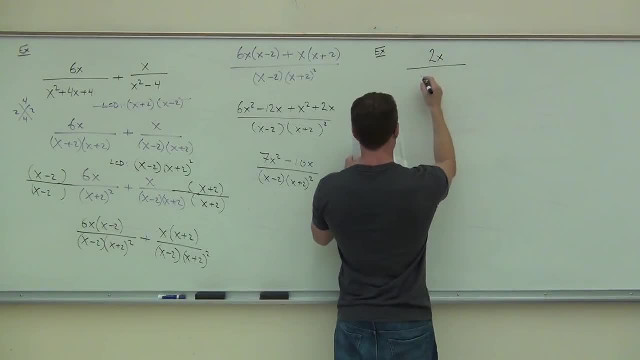 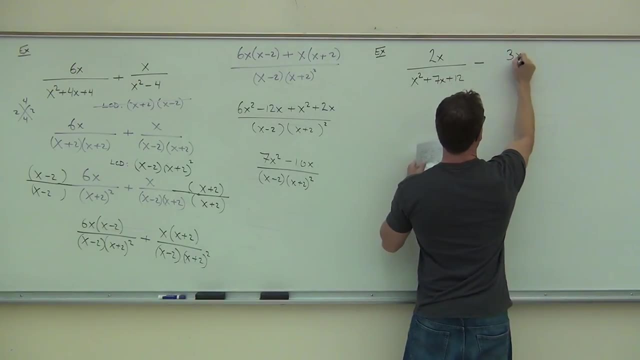 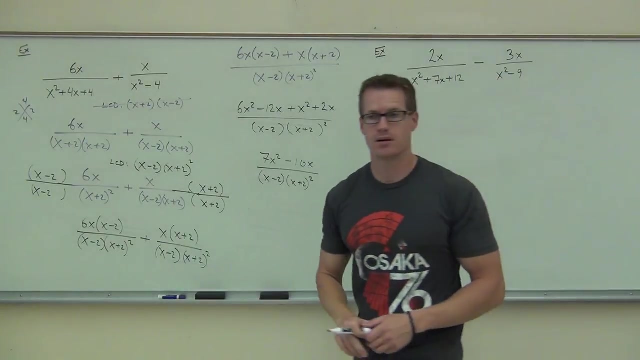 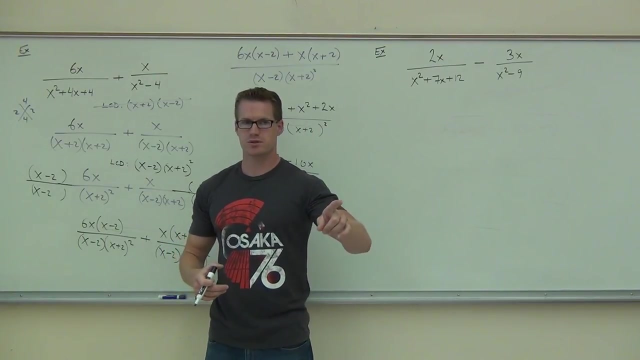 I did. That's horrible. Okay, now we should be very familiar with these problems. First thing I need you to do is do the very first step, which is to do what folks Factor. Go for it. I'm not going to have enough room over here. 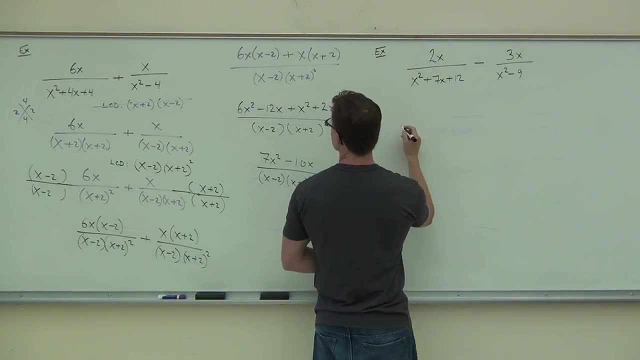 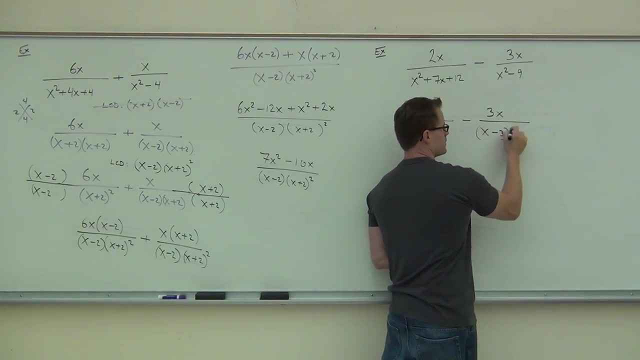 So factoring these should be kind of apparent to us at this step, at this point. This is the difference of squares x minus 3, x plus 3.. Did you get that? Yes, Fantastic. So what's going to happen? 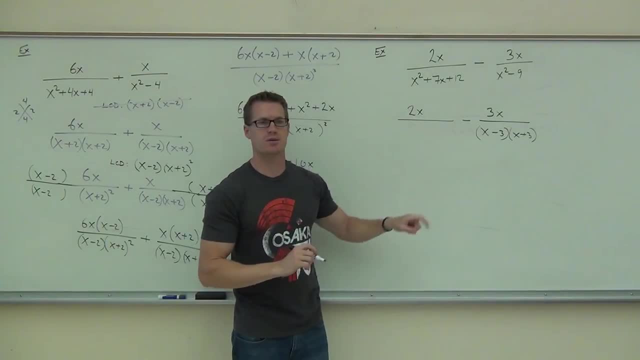 Is 7 on the top, 12 on the bottom. Are they done with the problem? No extra step. Yes, So we should be getting 3 and 4, x plus 3.. Both positive? Yes, Okay. 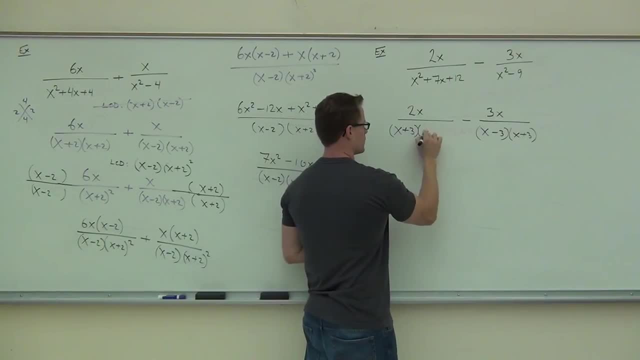 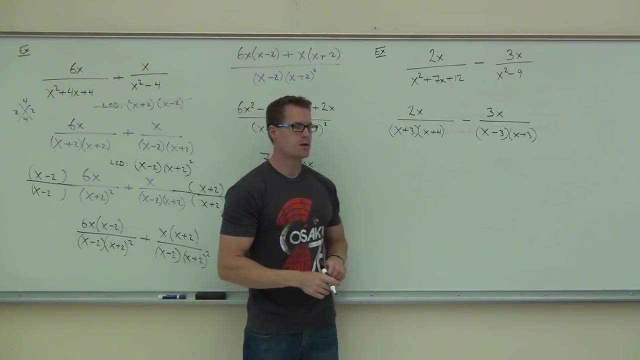 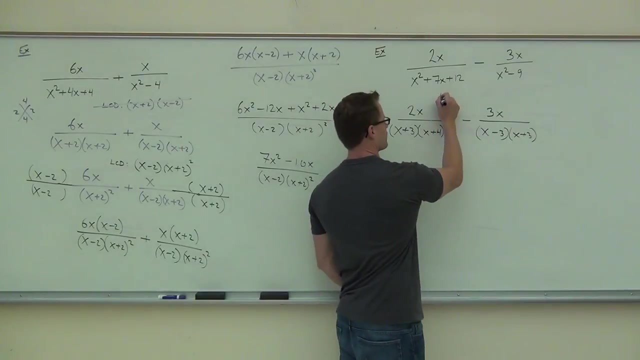 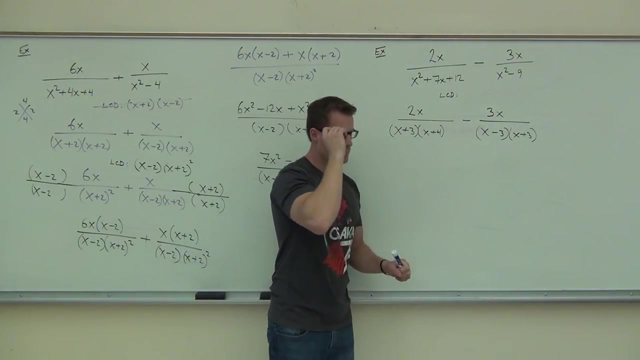 Now at this point, there's really no. there was no grouping to make squares. That's okay. What we want to find out is: what is the LCD? So go ahead and do that at this point right now. Hopefully you've done that now. 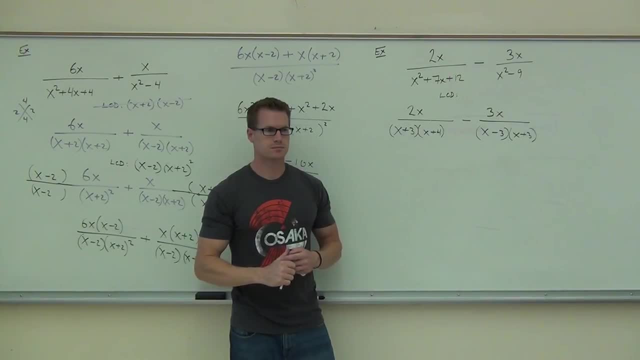 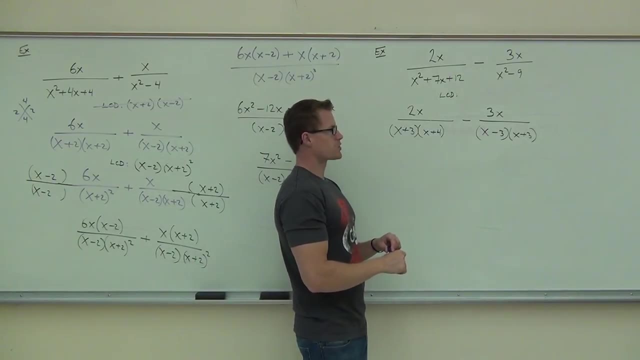 The first factor that I want to introduce here is four elements, So I'm going to call them five elements- Okay, We don't want to use all of them- or the first factor that I'm seeing is X plus 3.. Give me some other factors that I need. 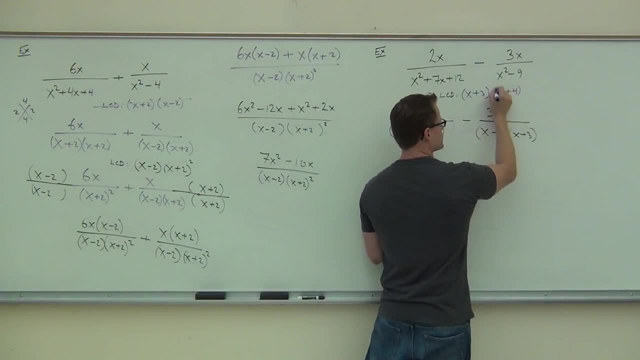 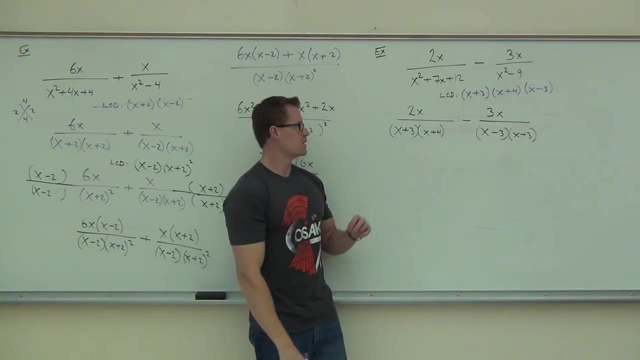 X plus 4.. Good, Somebody else Minus 3.. What was that? X minus 3. Perfect, Where are you able to find the LCD? Good, Okay, I'm going to double check it. Does it have the X plus 3?? 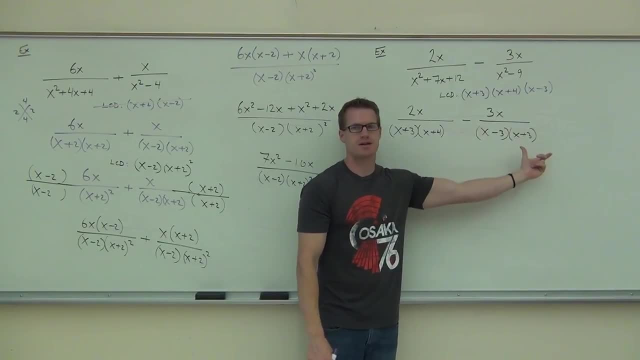 Yeah. X plus 4? Yes, X minus 3? Yeah, it already had the X plus 3.. We don't need a square up here, because we didn't have two of the same factors on the same fraction Here we did. 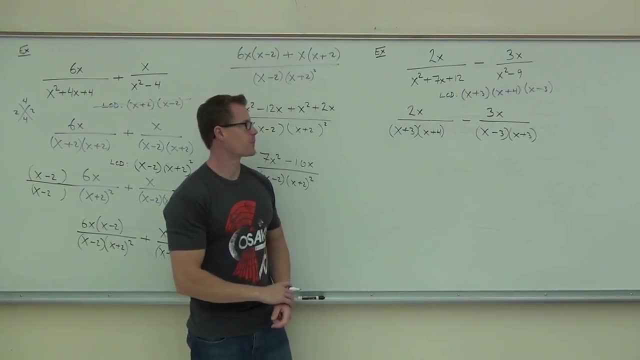 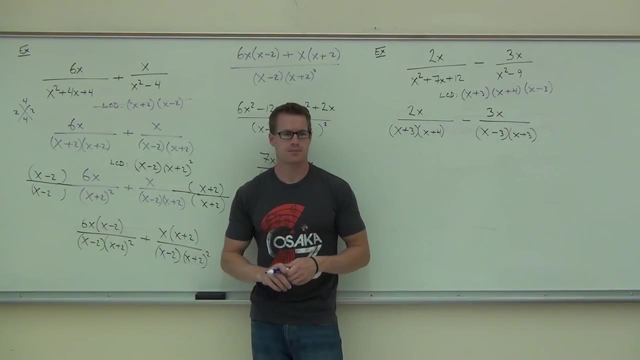 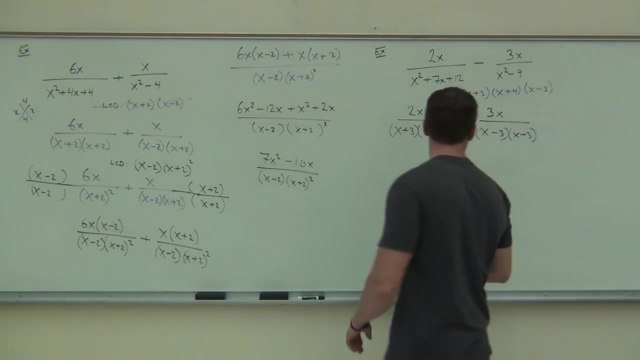 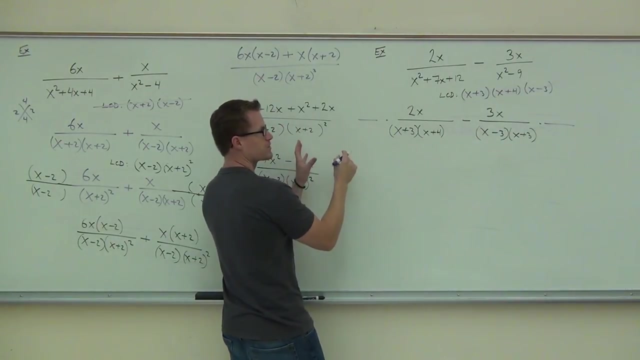 Here we don't. Okay, Now, after you find the LCD, use that to make your equivalent expression. So if you haven't done that, do that now. If you have done that, do that now. On the left fraction, we're missing the X minus 3.. 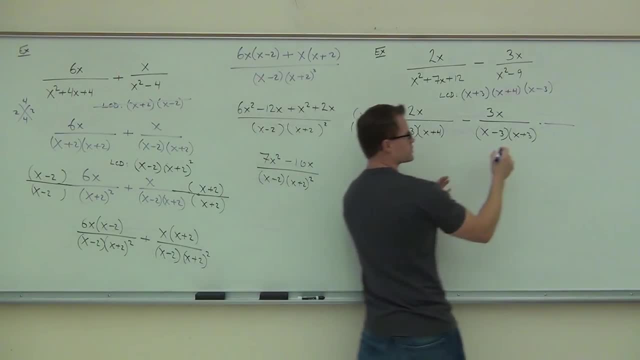 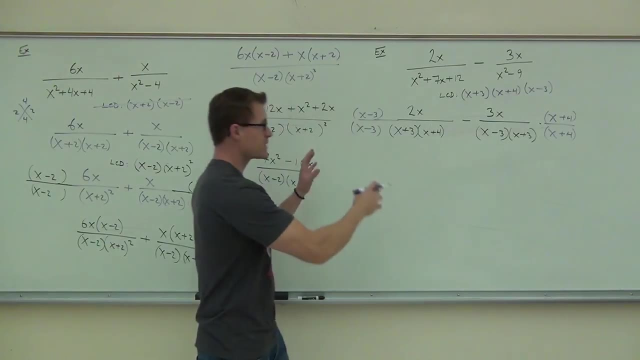 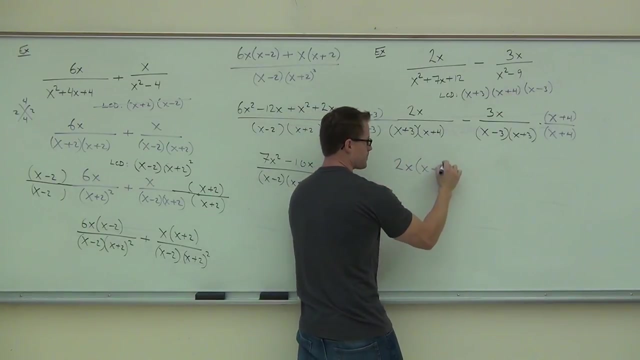 On the right fraction. we're missing an x plus 4.. Of course, we have the common denominator, So what I'm going to do is write this appropriately with a 2x times x minus 3.. I am not going to distribute this yet. 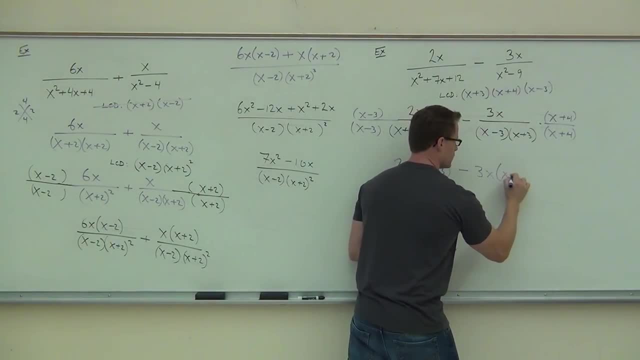 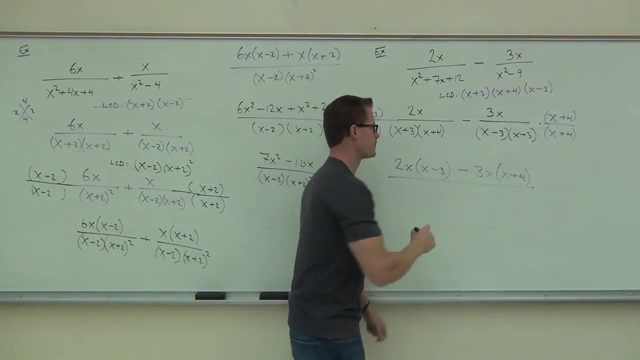 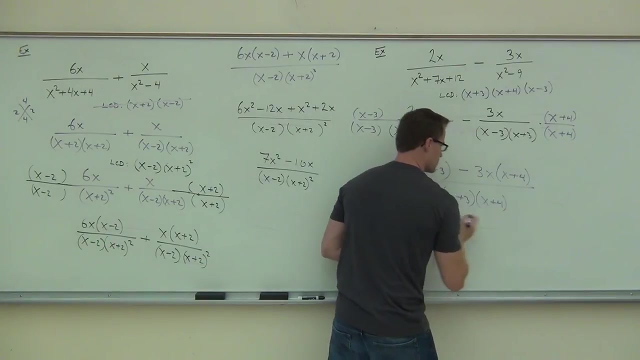 What I'm going to do is write this as one fraction. before I do that, because that minus sign that is going to distribute My LCD doesn't change, I'm going to distribute, combine like terms and then we're going to be done. 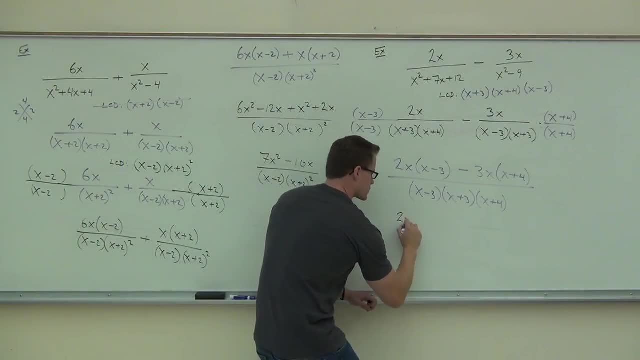 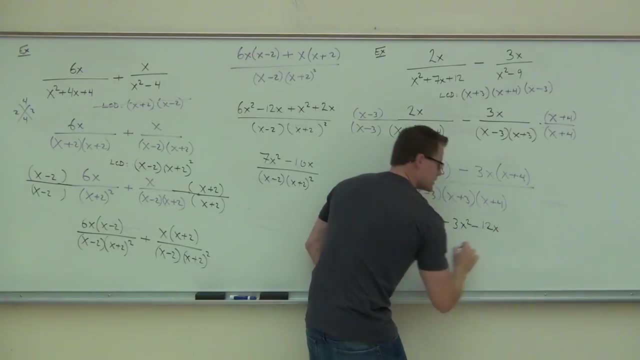 So distributing. hopefully. you've done this already. You have the 2x squared minus 6x- Good, And then we're going to have minus 3x squared minus 12x. Did you make it that far? Yes, Especially the minus 12x. 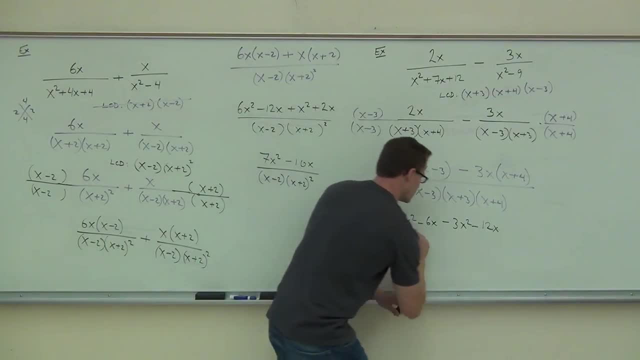 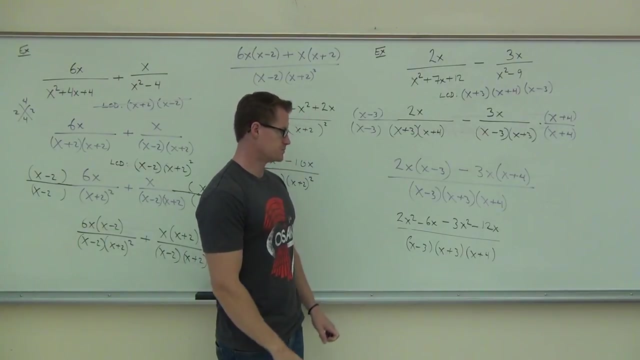 You have that Good. The last step we're going to have to do here is combine some like terms and then write a fraction over again. So if we combine like terms, how many x squareds am I left with Negative 1.. 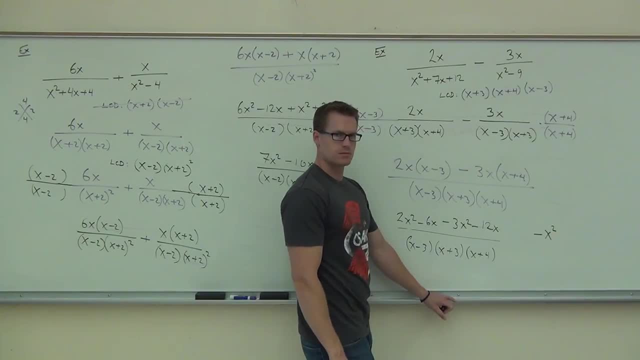 Negative x squared And Negative 6. What Negative 18x? Okay, If you have plus 6x, that sign's wrong. If you have minus 6x, you've done your math wrong. You should have negative or minus 18x on your paper, right there. 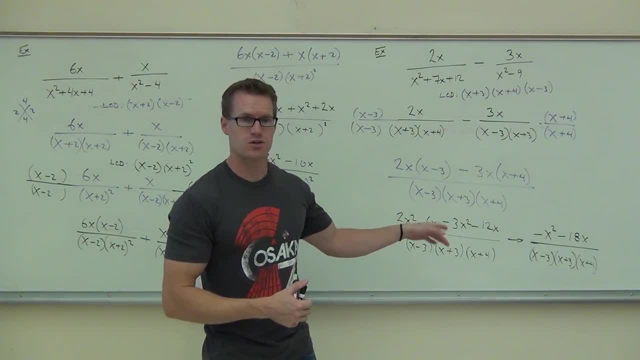 That's about as good as we can do. We can try to factor that out. If you tried to factor, you'd factor negative After negative x. you'd get x plus 18, but that's not going to simplify, so you're good. 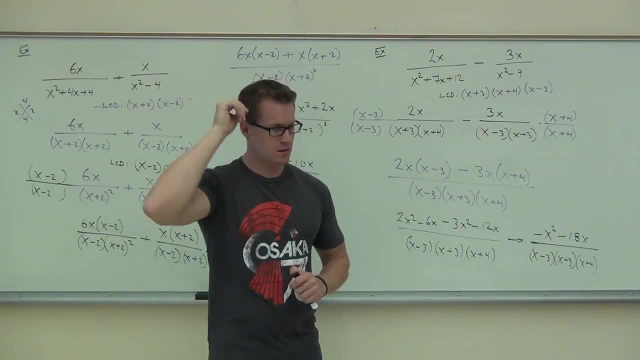 How many of you made it that far, or at least feel good about that? Good, Pretty good. 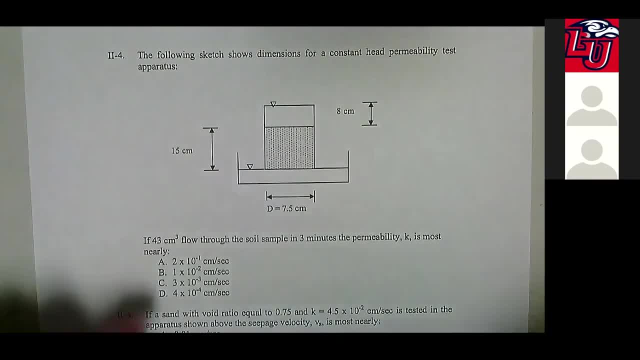 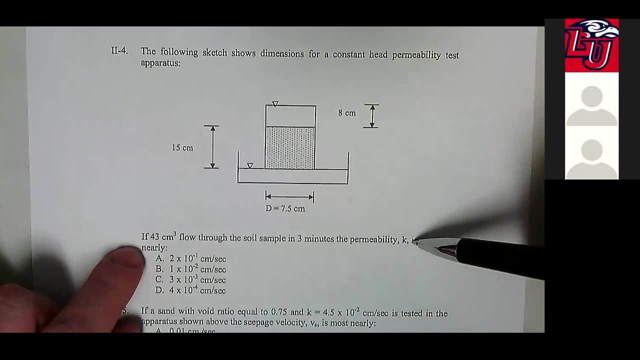 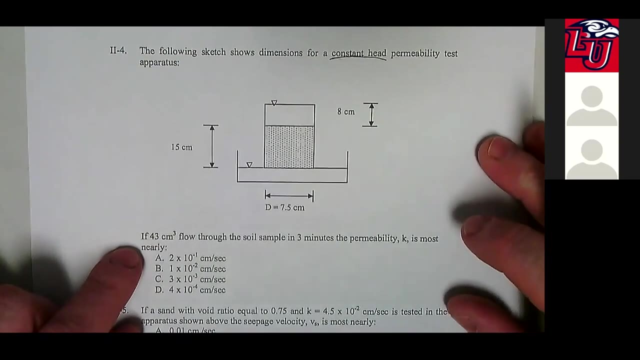 We have 43 cubic centimeters of flow through the soil sample in a time of three minutes. so calculate the permeability. Again, constant head permeability test is key to note here. Remember most of these things. you just flag these equations and highlight them, the ones. 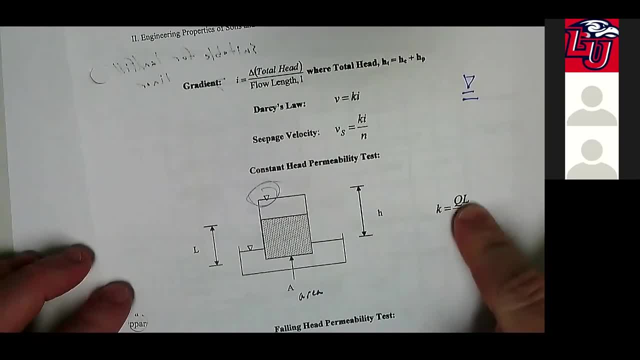 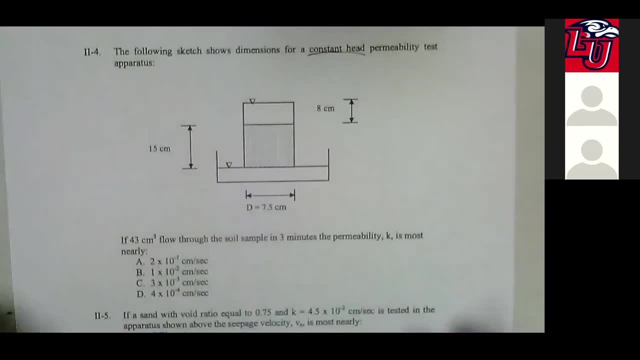 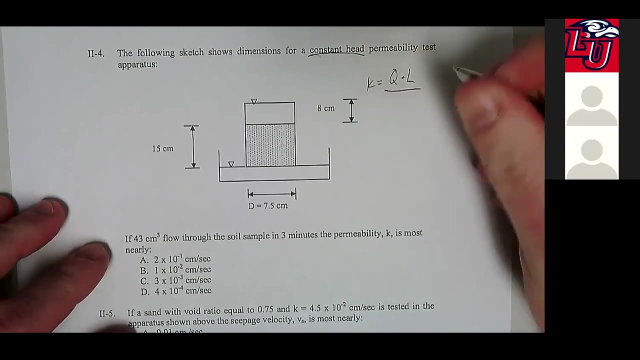 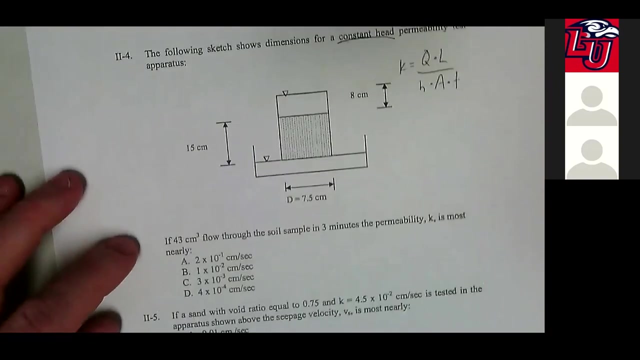 that you're going to need. This is what we need. K is equal to QL divided by HAT. That's our equation for permeability. for a constant head permeability test, Say: K is equal to Q times L divided by H times A times T time. What do we have here? What was given to us? 43 cubic centimeters. 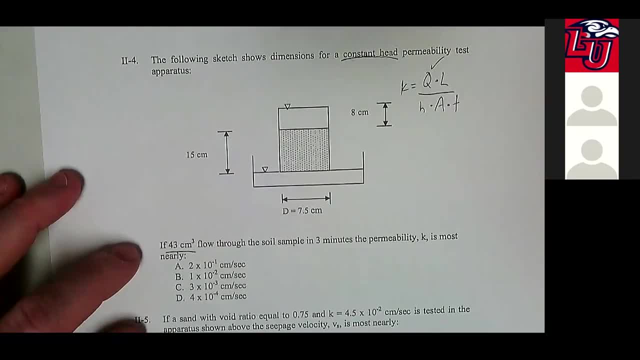 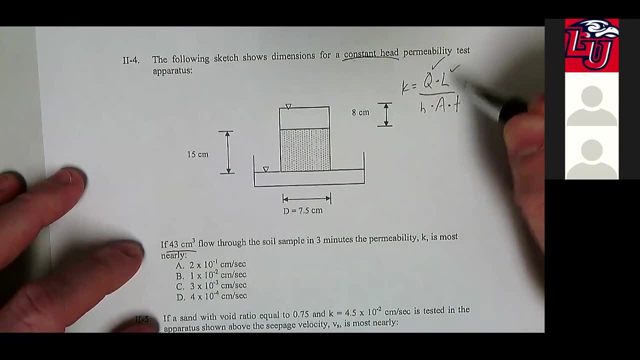 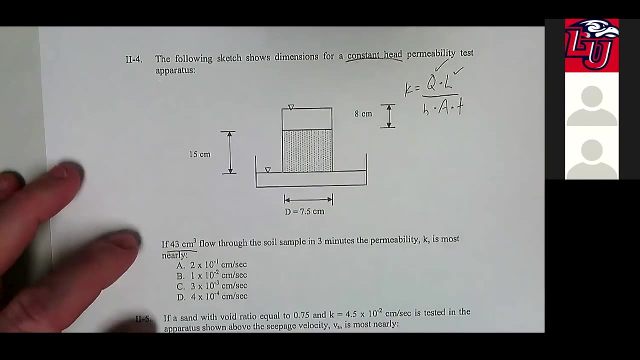 Q, volume of water was given. L is the length of the soil sample: 15 centimeters. that was given. H is actually the head. This is the head differential And remember this is where the problem will trick you up. 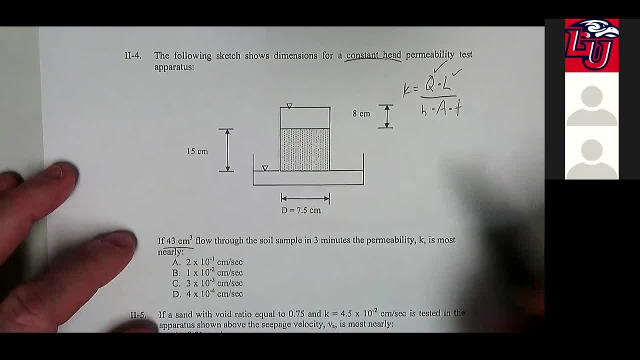 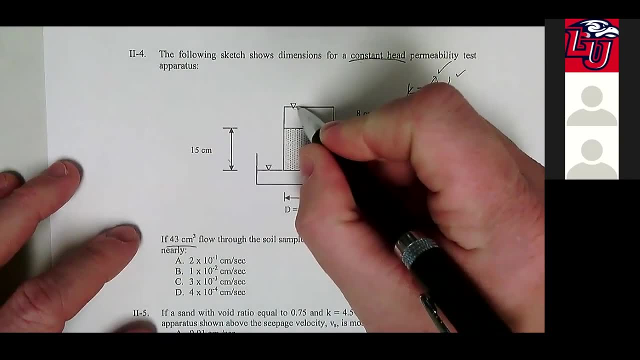 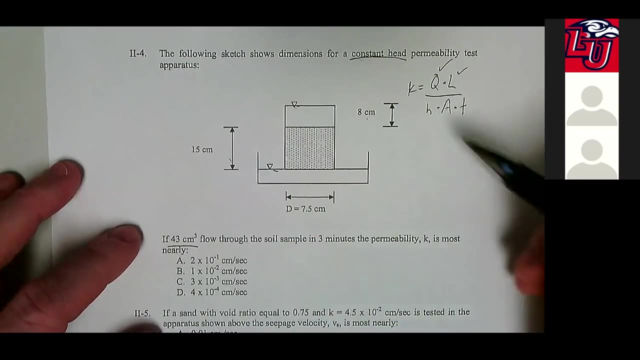 where people say: well, is this H or is that H? Well, neither one. Remember, H is the difference between this little symbol and then that little symbol. It's the height of water that's actually applying head or pressure on the soil sample. So H is actually equal to 8 plus 15, or 23.. That would be H.